Bombay, at Kalyan And then in Ooty between 1964 and 1966, I think- they built the Ooty Radio Telescope And after that the GMRT. the Giant Meter Wave Radio Telescope is probably history. 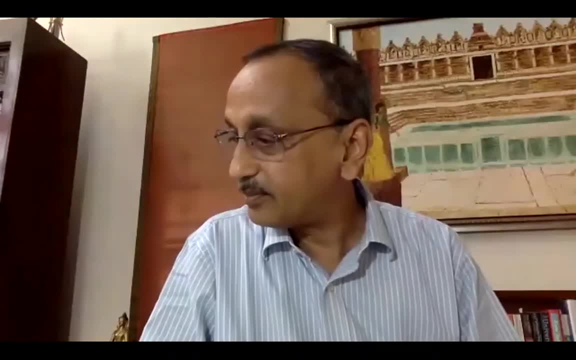 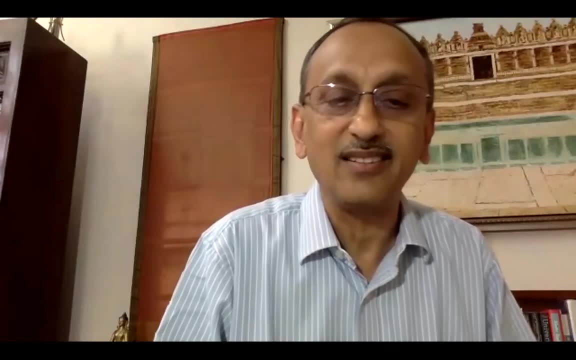 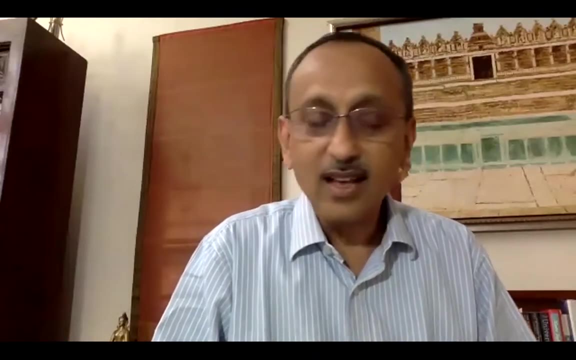 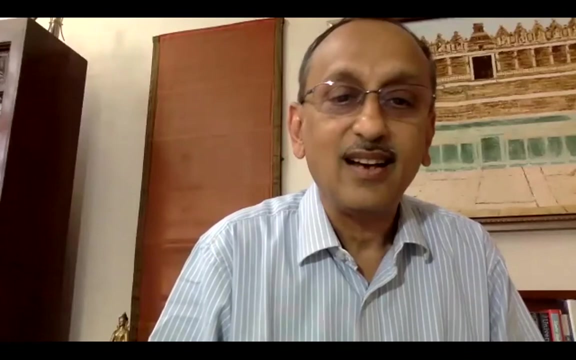 It's a big way for us, which has 30 fully steerable, an array of 30 fully steerable telescopes, 45-meter diameter each, So it's a big, big operation out there. We couldn't have found anyone better to chronicle this inspiring journey. It's a pleasure to introduce. 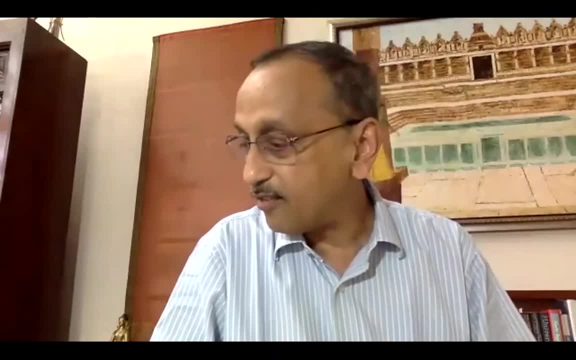 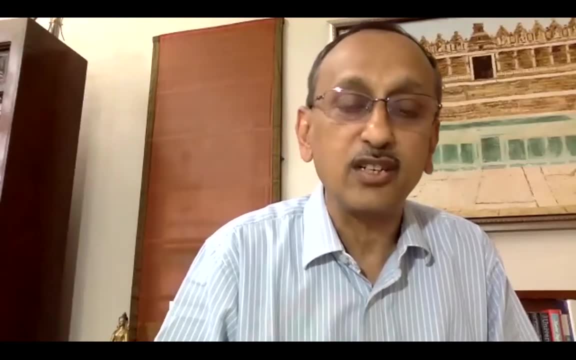 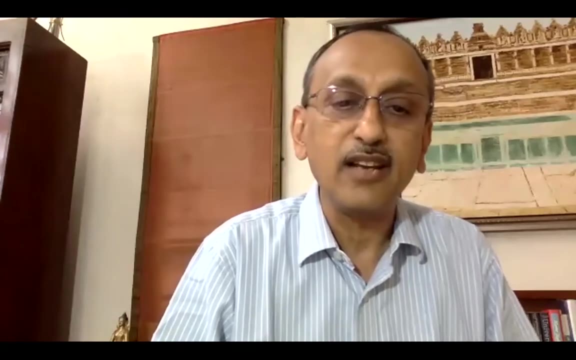 Hari Pulakat, a journalist, a winner of the Nobel Prize in Astronomical Science and a winner of the Indira Gandhi Prize for the popularization of science, And Hari has recently published a book called Space Life Matter, where he walks the reader through several 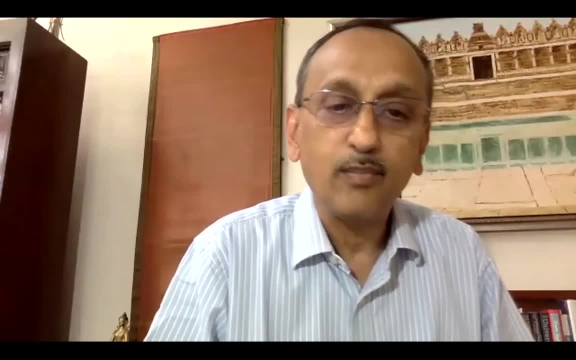 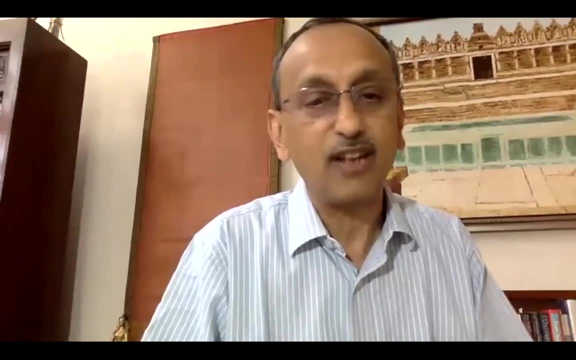 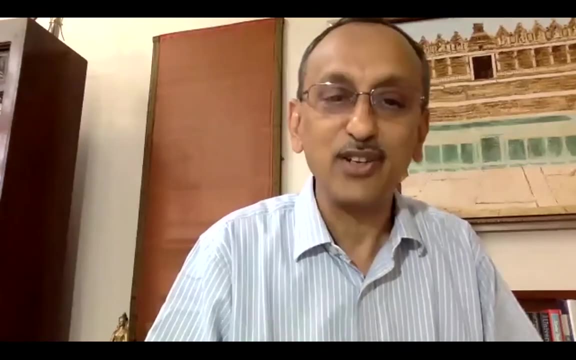 such inspiring journeys- post-independent India in the journey of science. So he's very painstaking. I've read the book. It's a lot of detail. It's an exciting story. I was deeply impressed and I couldn't put it down. I just had to finish it. So it's a 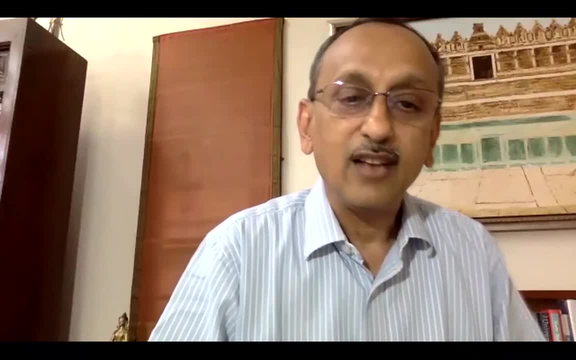 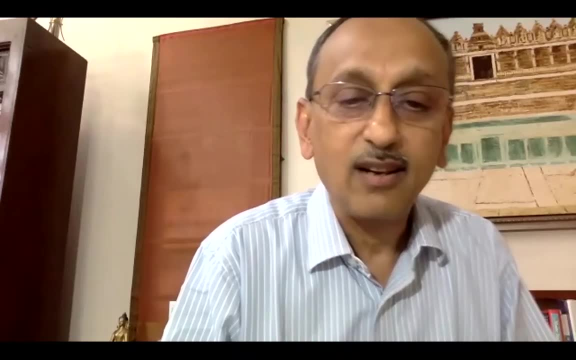 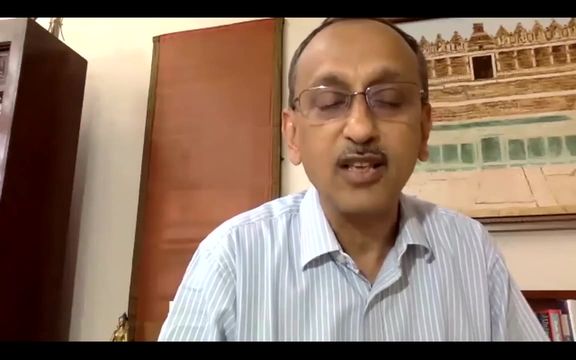 great read, So I will hand over to him. But let me just walk through a couple of a few of our house rules. I'm sure there will be lots of questions, So please put them in the Q&A box. Do not put them in the chat box, because the chat box is not being monitored. 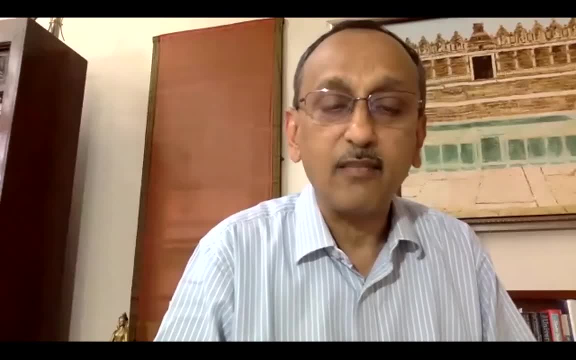 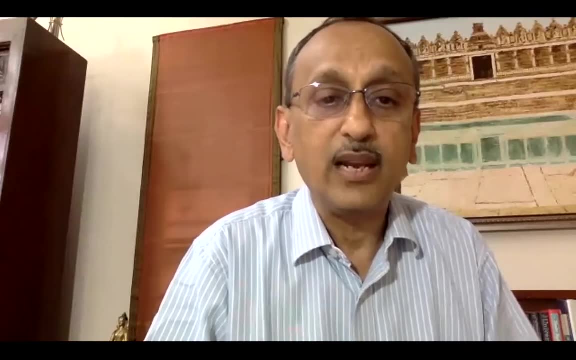 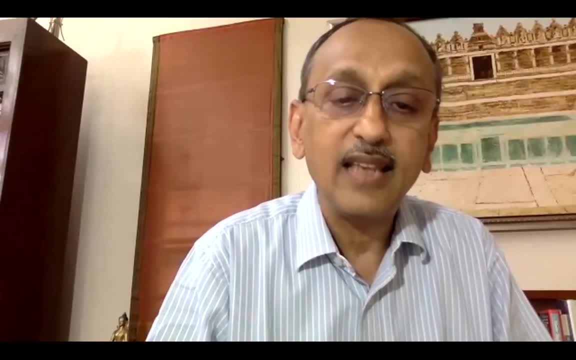 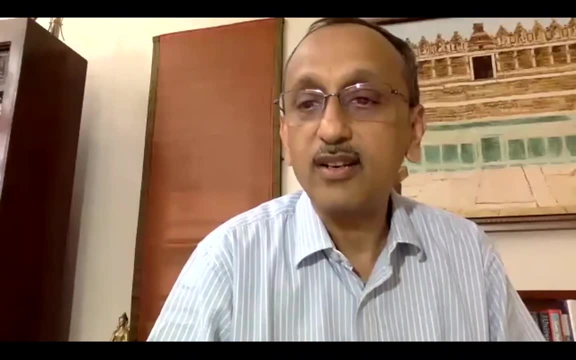 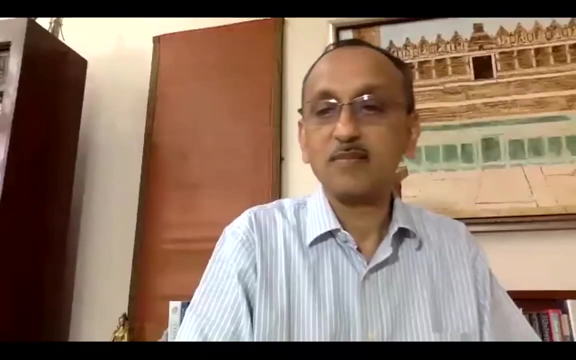 then start taking all the questions and at the end, uh, sushila will summarize the key takeaways from today's webinar. so, without any further delay, hari over to you. so thank you, ashok, and thank you sushila, for the giving this opportunity. um, my book contains a lot of. 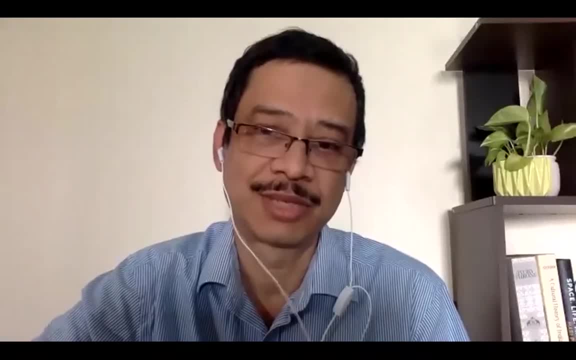 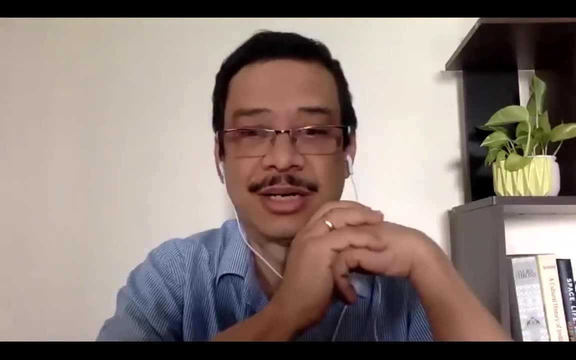 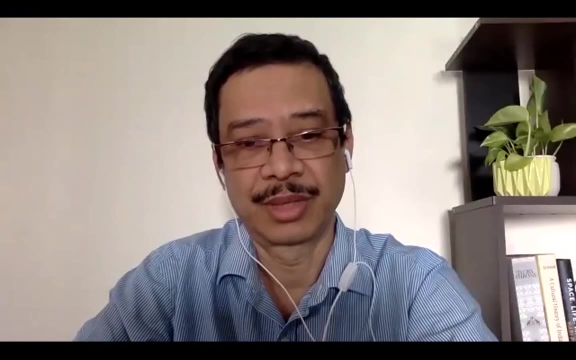 personalities in some some several aspects of science in india and one of the most memorable um experiences for me was to write and learn and write about what govind did in india and i hope i can communicate some of that excitement today. um, i have some slides. i'll start sharing them. 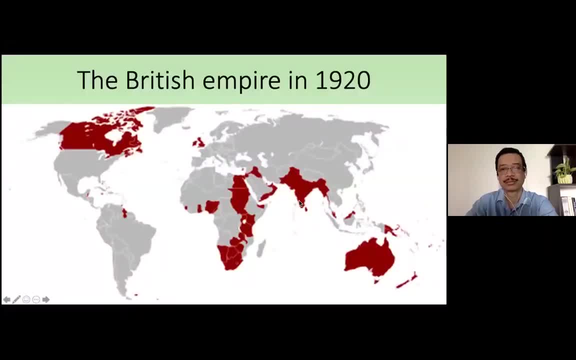 okay, so i start with a map here of the british empire in 1920.. um, there are more than 30 countries current uh. you know. in this map- and if you leave out canada and australia, which are countries made of primarily of european immigrants, india stands sort of unique in one respect because none of the other countries had uh: science. 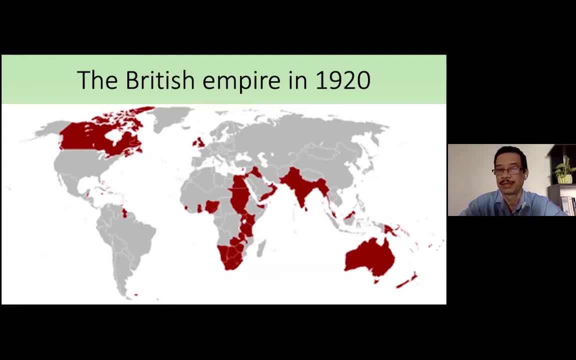 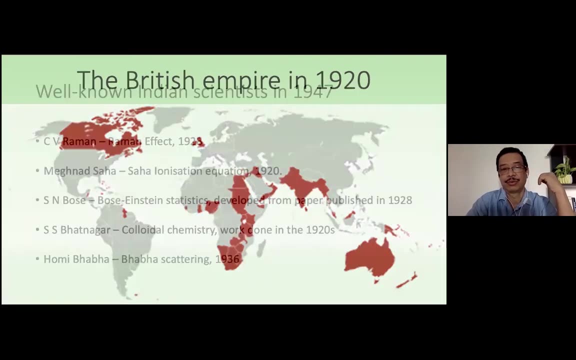 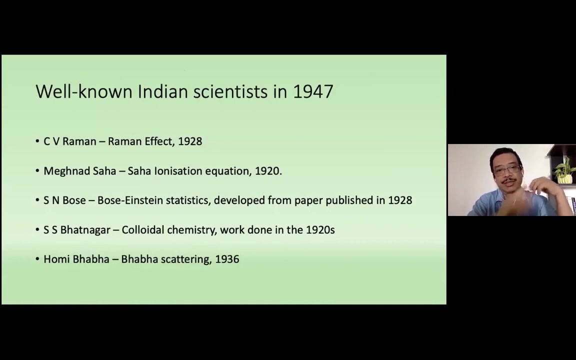 and then to any significant extent at the time of independence, their independence. so in 1947 india was probably the only country which had a significant scientific um program. and if you look at the in 1940s with what we did, so we had cv rahman, already a nobel prize. 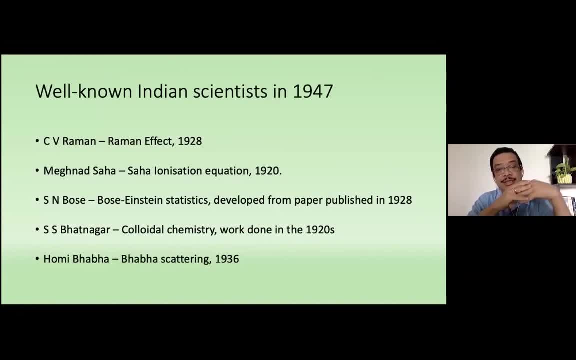 winner in 1930. um, in fact he was the second nobel price winner from from the former british colonies, and the first one was in canada, uh, not in australia. magnan saha had discovered the saha and i session equation, SN Bose developed Bose-Einstein statistics, also work done in the 20s. 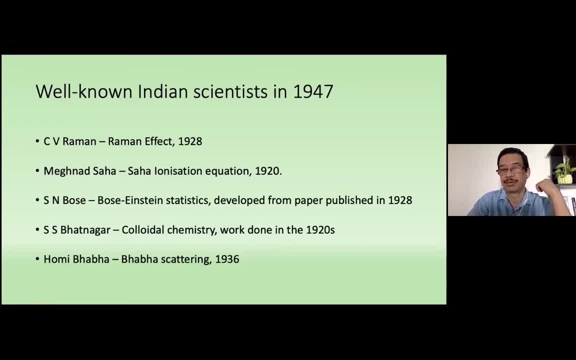 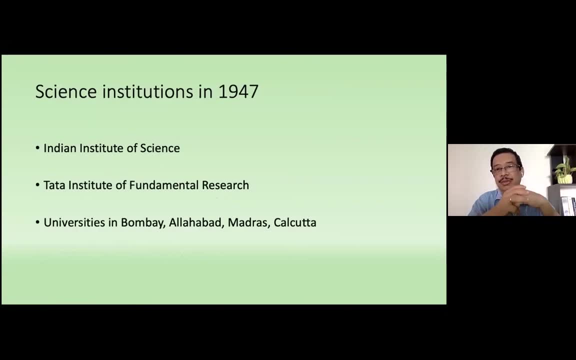 So something had been happening in India already when independence, when India called independence. So these were the institutions, primary institutions in India. in 1947, the Indian Institute of Science started. early in the 20th century, Tata Institute of Fundamental Research started. 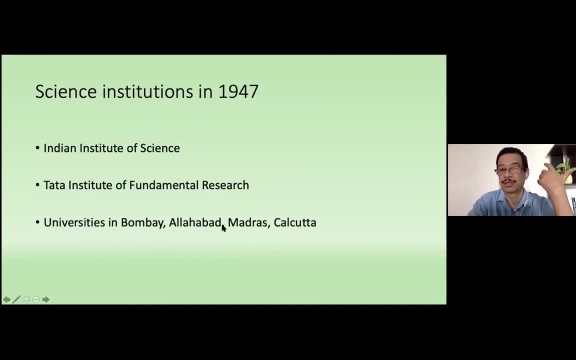 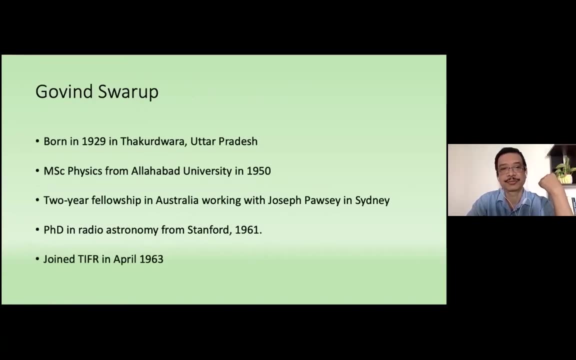 in the 1940s, Universities in Bombay, Allahabad, Madras and Calcutta were old, much older than that, And you had Banaradu Sindhu University also and a few others. So Govind Swaroop was born in 1929 in Thakur Dwara in Uttar Pradesh, at the foothills of 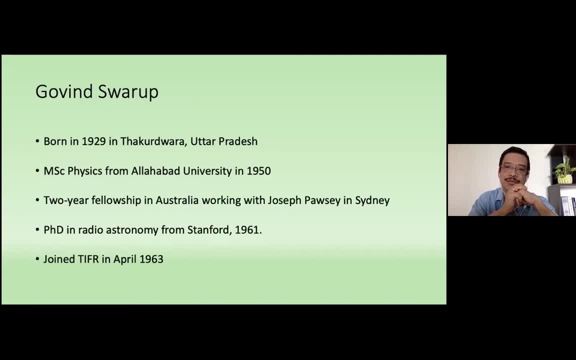 the Himalayas, I think about 50 to 60 kilometers from Moradabad. So he did his MSc in physics from Allahabad University, Then went to Australia for two years on a fellowship and worked with Joseph Posse radio astronomer. 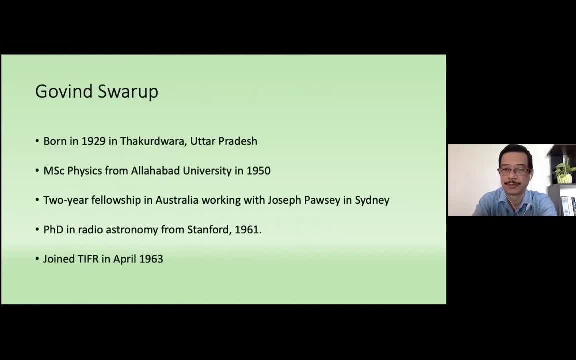 Then he came back. he built some about 30 antennas in Australia during these two years And Australia donated those antennas to him To bring them. So unfortunately Indian government wanted them to bear the cost of shipping also, which Australia was not willing to do at that time. 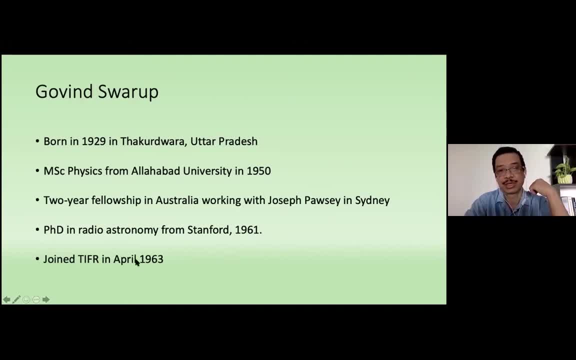 So Swaroop waited for some time and then he left for the US and he worked in Harvard for some time, went to Stanford, did a PhD And then came back to join KFRU. So that was it. He left KFRU in April 1963.. 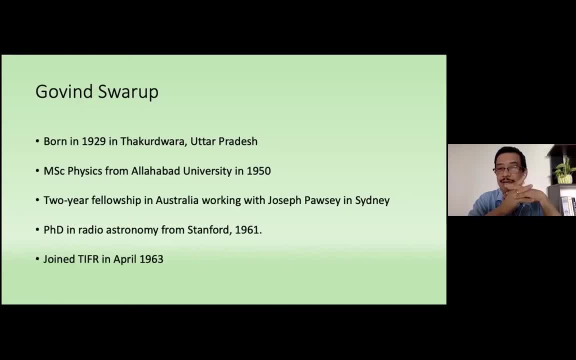 In fact the KFRU wanted him to join on April 1st and he refused to join on April 1st, on April Fool's Day. So this was the situation on radio astronomy at that time. Karl Jansky built the first radio telescope in 1931.. 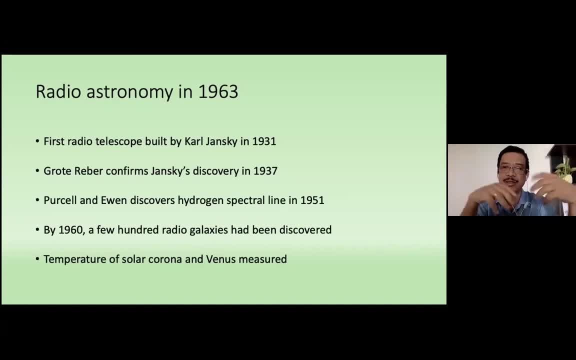 It was not quite a radio telescope. he just put some antenna on a platform with some tires- car tires- And then he got signals from the center of the galaxy, which was big news in 1931.. But unfortunately Jansky could not continue this work because he was working in Bell Labs. 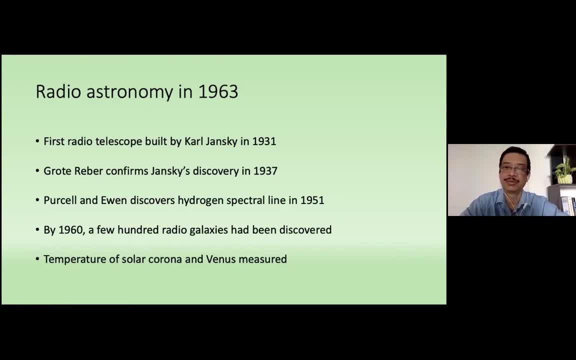 Nobody in Bell Labs was interested in funding this program, because they were interested in transatlantic communication, And Jansky's job was to figure out what would interfere with that communication. So then, Gro Treber, I don't know. I don't know. 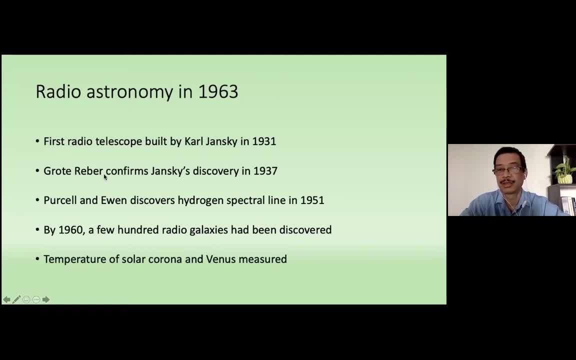 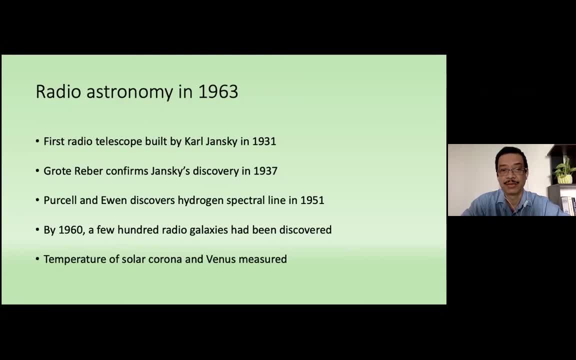 Jansky's discovery And then the H discovere s the hydrogen s um and contain a lot of information and and became a big troll in astronomy later. so in by 1960 when Swaroop was in GIFR. several hundred radio galaxies have been discovered. 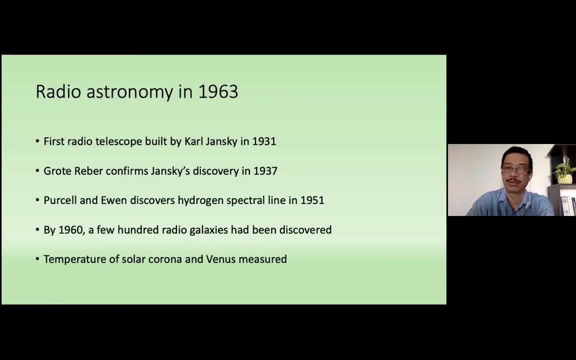 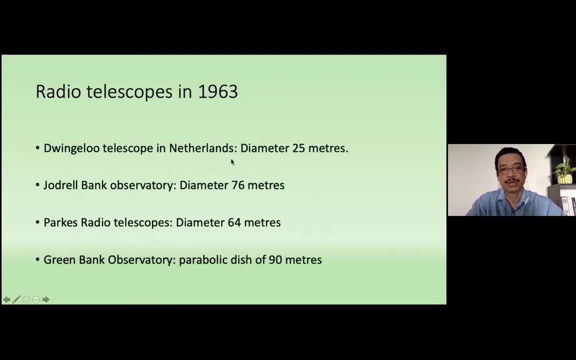 and temperature of solar corona and venus measure and and quite a few other things. so radio astronomy was a very well developed field already when he came back. so this was the telescopes around the world at that time, the major ones: radio telescopes, the dwingelo telescope. 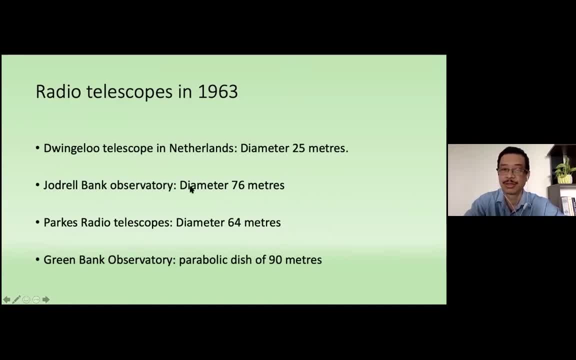 was 25 meters in diameter. the total bank observatory was 76 meters in diameter, the parks radio telescope 64 meters. green bank observatory, which was a parabolic dish for 90 meters in one, one direction, in one diameter. so there is an interesting film about the park. 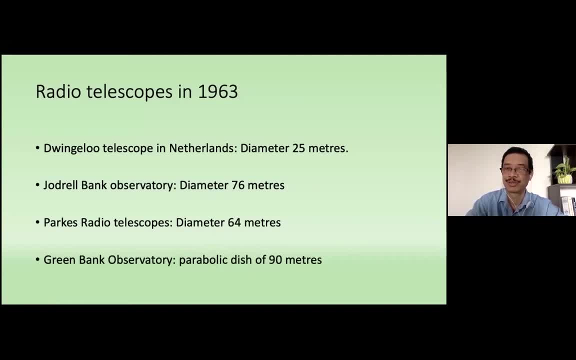 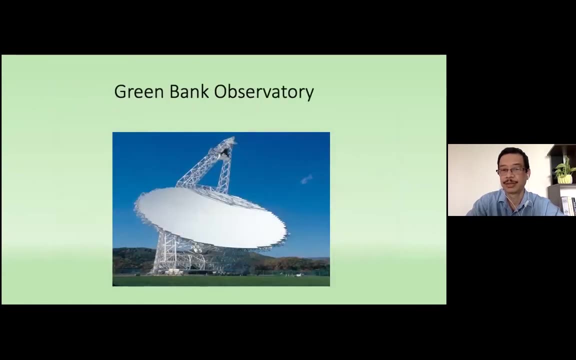 stereo telescope called the dish, made in 2002- it's a comedy- which was used as an appling antenna for the apollo program. so this is how the general bank telescope look and this is how the green bank observatory looks now. so these are all very sophisticated telescopes. 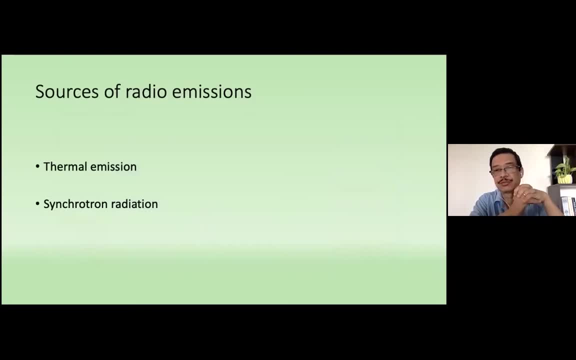 so? so there are two sources of radio emissions. one is a thermal emission, which comes from temperature of a body, and all bodies emit radio waves at all temperatures. so this is an important thing for radio astronomers, because you can look at objects at any temperature and get information. 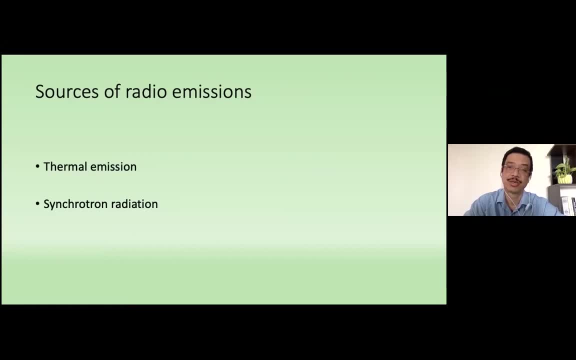 but they don't emit light at all temperatures, only when they're heated to a few thousand degrees centigrade. and then the synchrotron radiation which jansky found is. it happens when electrons spirited around magnetic field. now electrons are plenty in the universe and 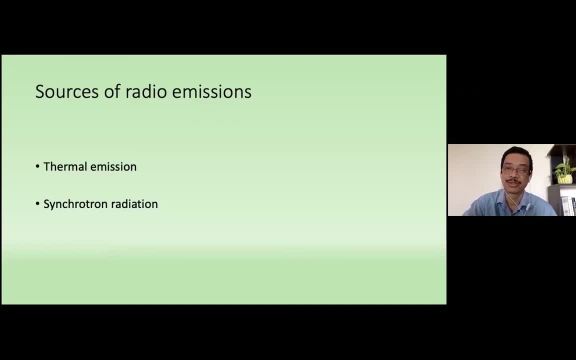 so are magnetic fields. so once again, this is a great source of information for radio astronomers. so the biggest problem at that time in the 60s was to find evidence for big bang. so the biggest problem at that time in the 60s was to find evidence for big bang. 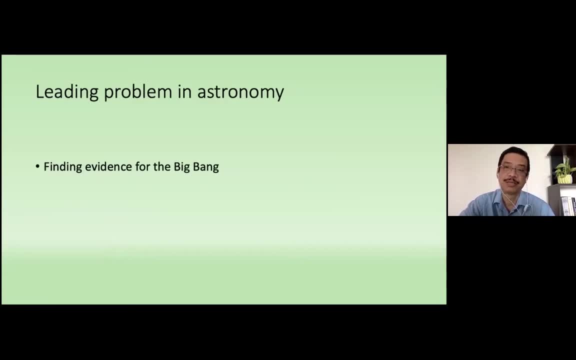 people thought that this was the. this was correct. the competing theory was the steady state theory propounded by fred hoyle and. but there was no convincing evidence that the big bang was correct and everybody was looking for evidence from it for the big bang, and swaroop also wanted. 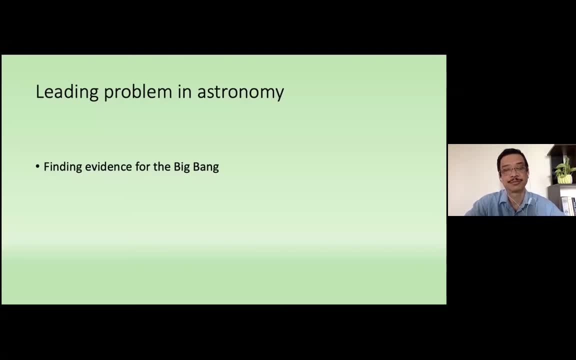 to find evidence. in fact he was preoccupied with the problem. so the state of tifr in the 1960s. in 1963, scientists had just moved into a new building by the sea next to the naval headquarters, the naval quarters. sorry, it's been a year and the intellectual climate there was incredibly incredible. it had central. 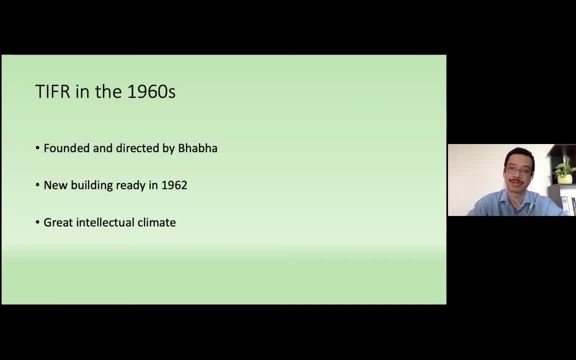 air conditioning, which was unimaginable in an indian scientific institution at that time, or probably any institution that baba wanted scientists to work in comfort and the the campus was fantastic. by the sea people could go for walks. uh, after lunch, gardens with a lot of interesting plants and animals coming birds, so 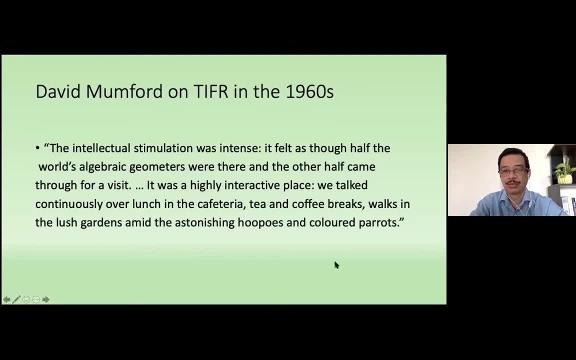 this is what mumford described. i i've got this in the book. the intellectual stimulation was intense. but david mumford was a mathematician, shan't recover it by hand. it's a study, not quite a failed student. anything clinical scorching effect An experiments will live today on naturalyou unique species and as such radiation continuation is excessive. the risk is minimal. 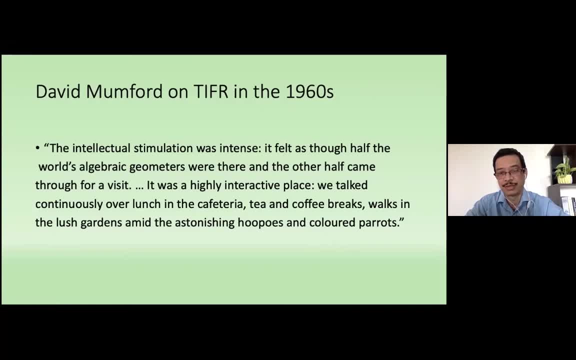 mathematician who worked in TIFR in the 1960s, who was a field medallist. The intellectual stimulation was intense. It felt as though half the world's algebraic geometers were there and the other half came through for a visit. It was a highly 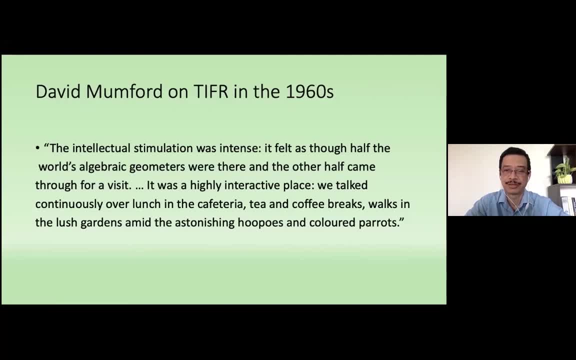 interactive place. We talked continuously over lunch in the cafeteria, tea and coffee breaks, walks in the lush gardens and amid the astonishing hoopoes and colored petals. So even Mumford, who came from an incredible place, found TIFR to be an incredible place, But there were problems. 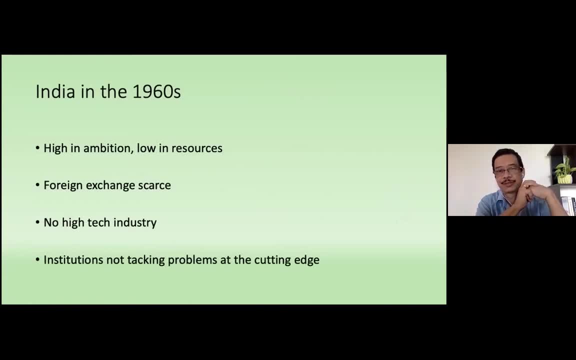 So this is how India was in the 1960s: High ambition, but low in resources For science. this was a big problem. Most of the scientists who had made a mark in the 20s- 30s were theorists. But Nagar was not a theorist. Siva Raman was. not a theorist, But science had been moving on since then and it was began to be equipment driven after the World War. So India did not have the infrastructure to do experimental science at the cutting edge. Foreign exchange was very scarce. What this meant was: you cannot. 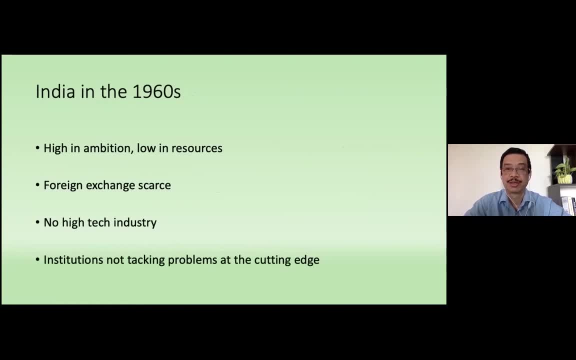 travel, you cannot import equipment, You cannot subscribe to too many journalists, You cannot subscribe, they can't, journalists cannot come by air and they came by sea So they came very, very late. So you're essentially out of touch and had no equipment. 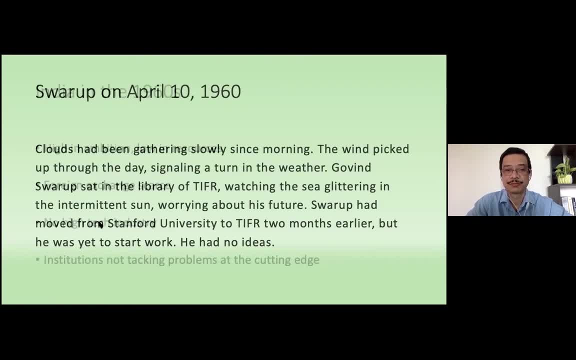 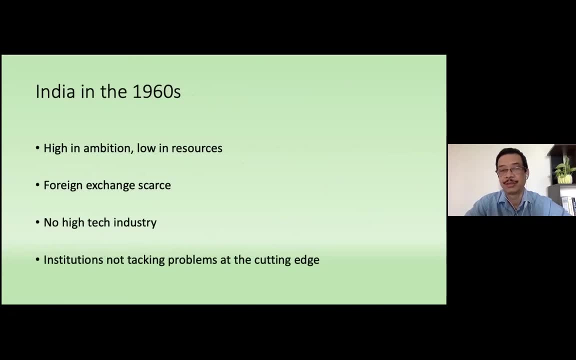 This was this, and no high-tech industry. That is because you need a private industry to make equipment And if you want to make them in India, if you can't, you can't import them any bit. But if you want to make them in India, you have to get. 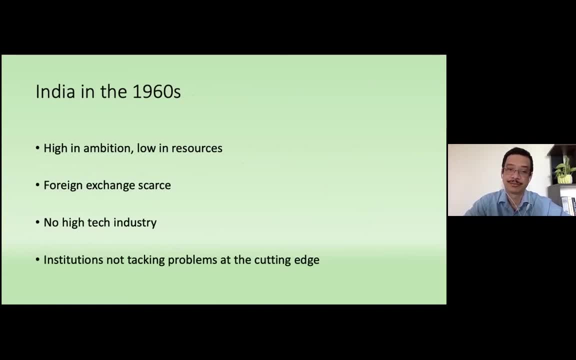 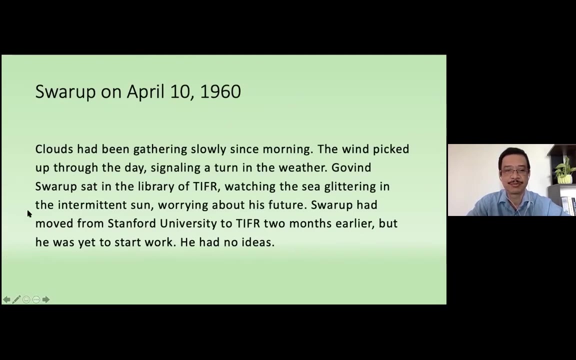 components And there were no companies who made the components. So, because of all this, most institutions did not work at the cutting edge. So this was the situation that Swaroop found himself in, And this is the opening paragraph of my book. I've just read it: Clouds. 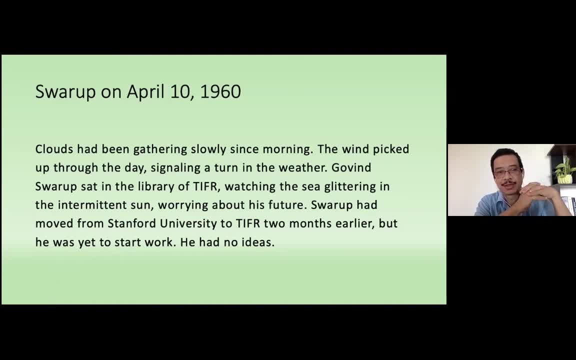 had been. it was April 10th 1960.. Clouds had been gathering slowly since morning. The wind picked up through the day, signaling a turn in the weather. Govind Swaroop sat in the library of TIFR watching the sea glittering in the intermittent. 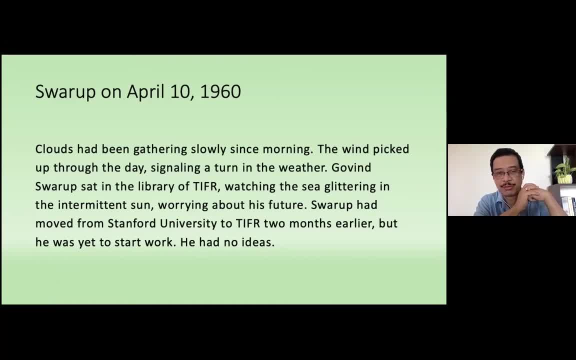 sun worrying about his future. Swaroop had moved from Stanford University to TIFR two months earlier, but he was yet to start work. He had no ideas, And he had been thinking about this for two months, but he didn't know what to do Because he had some. 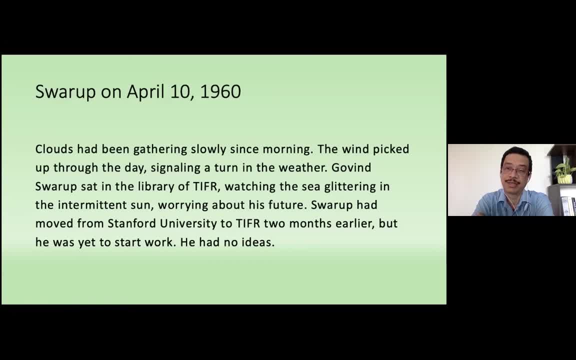 antennas- The antennas that Australia gave- they finally made their way to Delhi, And from Delhi they came to TIFR. But that was not good enough for him to look for evidence for the Big Bang, And this is a problem that Swaroop was preoccupied with at that. 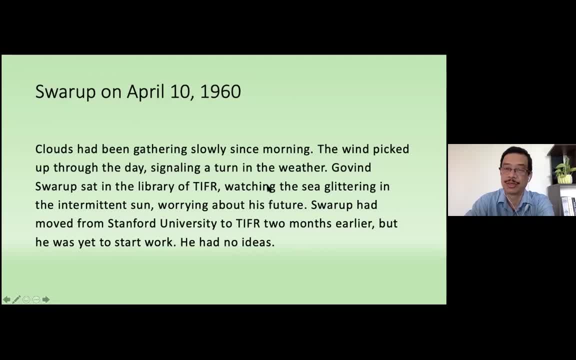 time And he really didn't know what to do, And he describes this period that takes two months as one of his lowest points, because he had come back, He had given up a job at Stanford and he didn't know what to do, So he had actually gone to the library. This was in the library. 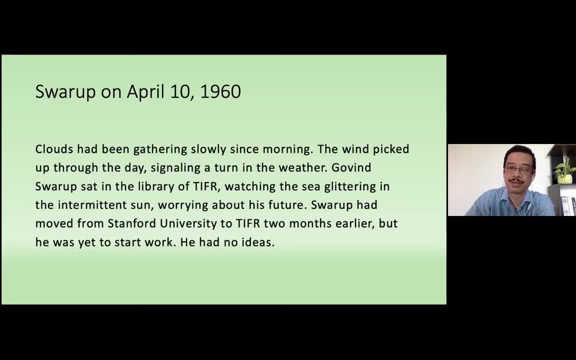 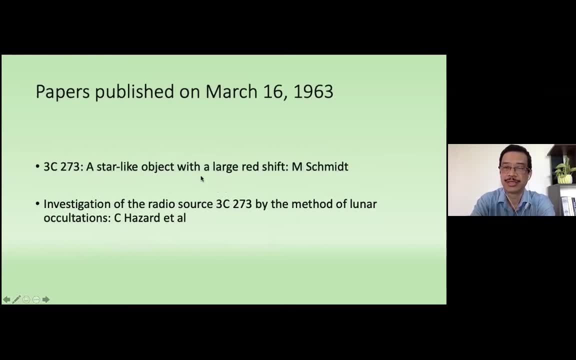 to read some papers, but he did not read for a while, He kept brooding And then finally he read two papers. So Nature had on March 16th had published four papers on radio astronomy. Swaroop found them on April 10th. There were two papers here. 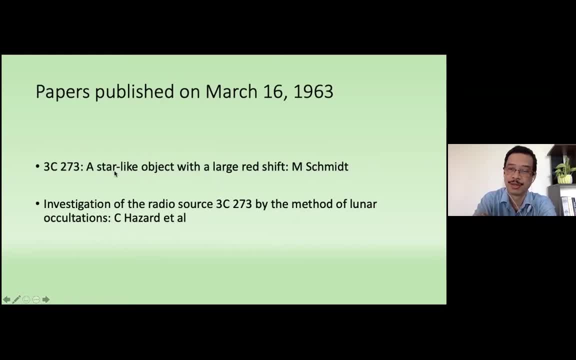 This was by Martin Schmidt. the first one announced the discovery of quasars, large objects with a black hole at the center. Some of them were shown. some of them were shown with the brightness of an entire galaxy, more than the hundred billion stars in the 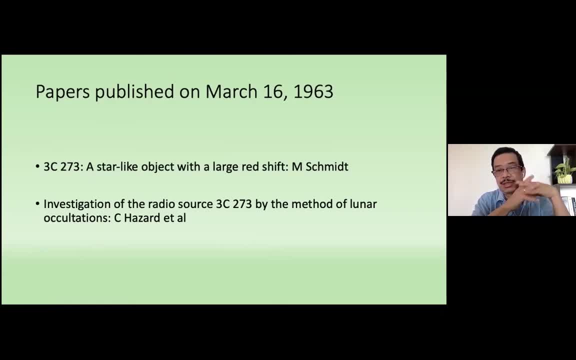 Milky Way, for example. And one other paper which Swaroop saw and got interested in was a paper which investigated this quasar using lunar occultation, you know, using the moon edges to improve the resolution of a telescope. So when he read that he immediately realized what he could do. 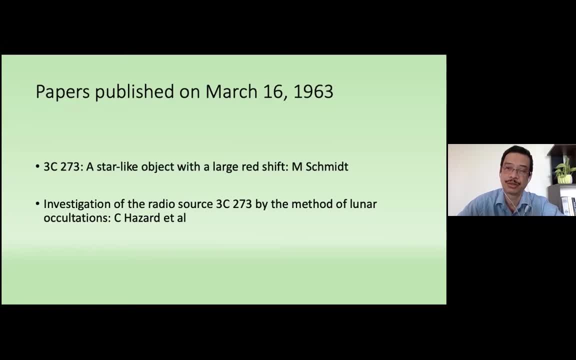 So he could build a telescope that used lunar occultation to improve the resolution so that he could look far into the distance, into the early time, early period when the universe was formed. So he thought that if you looked far enough you would find how. 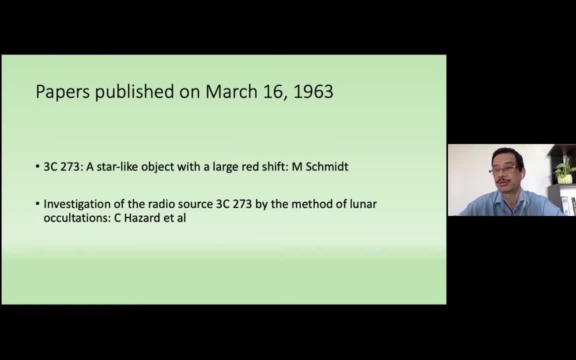 the universe looked like in the early universe soon after its formation And that would give clues to you know whether the Big Bang really happened or not. The galaxies were close to each other. That means the universe was different 10 billion years ago, which. 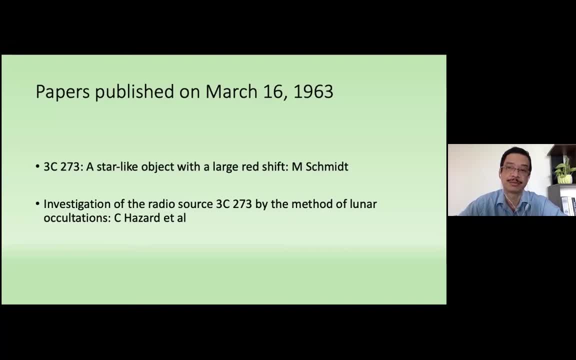 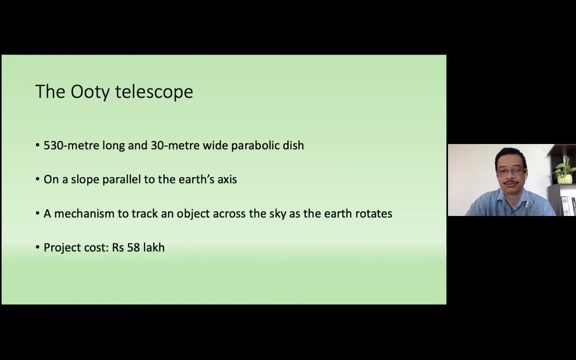 was what people thought at that time when the Big Bang happened. We now we know it's more than 10 billion years, it's about 13.7.. So then Swaroop sat there and conceived of a telescope. We have seen earlier that the biggest telescope at that time was 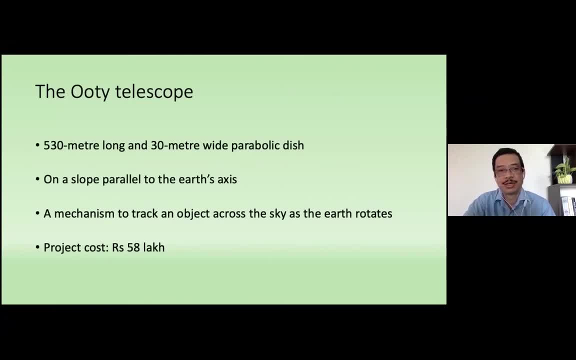 the Greenback Observatory, So 90 meters. He thought he would build a telescope just 530 meters long and 30 meters wide, More than half a kilometer long, and he would put it on a slope That is parallel to the Earth's axis. 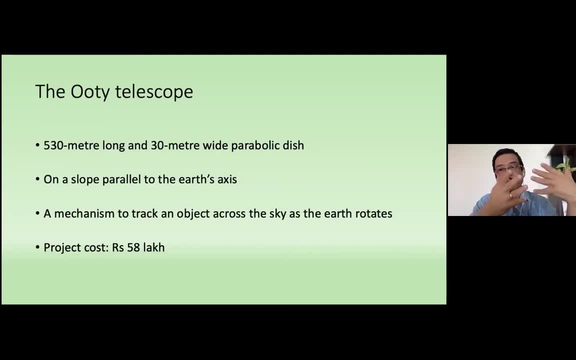 And then he would steer the telescope across the sky to track an object as it rose from the east and went across to the west. He went to Baba and asked him, told him about his idea and said he will write a proposal. Then Baba said: you know, don't waste your time, form a team and 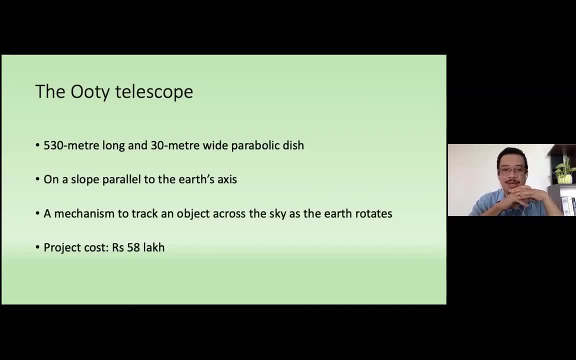 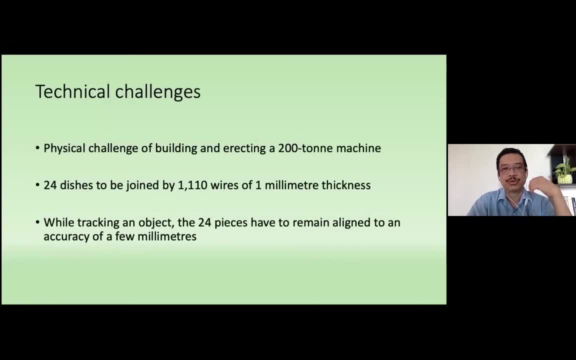 then we will see. And if you have, once you form a team, you will fund, And the budget was around 58 lakhs. So this was a challenge. If you build a telescope which is more than half a kilometer, it. 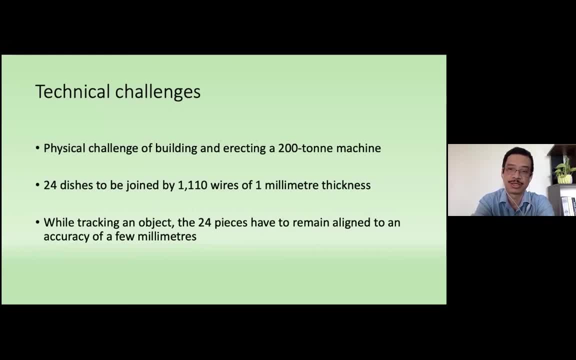 would weigh at least 200 tons, and it turned out to be more than 200 tons. later there were 20, to be 24 dishes, each one of them separate, and they have to be steered separately, joined by 1110 wires. 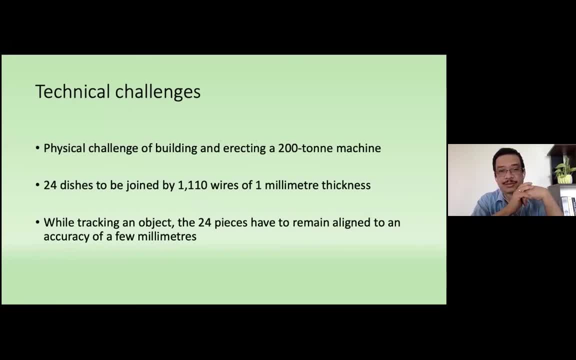 of one millimeter thickness and these pieces have to be steered to precision of a few accuracy, of a few millimeters. nobody has seen, has that kind of accuracy in India and in fact the company which took up the project said: we have, we used to, we are used to in accuracies. 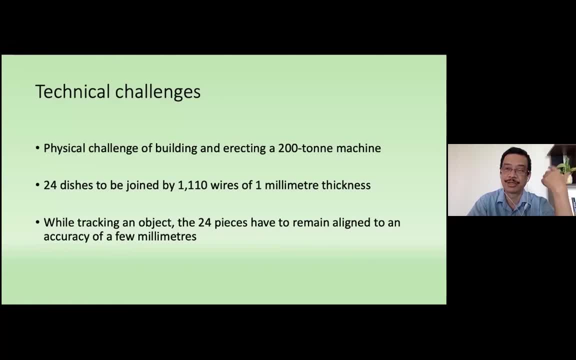 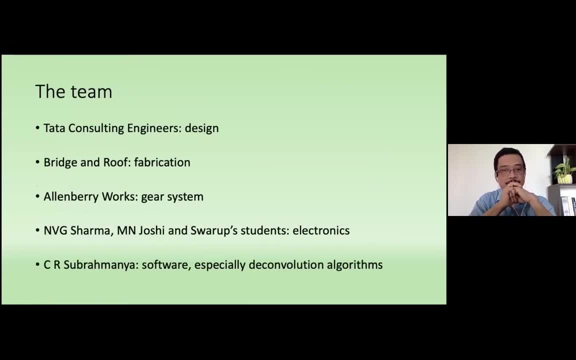 in feet, you know in tens of millimeters and not in millimeters. so he formed a team. Tata consulting engineers got the design. they were not very keen to do this design initially because they were scared. they had not done anything before this like this before. so then, 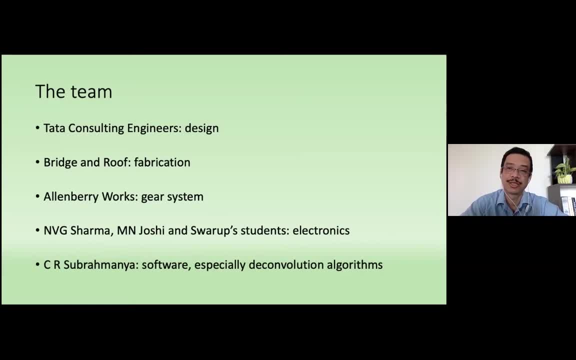 Baba had to convince them that if Baba will take the responsibility of failures, if they put their best people on the job- bridge and roof in Calcutta with the fabrication, Allenbury works, also from Calcutta with the gear system, and there were only two experienced 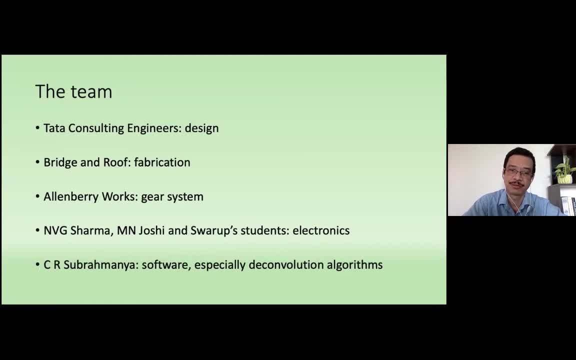 scientists, experienced astronomers, MBG Sharma and MN Joshi from National Physical Laboratory in Delhi. they joined his team and the rest, all the rest, was students. the students built the electronics. software was built by one of his students, CR Sabramania, and he developed the big convolution as our algorithms, which is: you know they, when you, you know the recasting. 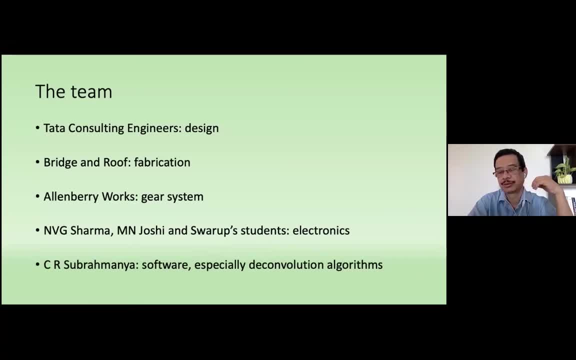 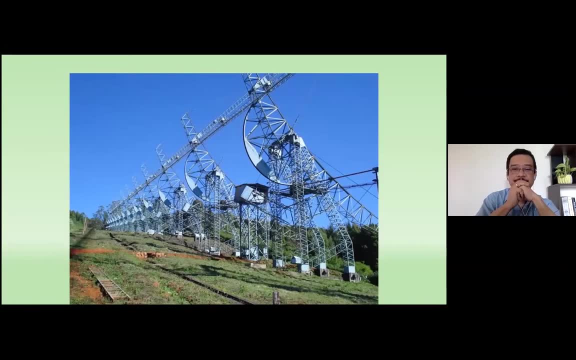 to the image. objects from the image. so is how it looks like in 1970. the telescope came up. soon after, on the day India invaded Bangladesh, the telescope collapsed. part of the telescope collapsed and it took another year for them to get it up and running and they lost one year, but it finally it started operating. 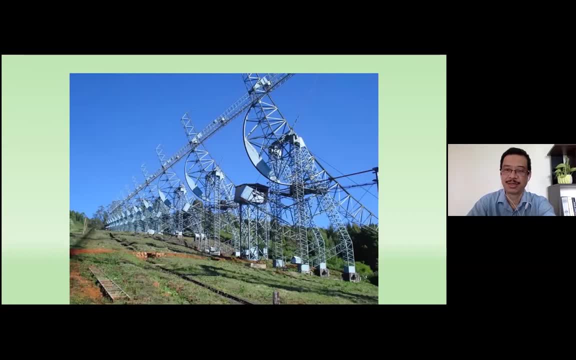 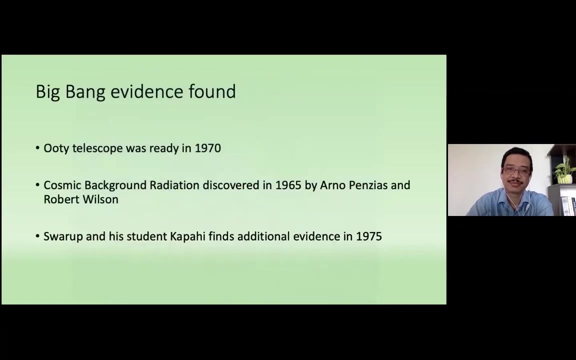 and it has been operating ever since. a picture like this does not give how give any idea of how the telescope really looks like. if you go there you realize how big it is. you know it's a size is really extraordinary. so his aim was to find evidence for the big bang. 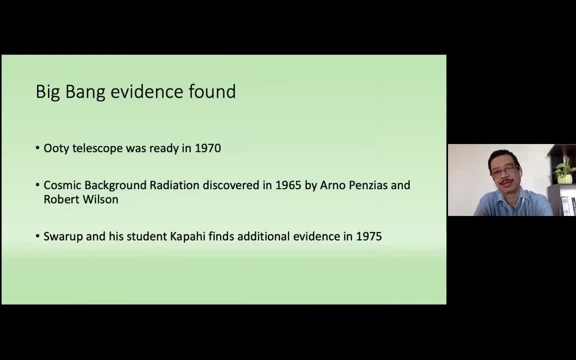 the telescope was ready in 1970 but evidence for the big bang was found in 65 when Arno Penzias and Robert Wilson from Bell Laboratories found cosmic background radiation. but Swaroop and and a student first, student Kapahi, who became later became the director of NCRA. 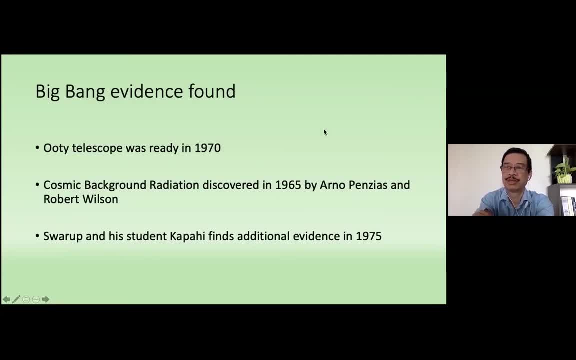 found additional evidence because they found that the galaxies were very close together and soon after the universe was formed and that paper was published in 1976 and since then the UT telescope have been used for a lot of work and to study pulsars used to study. 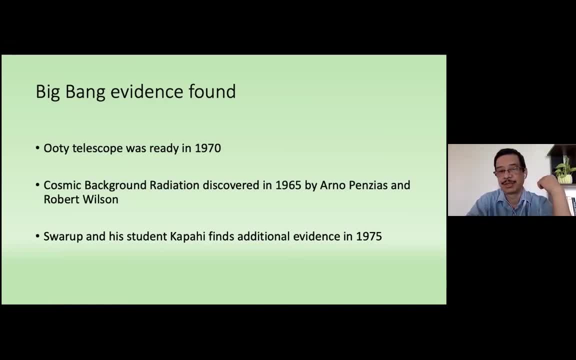 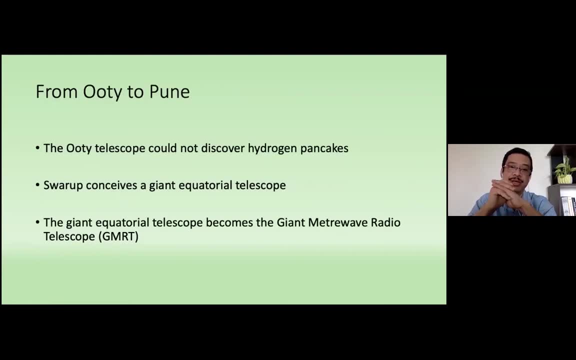 space weather especially. but then Swaroop had another big problem in his mind at that time, so to find hydrogen pancakes. so people thought that galaxies were formed in the universe after the universe was formed. so people thought that galaxies were formed in the universe after the universe was formed. 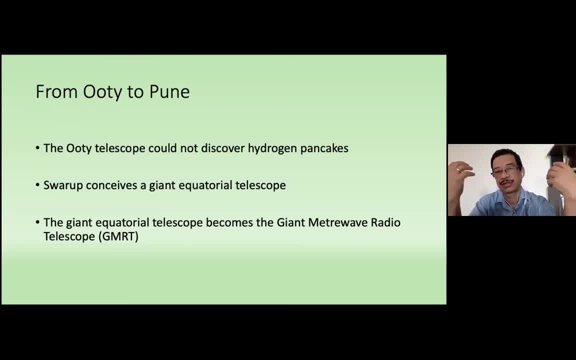 was formed from top down. there were huge bank hydrogen clouds which broke to form galaxies, which broke the farm which we're talking from clusters of galactic clusters and then broke the form galaxies from them, from the smells and like. so he could not find them with a woolly telescope. 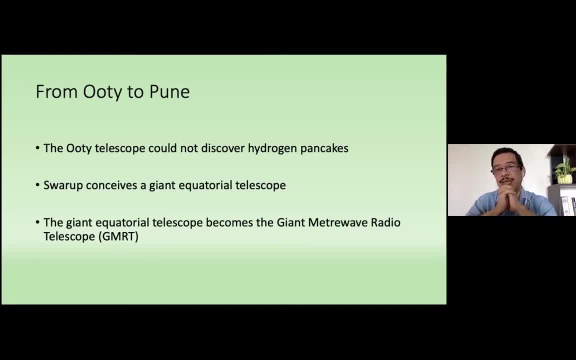 so immediate and he thought that if he built a big enough telescope, a much bigger one, he could find them. so he conceives an equator, giant equatorial telescope to be located somewhere in the equator with a series of dishes that could that be big enough to find hydrogen pancakes? and he spent 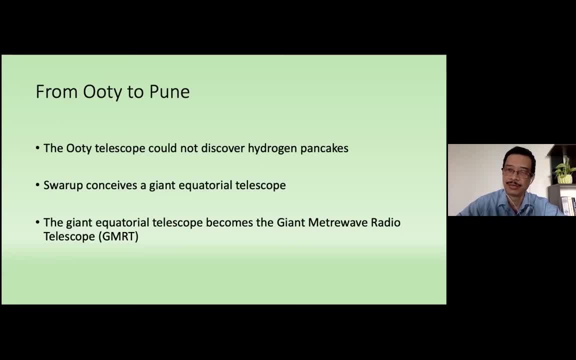 several years trying to find a location. he went to kenya, he went to indonesia and when he went to kenya he was supposed to meet kenyatta, the president of kenya, but the day after he arrived kenyatta died and he had to come back, and then this idea died. but 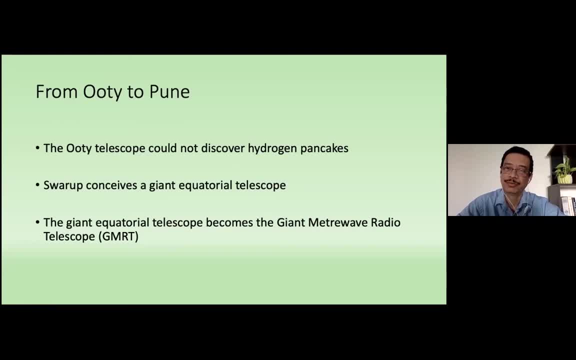 and sort of kept thinking about the problem for several years and finally, you know, on one night they, when new year's eve, um late in the night at about 1 pm, he got the idea that he would build some, uh, a telescope like jia market which consists of 30 dishes about 45 meter in diameter. 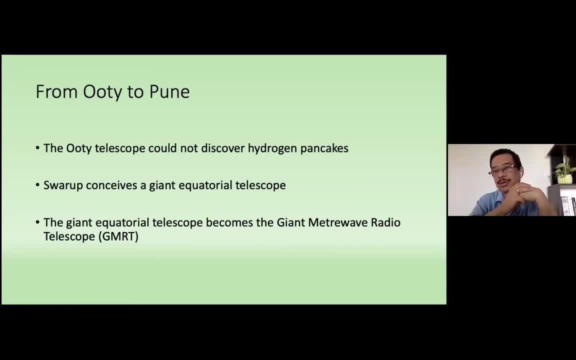 and together they would. they would be able to look far into the universe and have a good resolution. so he went to korea to build a telescope and it was an amazing thing for him. so he moved to pune to build the telescope. pune was picked as a location, i mean. 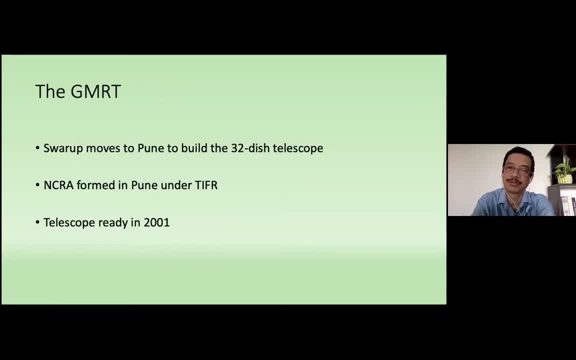 a village near about 60 kilometers from pune called kodak khodad, on the nashik highway. pune nashik highway was chosen as the spot after a long survey. they took about a year. they went all around to move away from the equator. so 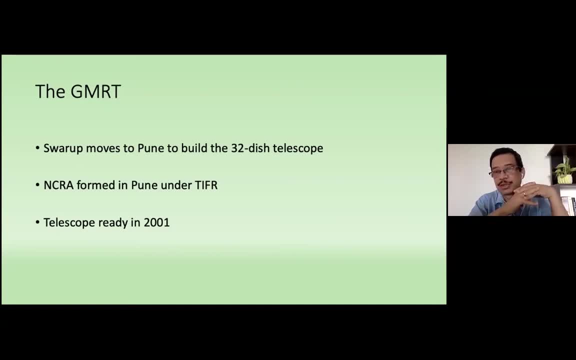 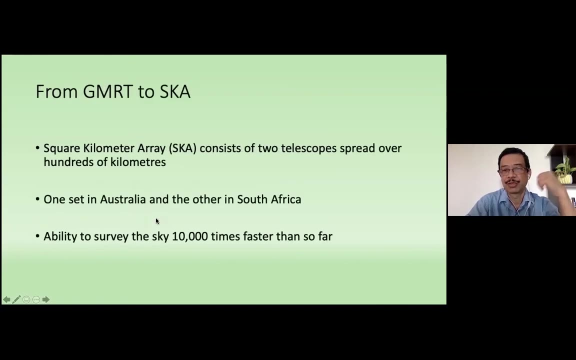 and then in the organa, ncra was formed under ti for it, because if this was near pune, it was decided to form. what is? the telescope was ready in 2001 and now gmrt is. it's a low frequency telescope and right from the beginning, about 30 countries use a telescope. 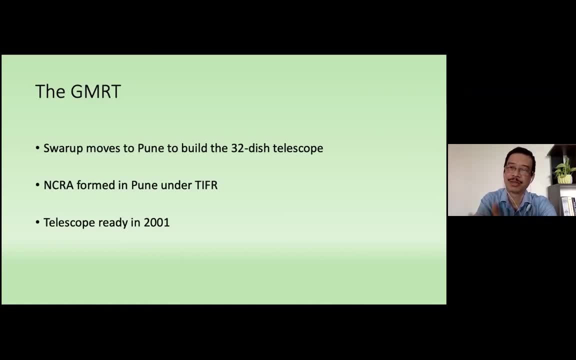 and nobody could get a project automatically, even go and syrup could not get. it is still the world's most powerful low frequency telescope. so from gmrt, as even as the gmrt was being built, surub thought about an even bigger telescope. you know hundreds of dishes spread, you know, at one, two places on the earth. 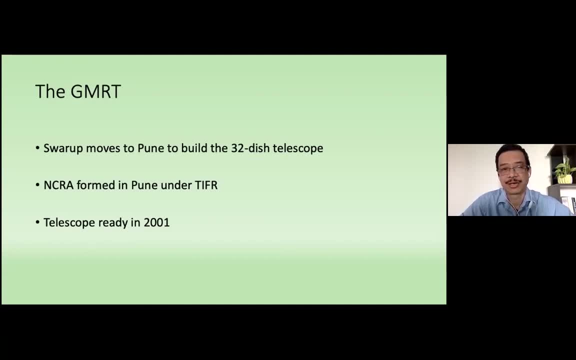 far away from each other so that you can get a long baseline. so that became the idea bec. there were others also who thought in those terms. it became the square kilometer array, which is now a project with about nine, nine to ten countries. india is one of the members who's involved right from the beginning in the negotiations there were. 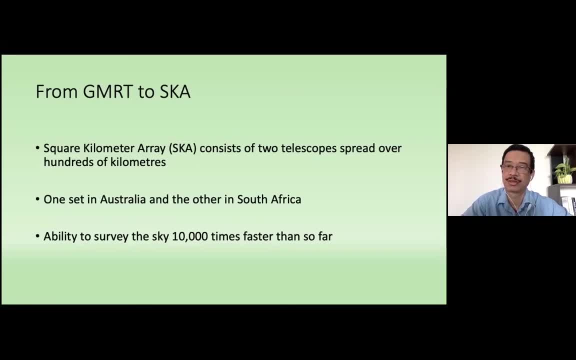 one set of dishes that are in australia, the other set of dishes in south africa. It's one of the biggest scientific projects the world has done. It has the ability to survey the sky 10,000 times faster than any other telescope so far, And India would never have joined this project except for GMRT and the experience gained. 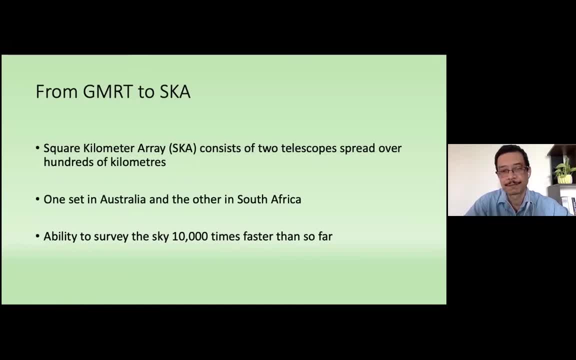 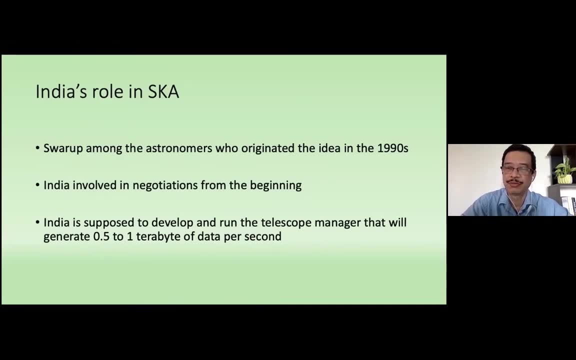 from GMRT. The amount of data that the SKA would generate is close to the total internet traffic in the entire globe. up to one terabyte of data per second it will generate. This is the biggest challenge for the telescope: to analyze this data. 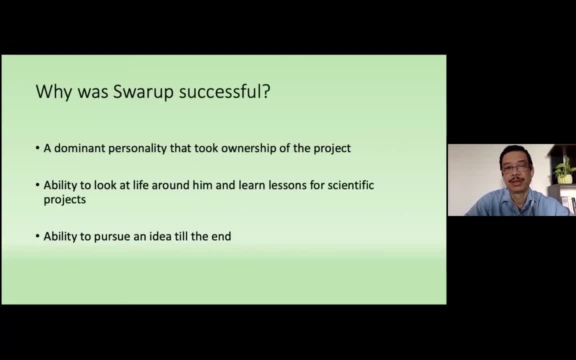 So, looking back, Swaroop did not create just two telescopes, He formed an entire team, he formed a field in the country. Before he moved to India there was no radio astronomy in India, Nobody had built a telescope, Nobody had seen a telescope. 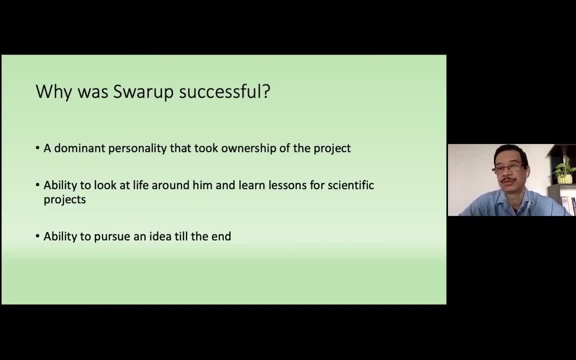 So now India is one of the leading nations in radio astronomy, with two big telescopes and a large team of astronomers. Why did he? why was he successful? and if you look back, there are not that many scientists who created an entire field in the country. 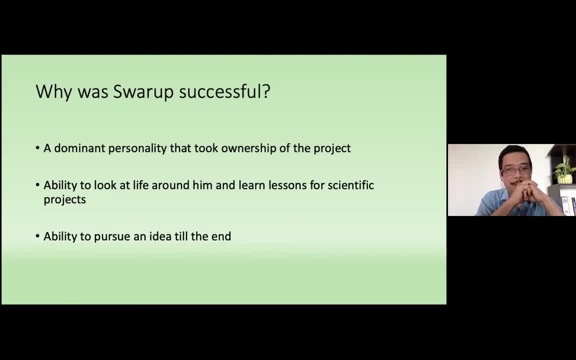 So he was a very dominant personality who took ownership of the project. Now, this has a flip side as well. There are people who say that he micromanaged, but in those days, because they were all young engineers who had not seen a telescope, who had not done anything, he had to take ownership. 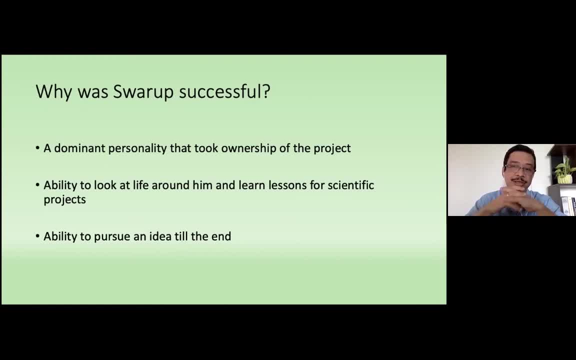 and he did everything. He studied engineering from textbooks. He was a physicist, actually not an engineer, but he studied engineering. He went through the accounts, he managed the finance. he got people to meet the vendors and taught them how to talk to the vendors, not to let them cheat work with the private. 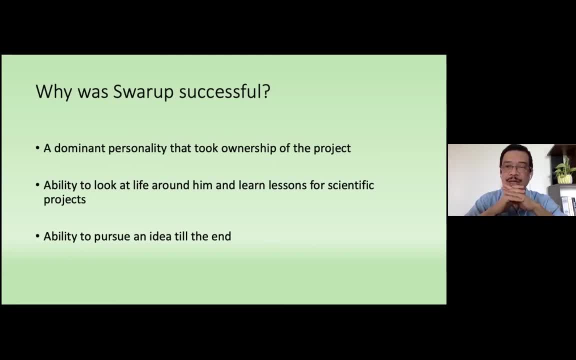 companies check everything, And he would never let anything go unless he was completely satisfied. And he had a limited ability to look around him and learn lessons for scientific projects. So this would mean that he would you know these lessons he would take from the novels. 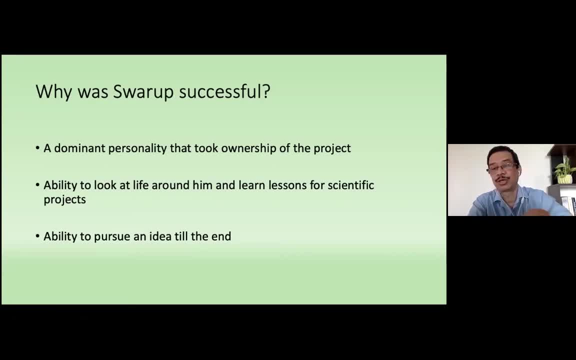 of Premchand, which he read as a child, to what he saw around him in Thakurdwara: how people made baskets, how they gave curvature to baskets, an idea that he used in giving curvature to GMRT, the dish in GMRT. 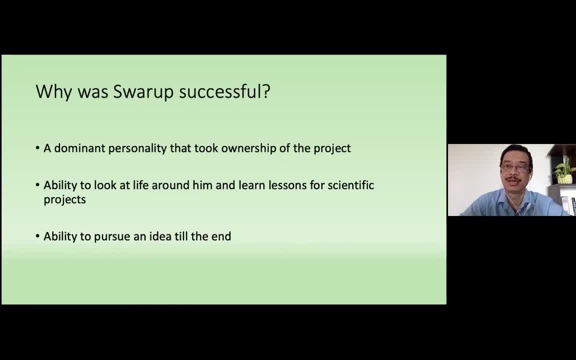 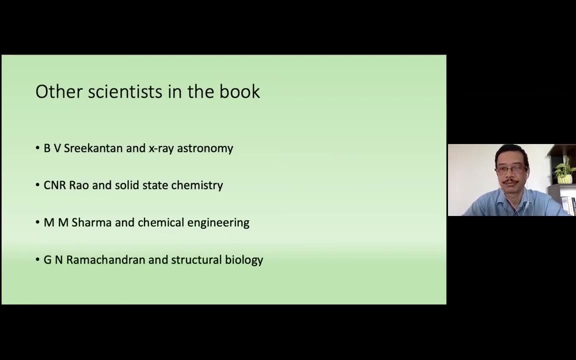 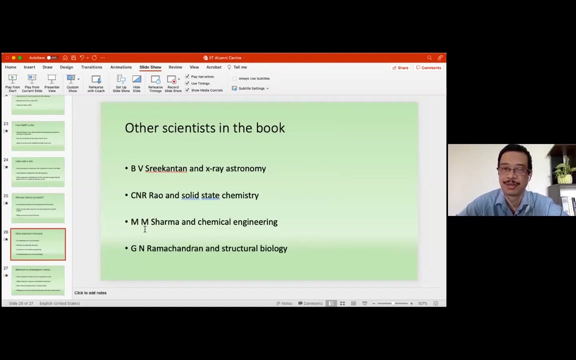 And he had a doggedness and he would pursue an idea till the end, no matter what, And I'm sure many people would have these qualities In those years. you know those were So. BV Srikantan created X-ray astronomy in India. 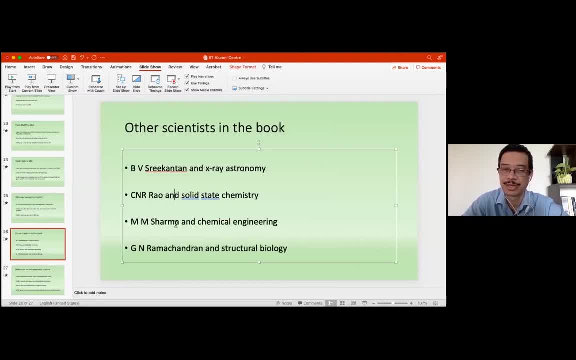 Sienna Rao similarly created solid-state chemistry. MM Sharma created, not created chemical engineering, but was a major figure in chemical engineering which who grew the field. JN Ramachandran was responsible for structural biology. So these were the people who built science early in the after independence and but. 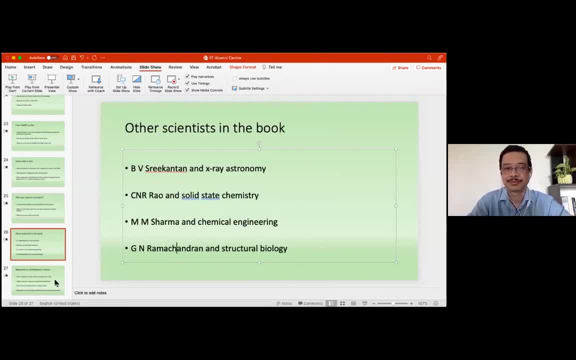 for them, Indian scientific infrastructure wouldn't be like this. Okay, What is the relevance of these people to contemporary science? So they had a fierce motivation to build science in independent India. They lived through the independence movement and they experienced it. It is one thing to experience the independence movement and another thing to read about it. 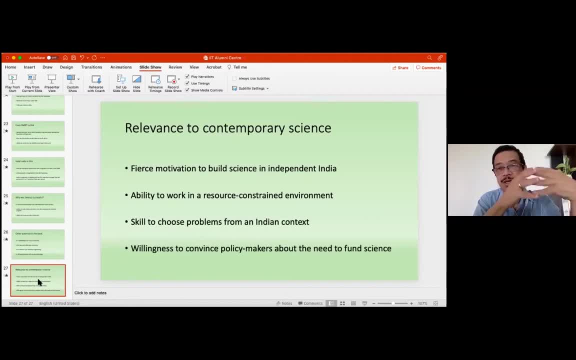 in from textbooks or other books. So they were all nationalists- nationalists in a good way. They wanted to build a new country And they believed that science was important. They all had an ability to work in a resource-constrained environment. Once again, this is a double-edged thing. 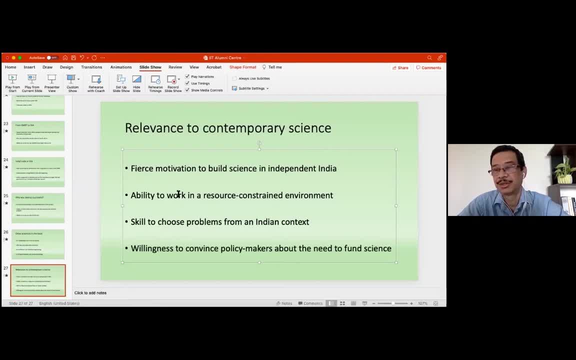 Not everything can be built in a resource-constrained environment. Some things need money, but certain things don't. And they thought about what they could do And they selected problems very carefully: things that they could solve yet were important Okay. 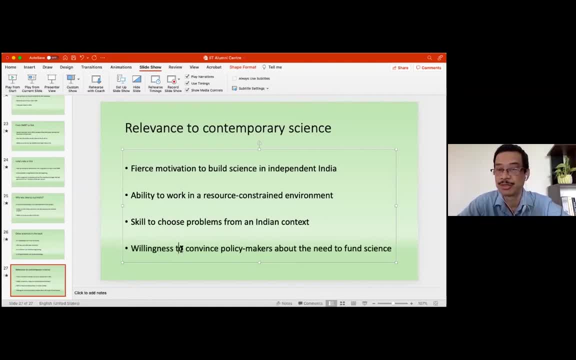 Now they had a willingness to convince policymakers about the need to fund science. All of them- Swaroop Sienna Rao, M M Sharma- they were all networked very closely with policymakers in Delhi and relentlessly pursued science. Okay. 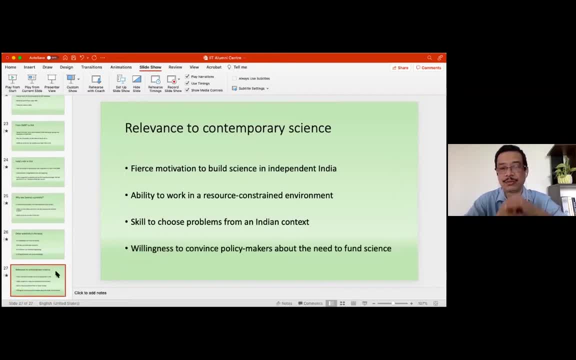 Okay, Okay, Okay. So from an Indian context. now we are sort of at a stage where we will always be constrained and resource-constrained. Money may not be enough, So we may have. we can probably take lessons from what they did. 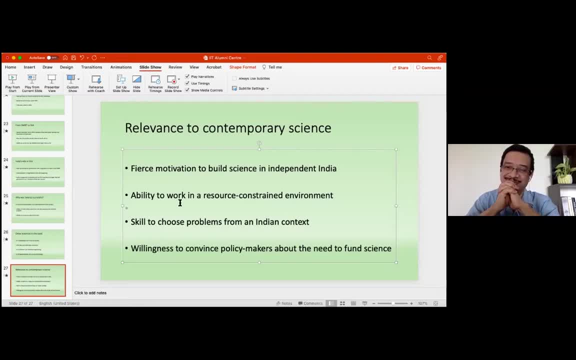 That's what I have to say. Thank you, I think I finished a bit early, Okay, So maybe we could… Stop screen sharing. Yeah, So, Shila, can I go first? Okay, So, Hari, thanks for that talk. 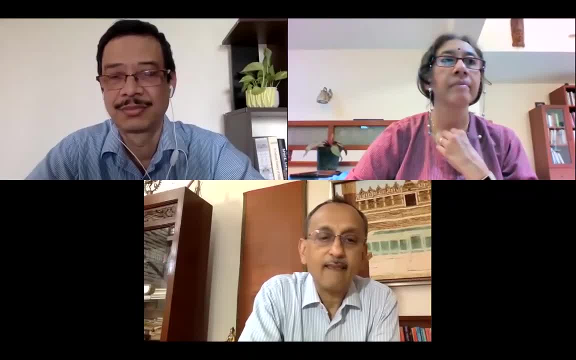 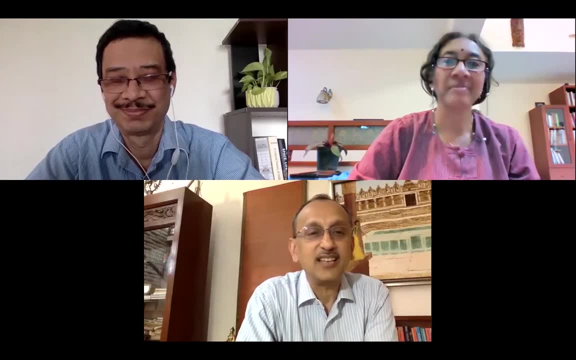 You know, in one of your concluding slides as well, you point out the importance of the fact of the number of people who are in a situation like this, And your talk was about the fact that we need to build a more inclusive and sustainable society. 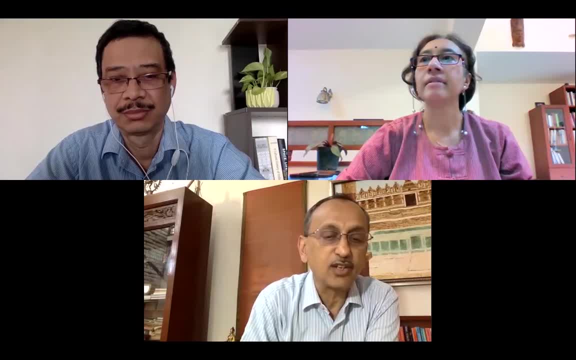 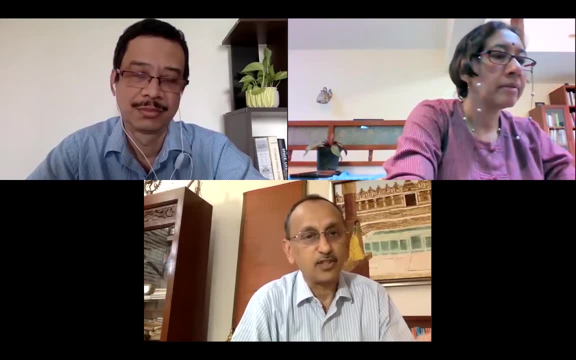 We need to build a more inclusive society. I think it's a great point. I think it's a great point. I think it's a great point, It's a great point. out other stalwarts like Prof Srikanthal, Prof C I Narayana Rao, Prof Sharma and others. 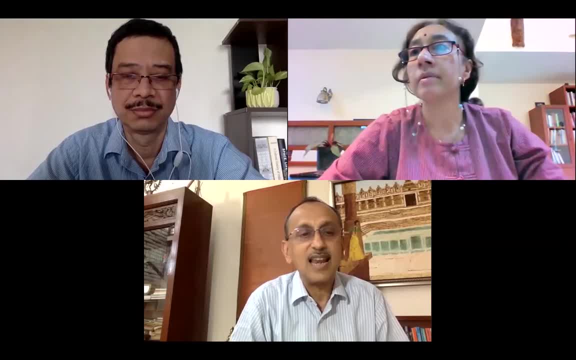 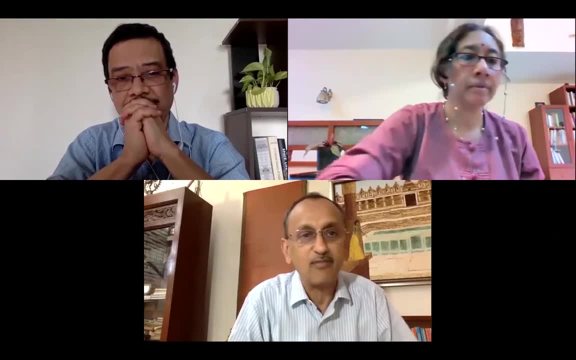 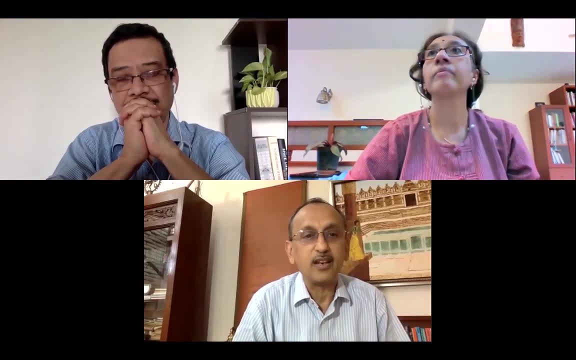 What, in your opinion, are the lessons that we can learn from the way these stalwarts actually built institutions? I mean, every one of them is a legend in some shape and form right. So what can we, in your opinion- and you've, I think, in the course of writing your book? 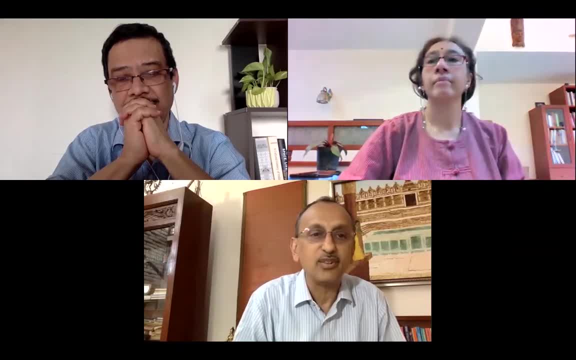 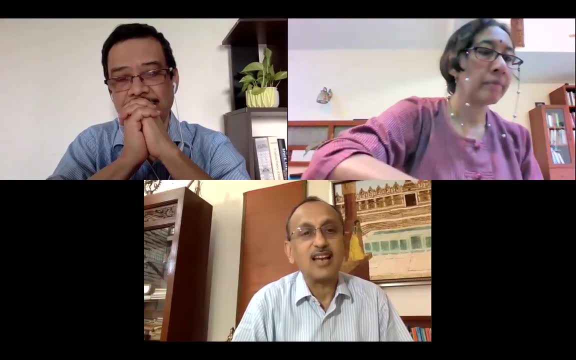 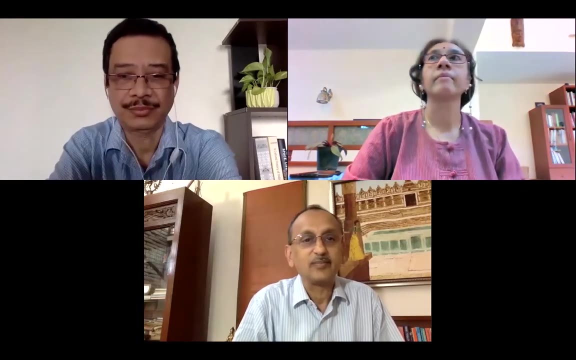 you've met them and interviewed them at length, or interviewed their colleagues as well. What would you say would be lessons that today's scientists in all these institutions can learn from? and, you know, build our scientific base. They all learned how to work with. 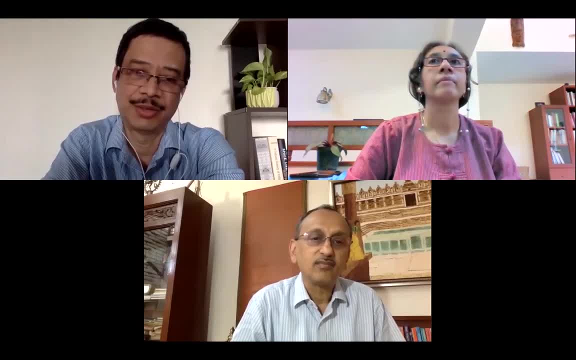 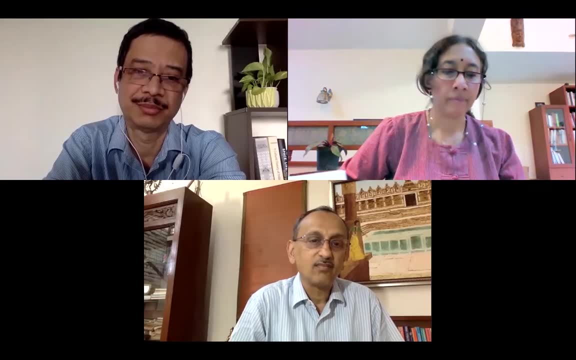 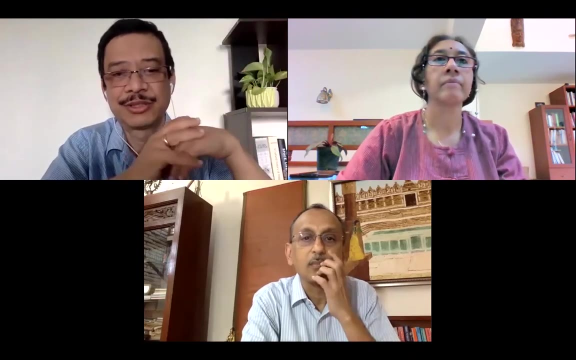 very little resources. That was the first. I mean resource. we are always in a resource-constrained environment. There will never be enough money for science. So there is no technique as such. in the sense there is no. it's not a methodology. 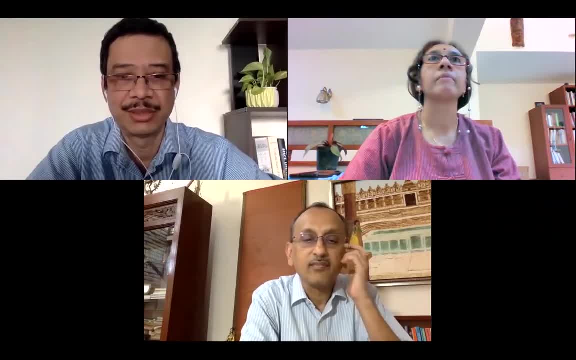 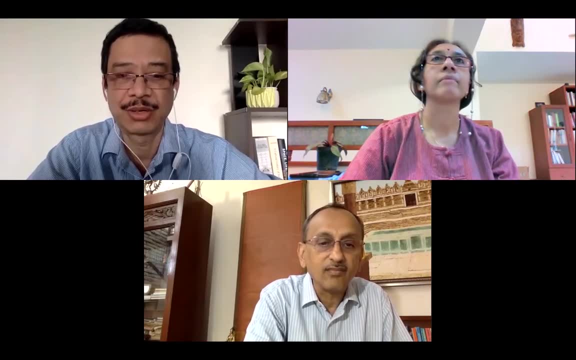 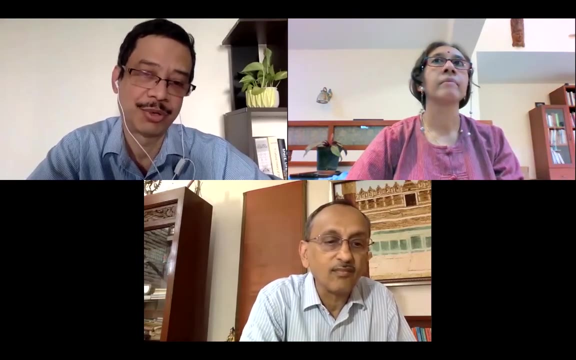 you know, like, as they say, Jugaad or something, but they knew how to get things done When you build an equipment. they knew, knew how to figured out how to find the parts easily. They chose the parts that they could get done. It's not a top-down strategy. it's more about 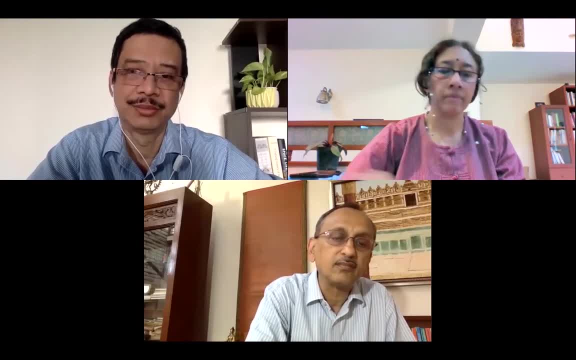 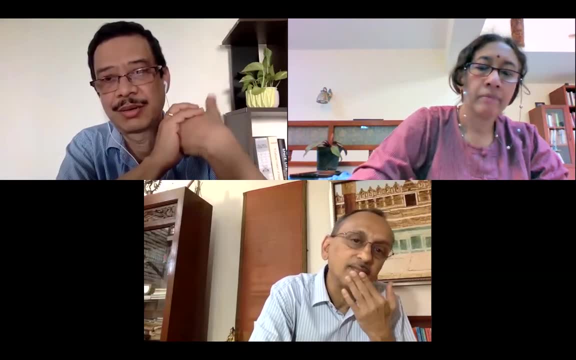 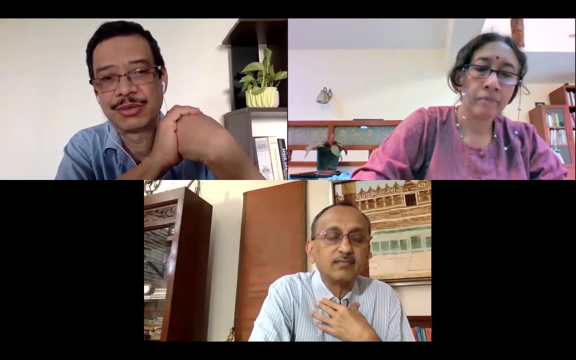 like you know what are the problems that they could do, And yet, important that is one, And the situation at that time was, you know, country. they all had a drive, which is because they lived in a newly independent country. So we don't have that kind of atmosphere now in the country We have. 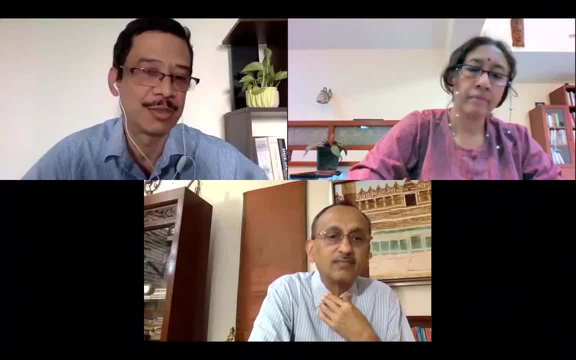 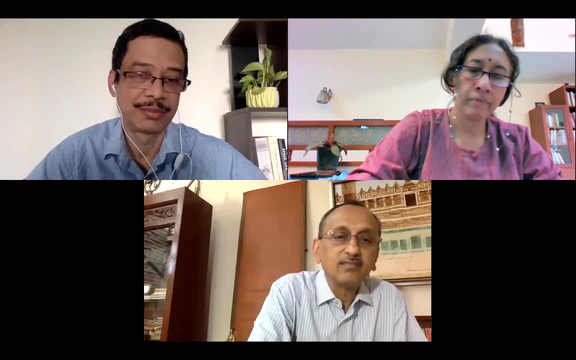 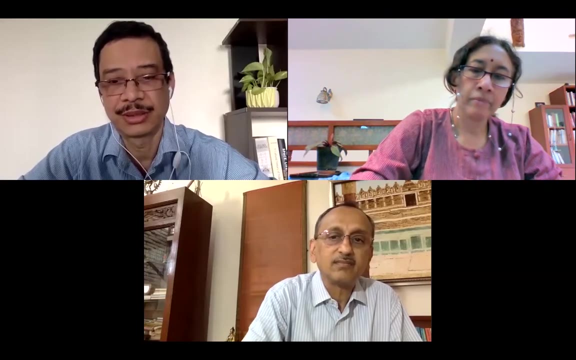 read about. I'm not sure we can get the same spirit at this moment. They all had good jobs, but they came back because they thought science was important And over a period of time, and people believed science was important at that time. Now that sort of belief has. 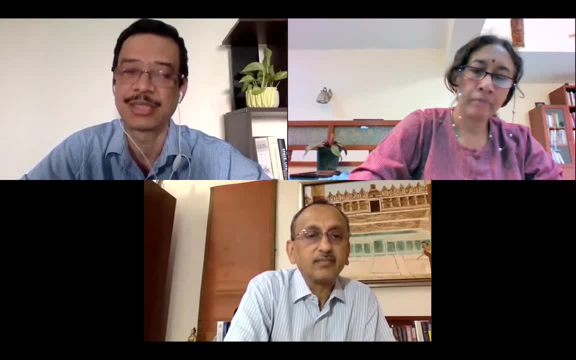 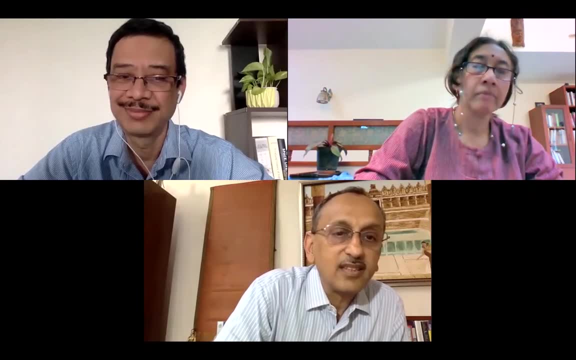 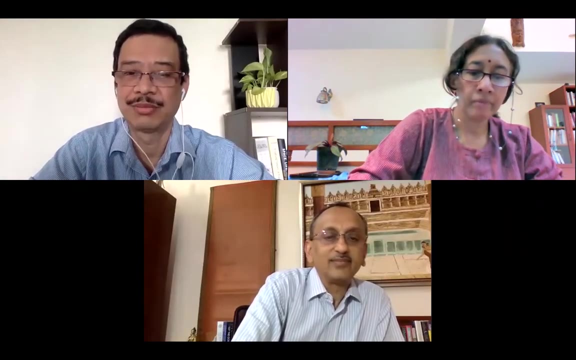 gone away from the public perception. at this point Science is a big distance. At that time science was not distant. Science is a bit what Science is a bit distant from the public. It was not so in those times. I mean at least those who were educated and who read newspapers. 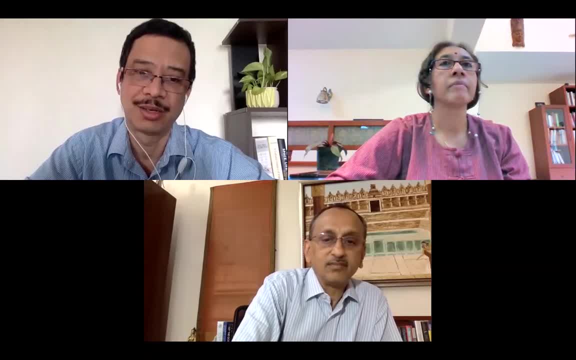 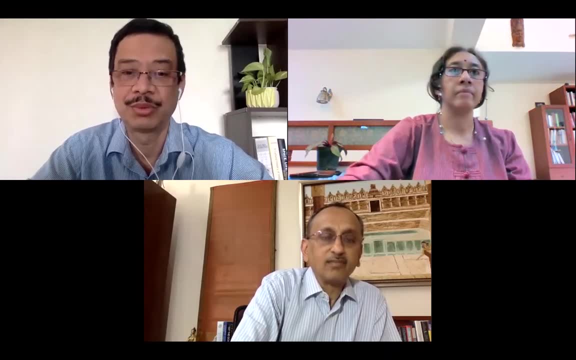 So it is probably a function of the times that they did well. Also, it is you know you cannot transpose what they did to the current context completely, Because we are now judged. We are not building a foundation anymore. We have to compete globally. 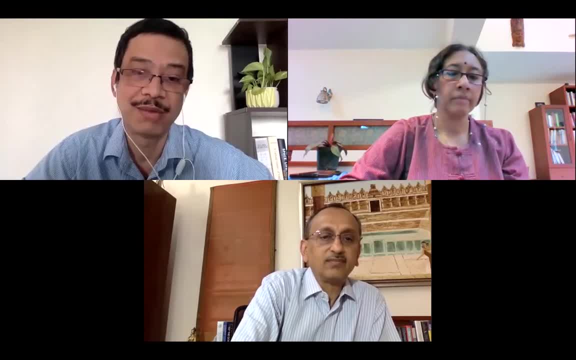 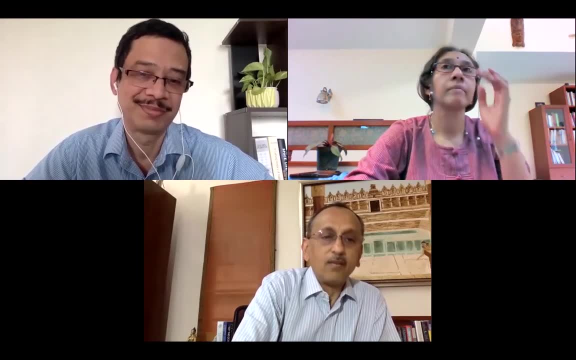 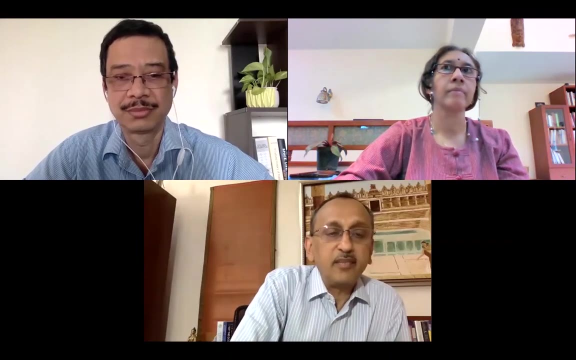 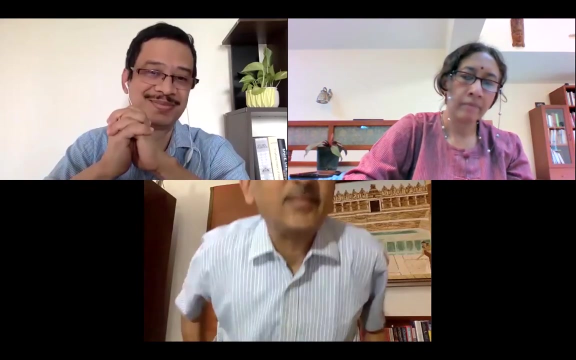 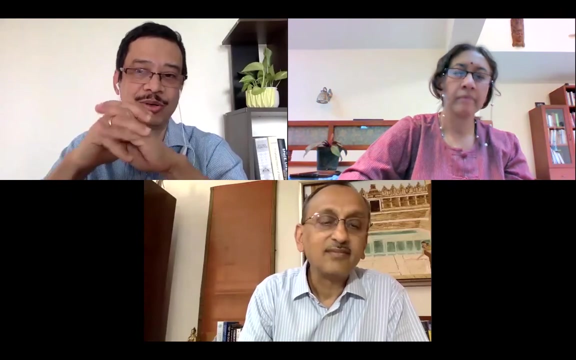 So we cannot choose problems that can be solved. We have to do problems that have to be solved, So find a way. So would you advocate more investment in basic sciences? if you are talking to policy makers, Yes, It all depends. It's all relative. What is basic science? I don't know whether there 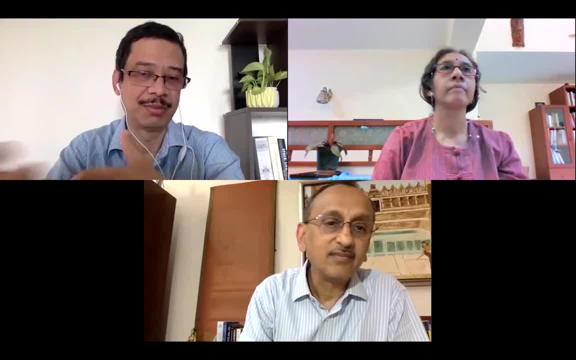 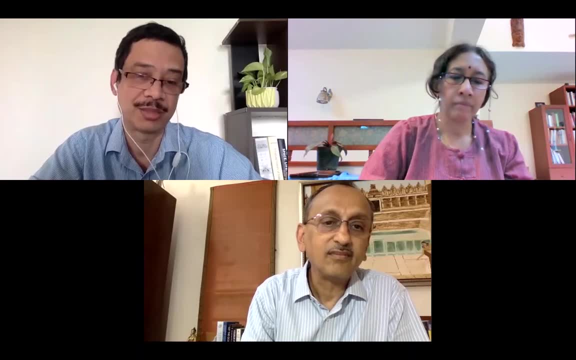 is such clear divisions between basic science and applied science. Some of these projects you know- SKA that we mentioned and the other big projects that India is part of: international projects, a fusion project, ITER in France, the LIGO. 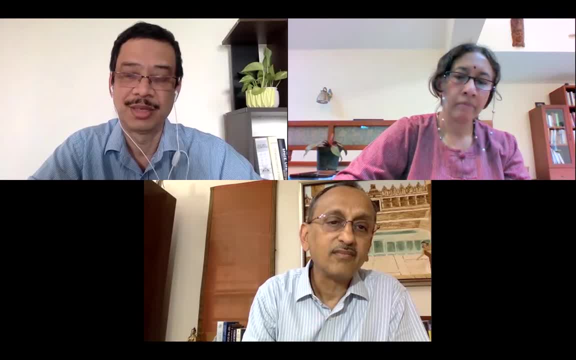 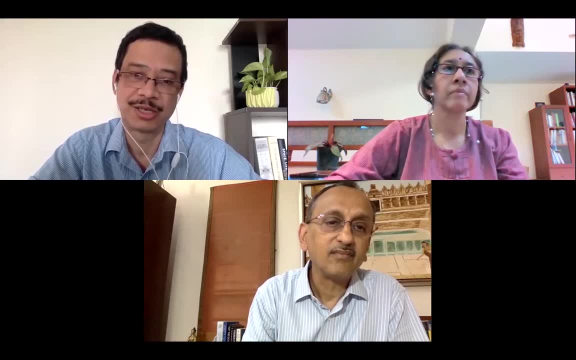 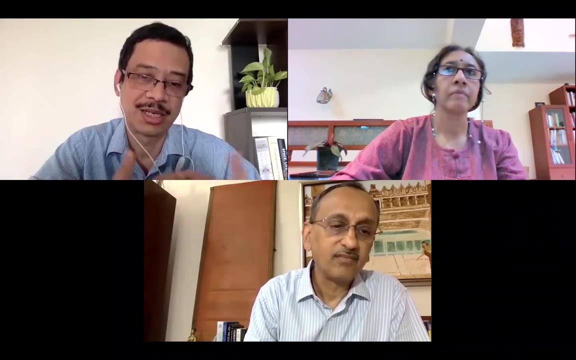 India's own, the TMT, the optical telescope in Hawaii. all of them are big projects and they involve a lot of engineering, And science pushes the frontiers of engineering. you know So because if you're tackling a scientific problem, very often you would find that you would need an 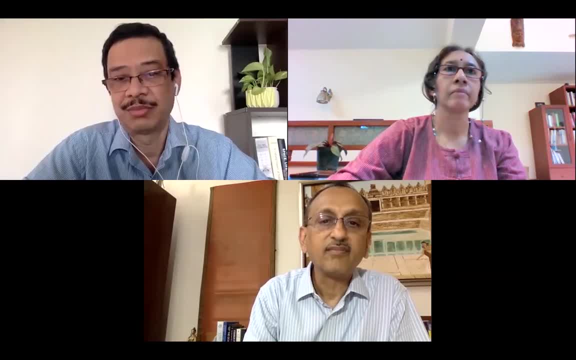 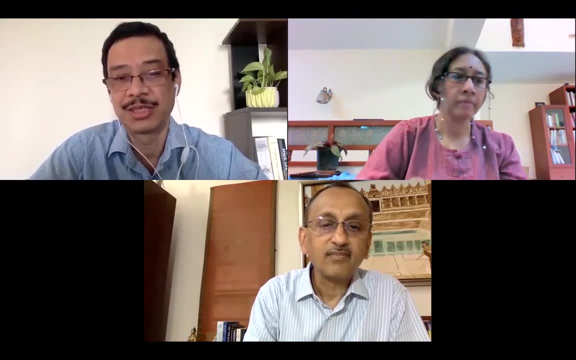 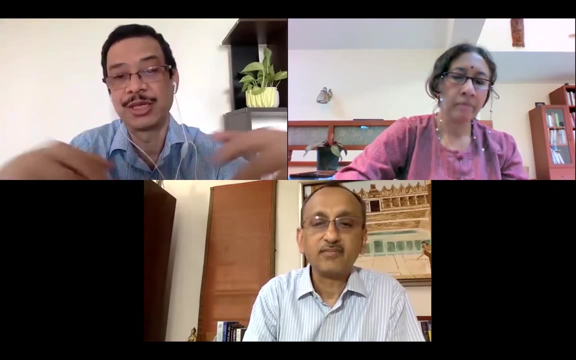 instrument that has never been built, Because a lot of scientific problems require instruments that don't exist. So when you build them, you build capabilities in many different areas, Areas of technology, So each of these areas can develop into full industry at some point. 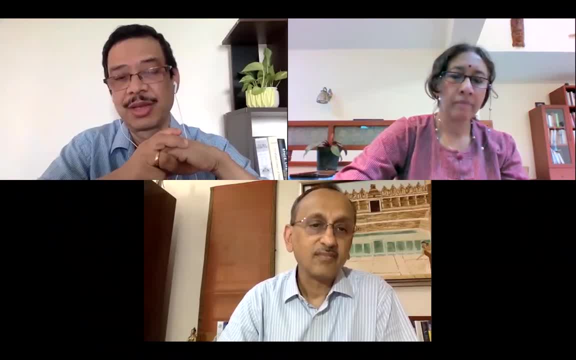 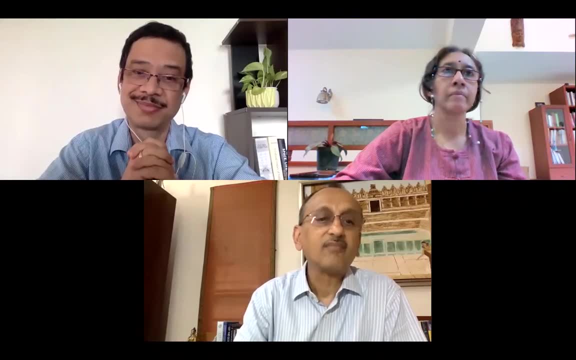 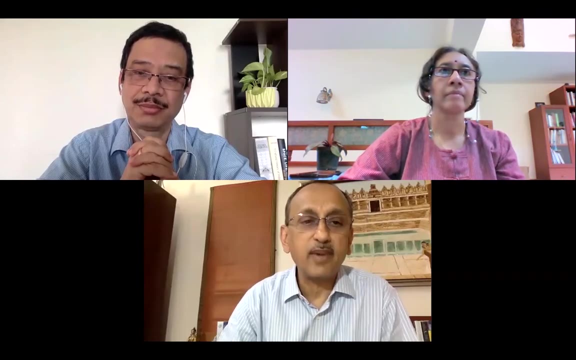 Sometimes they don't, but sometimes they do. So investing in fundamental science in many ways is actually investing in technology, in applied science. So I know you know when you write a book you probably are constrained by you, know how much you can write And you know it also can't be a thousand pager. 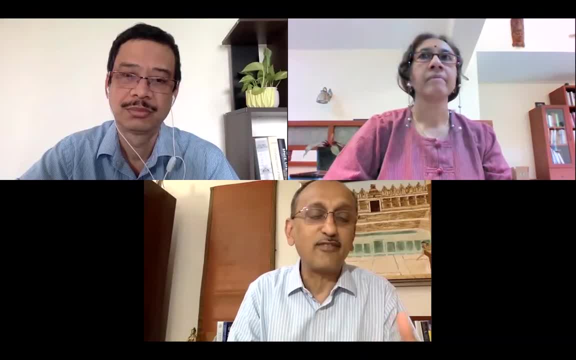 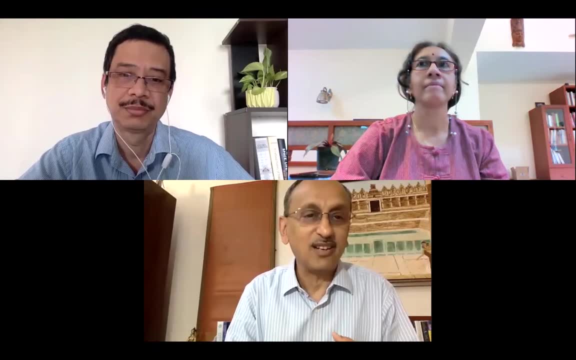 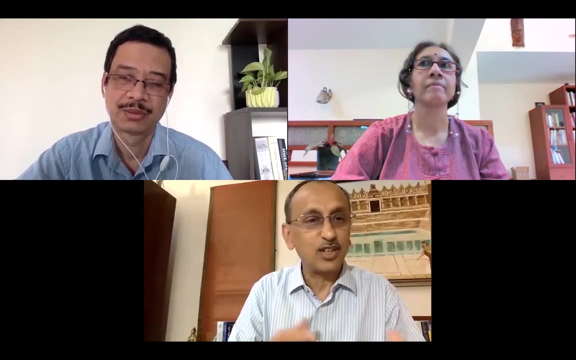 And so you miss out many things. But just to kind of ask you your opinions on a few things: like Professor MGK Menon, also a stalwart, What's your, you know? have you researched him at all? Yes, yes, yes. 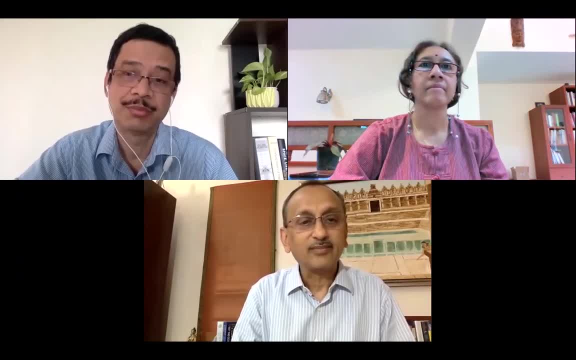 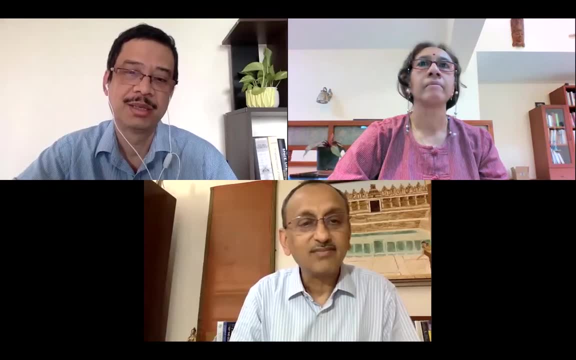 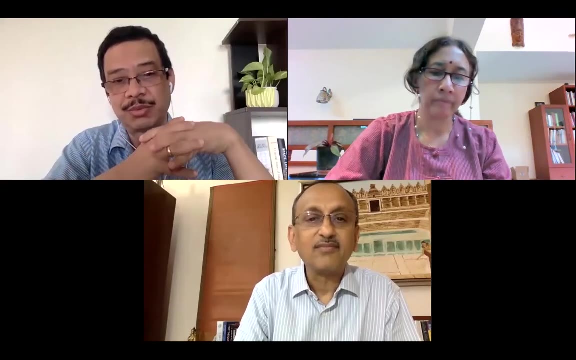 Do you have any comments that you can make? Yes, he was an important. He was BABA's deputy And for Swaroop himself. when he came back, MGK Menon made sure that he got all that he wanted. It was a very smooth transition. So even the equipment that he wanted in TI-FAR were there when he came. 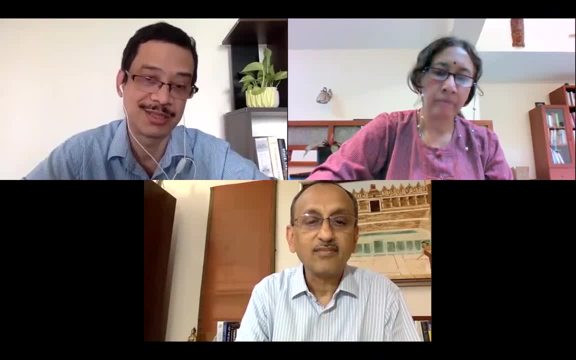 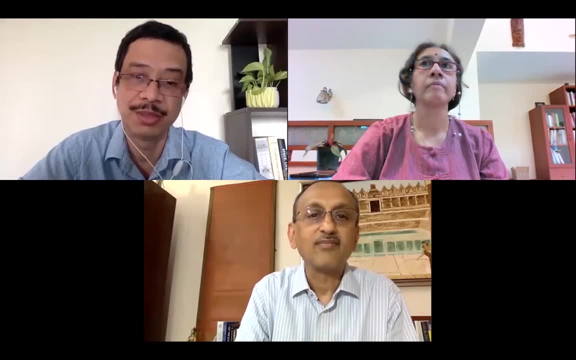 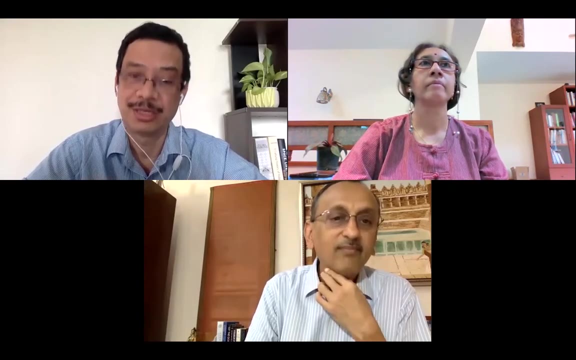 But unfortunately he had big ideas and that equipment was not really enough for him to work with. But MGK Menon supported big ideas and After BABA died he was the director of TI-FAR And then later he went to Delhi and he was a big figure in clearing big projects in the country. 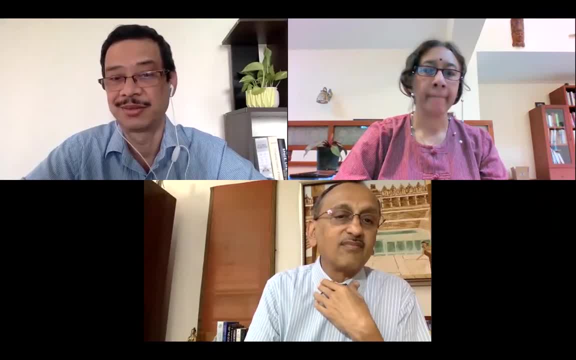 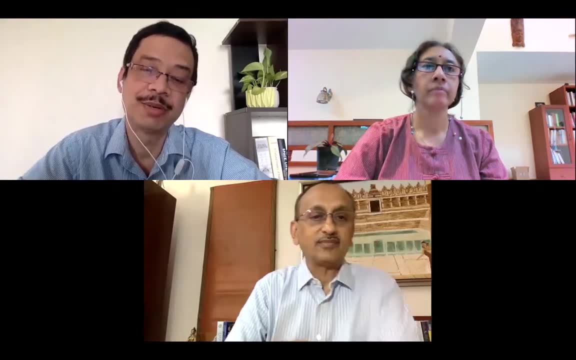 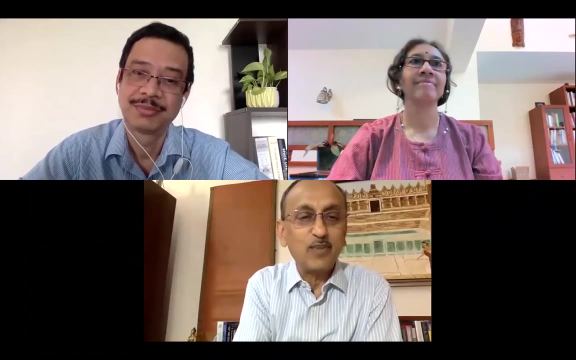 Without him, some of those big projects could not have be cleared, including GMRT. You can't write about everybody. This is not a history of Yes, yes, yes, No, no, you know, but since we're chatting about all these inspiring and inspiring projects, but it's a long way from here. 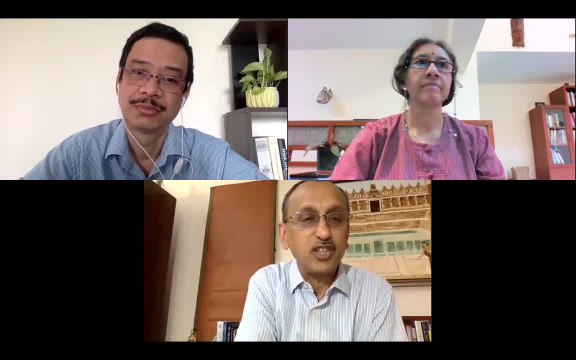 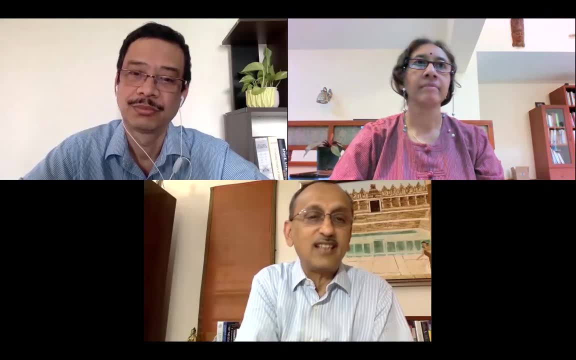 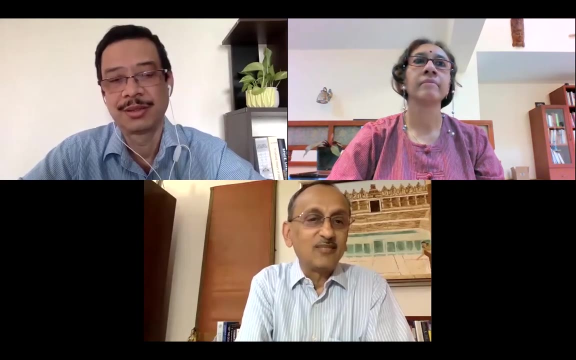 You're looking at also people like Professor Satish Dhawan or Dr Vikram Sarabhai. These guys laid the foundation of institutions like the Indian Space Research Organization, Dr Yes. well, the foundation of the Space Research Organization was done by Sarabhai, led by Sarabhai. 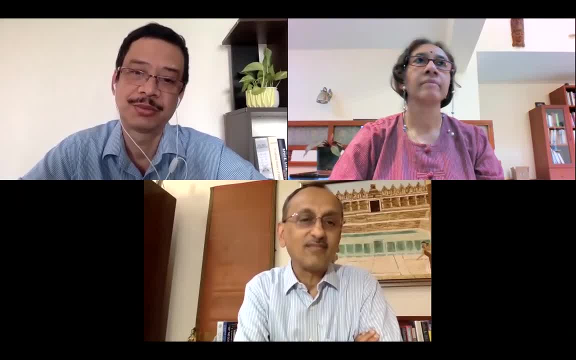 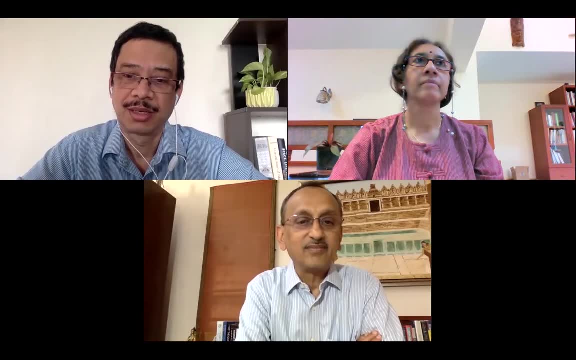 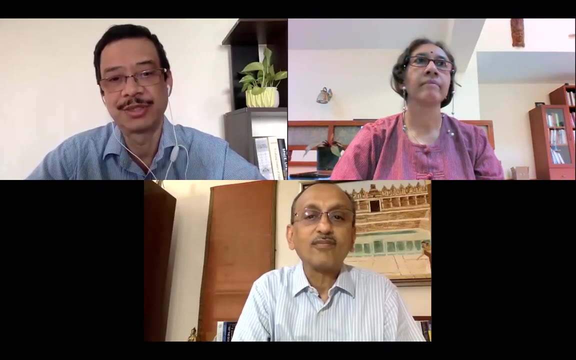 And Bhabha also had a role in it because Sarabhai it was part of the Atomic Energy Commission when it began and Satish Dhawan came later when Sarabhai died. But he had a role because he smoothened everything and he was very good at administration. 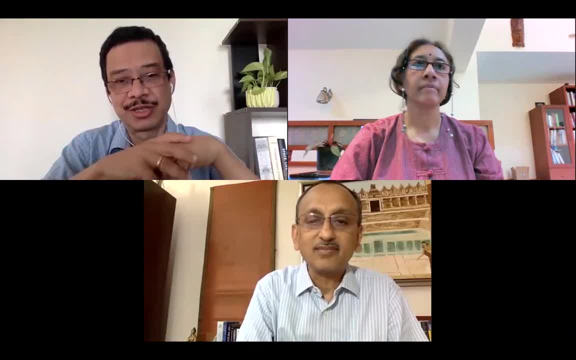 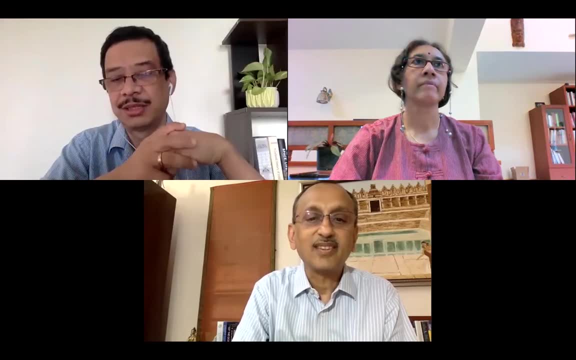 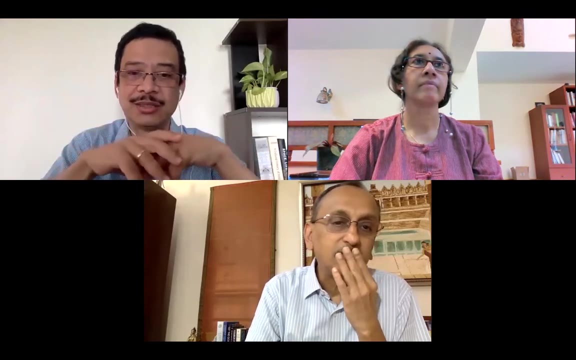 He put procedures and made it a well-functioning machine, and he made it an open organization also. It's not that it was not open in the beginning- it was, But then he had instituted the system of reviews where anybody could ask anything. 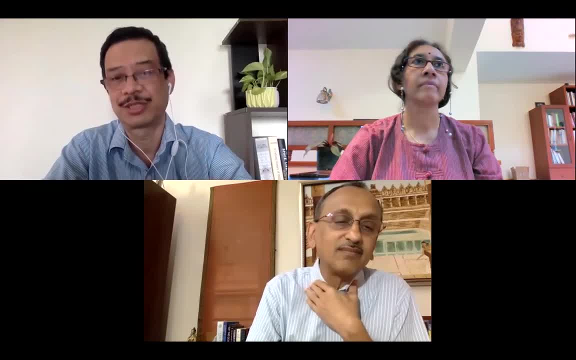 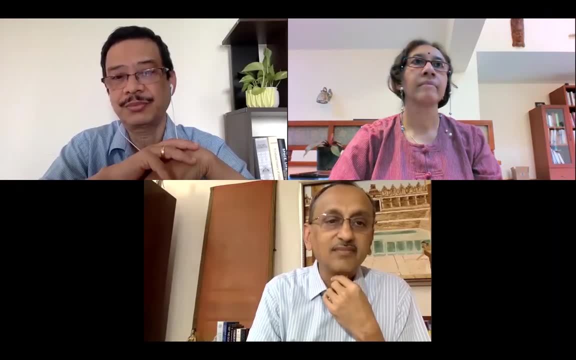 There were no hierarchies. even the most person could ask any question. So that culture remained in ISRO for a very, very long time And Satish Dhawan had a. his role in building Indian Institute of Science is not that well. 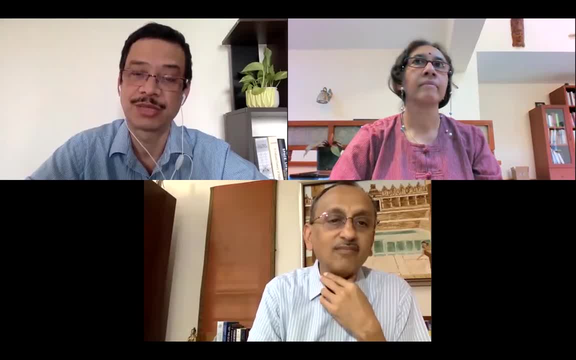 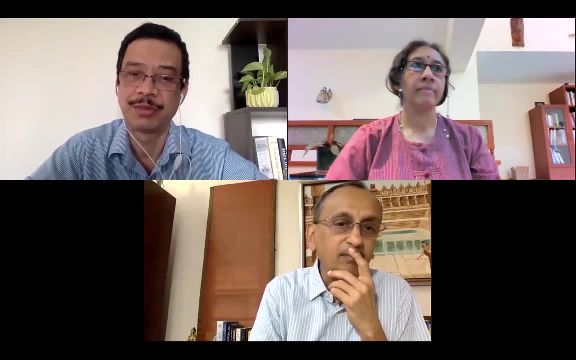 known, But he, it was he who transferred Indian Institute of Science. He hired a lot of people in. you know, I heard that he is a Dr. Yes, He hired about 60 to 70 people in one year. went around the world, met young scientists. 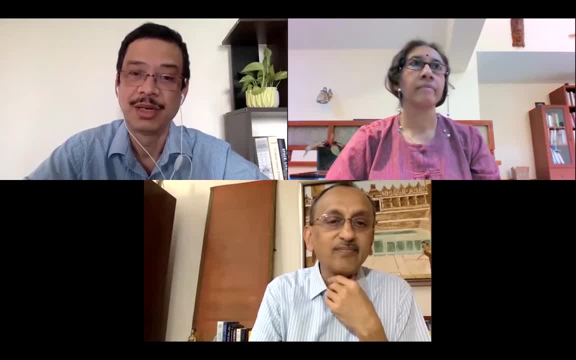 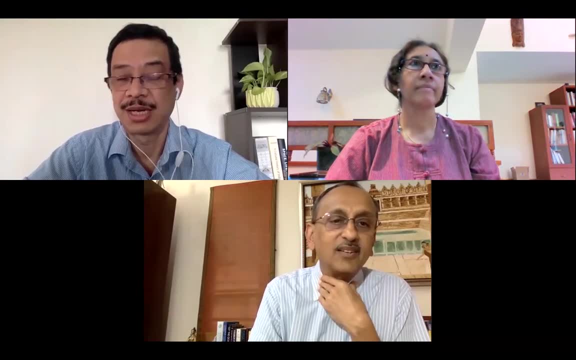 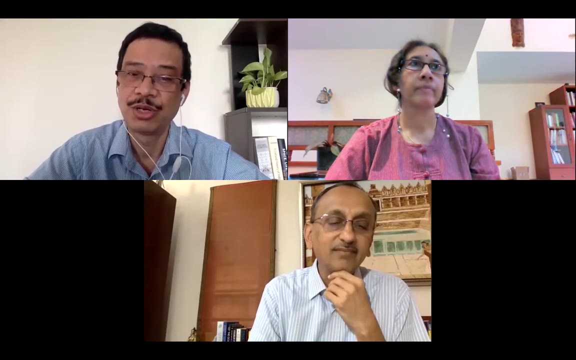 and offered them jobs, made them come back And he grew the institute from a small institution to a big institution And he was handling soon after that he was handling to space and IIC at the same time And, of course, slowly over a period of time. I think his attention was more focused on 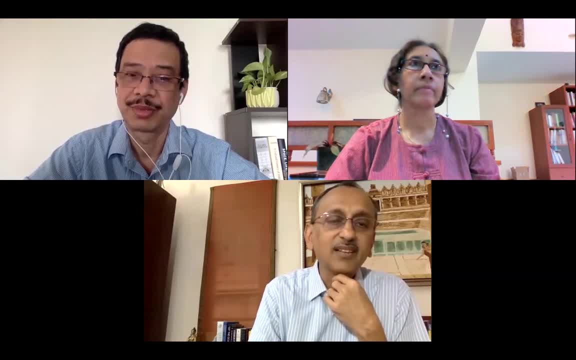 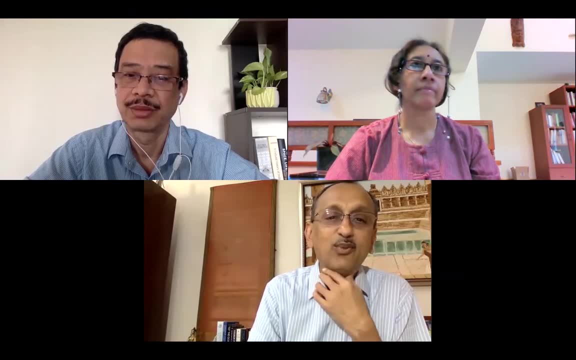 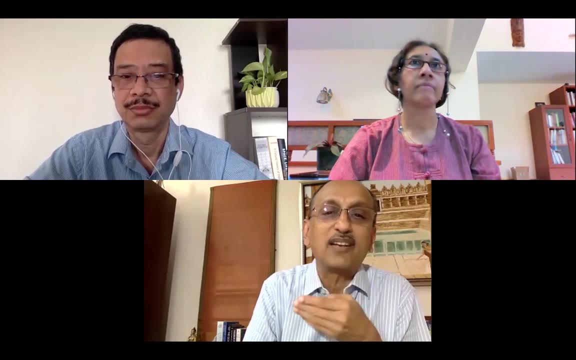 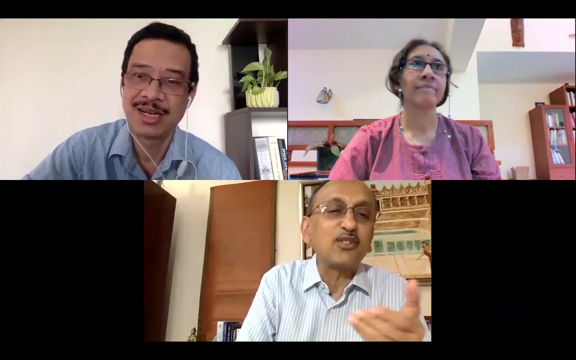 space, Dr. Yes, Thank you, Dr. So during your research? so there's an interesting question from somebody here. It says: why is the current scientific environment? why are they focusing on radio astronomy rather than optical astronomy? I don't think anyone's looking for a technical answer, but in the interviews, yeah. 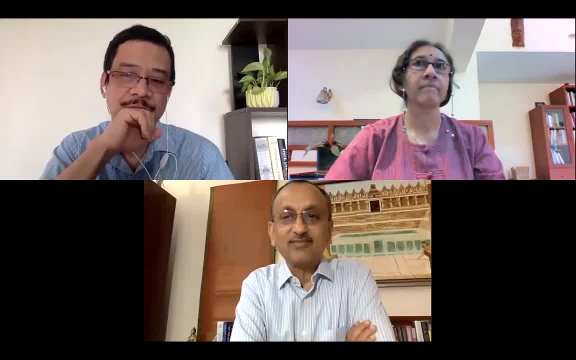 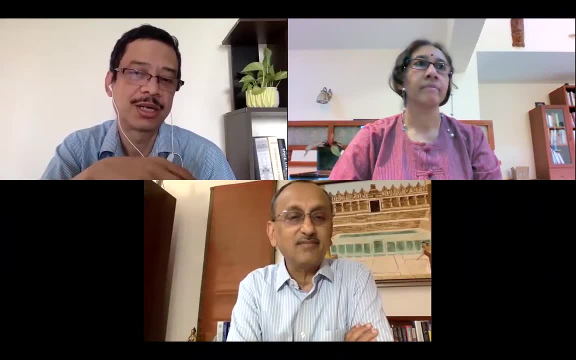 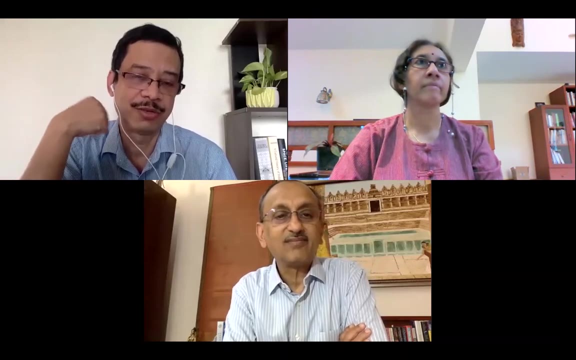 Dr. So in radio astronomy, Yeah, Yeah, Yeah. In radio astronomy they try to do what they could do rather than what they can tackle the biggest problems that they could not do. So optical astronomy requires a lot of investment, much more than what India could afford at. 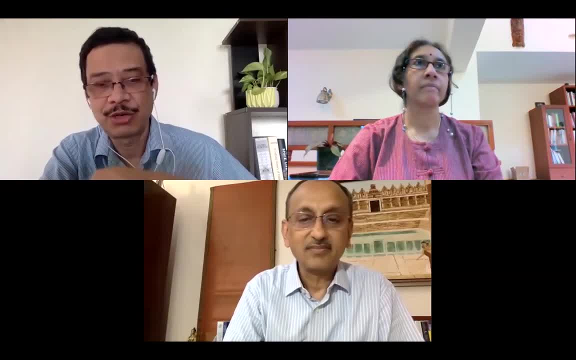 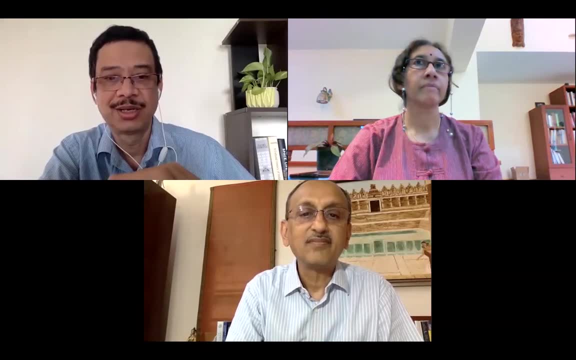 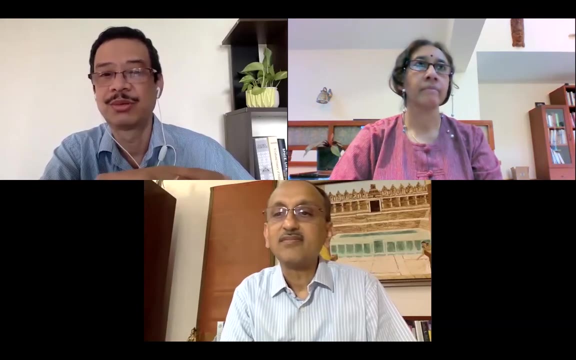 that time, And even in radio astronomy they stuck to low frequencies, where you don't need to cool the equipment to very, very low temperatures. You could work at normal temperatures. So even the UT telescope and GMRT are both low frequency telescopes. 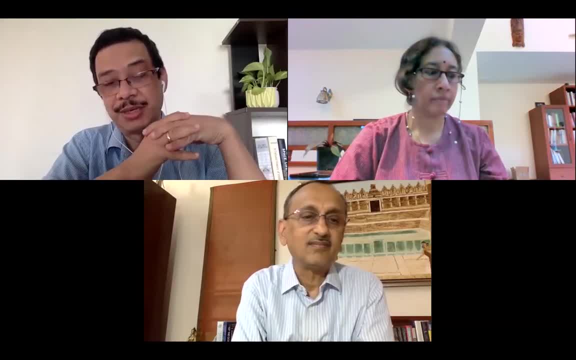 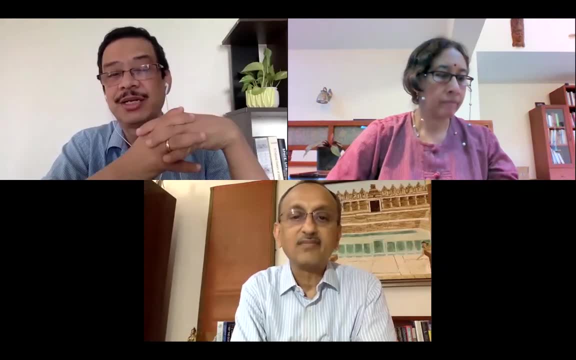 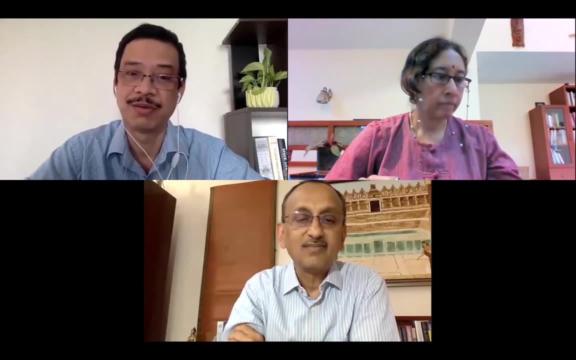 So, and they were built at a place where there was not much radio noise at that time. So they selected the problem carefully And this was an area where India could do something with that limited resources. So in optical astronomy we still don't have a big telescope. 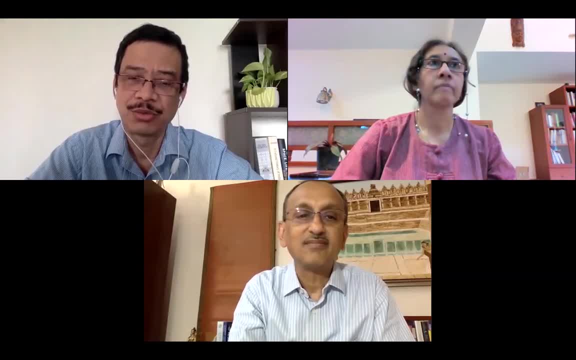 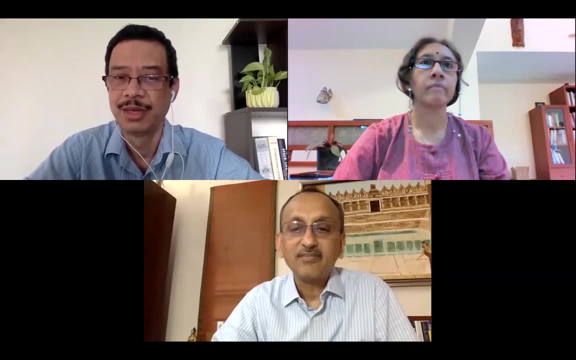 I think the biggest is in 90,000.. It's about 2.5 meters or something. I'm not sure exactly how much. it is somewhere between two and three meters. Well, around the world people have gone more than 10 meters. 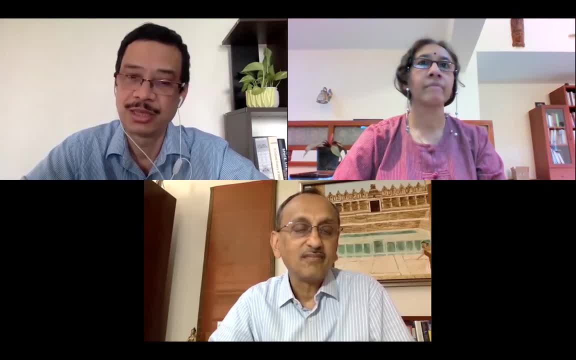 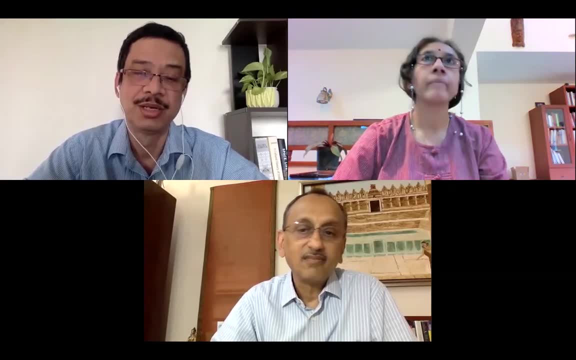 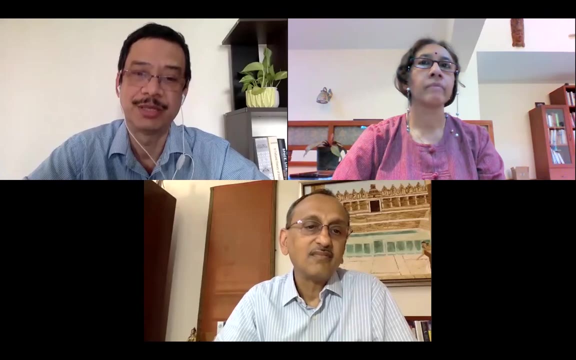 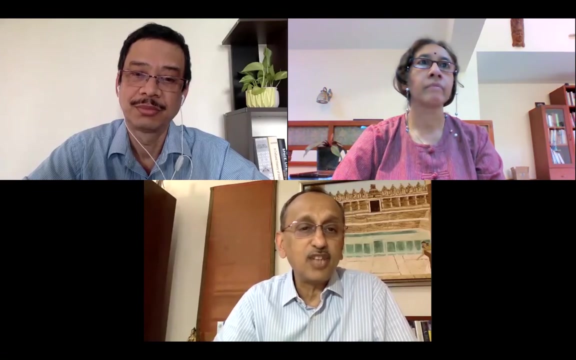 So that requires an investment that was beyond the capability of India at that time and even now, and probably of most countries at this time. So that is why these joint global projects- PMT is an international project, many countries shipping it, So I think, with the Hubble and now the James Webb going up, you have better resolutions. 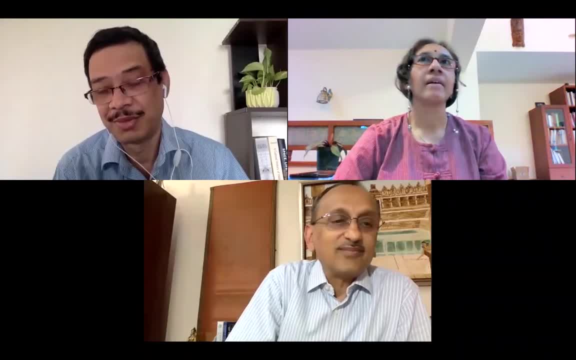 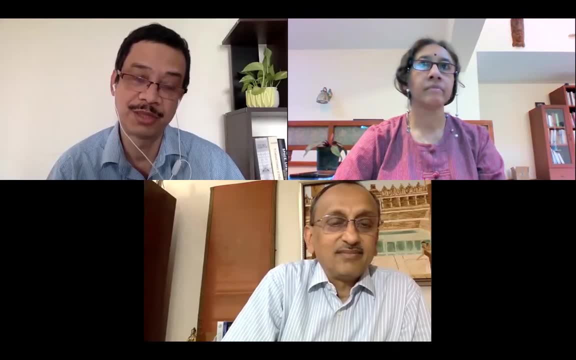 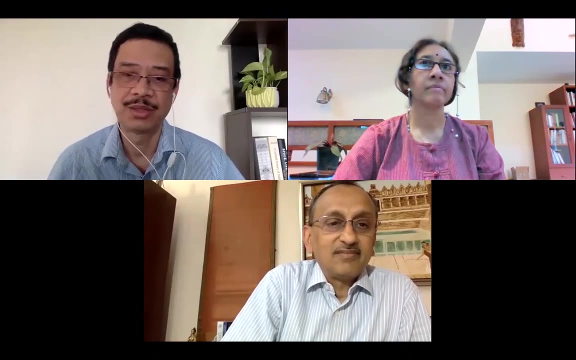 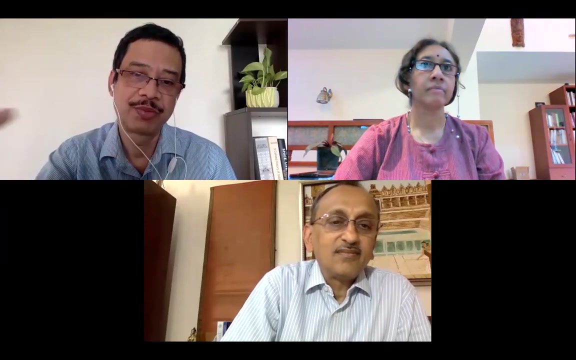 out there. Well, I think, as far as I know, people have figured out a way to do optical astronomy from the earth. They can match these space telescopes. They have this technique which they use to Compensate for the atmospheric effects, which will give images as good as what you. 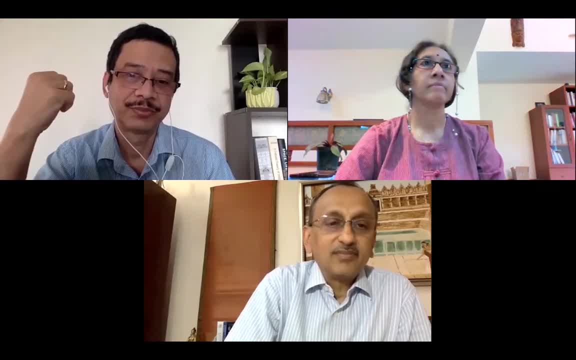 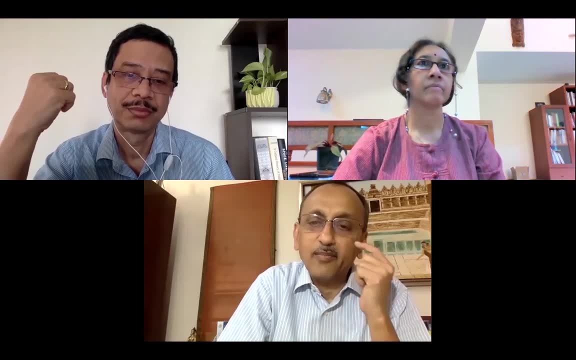 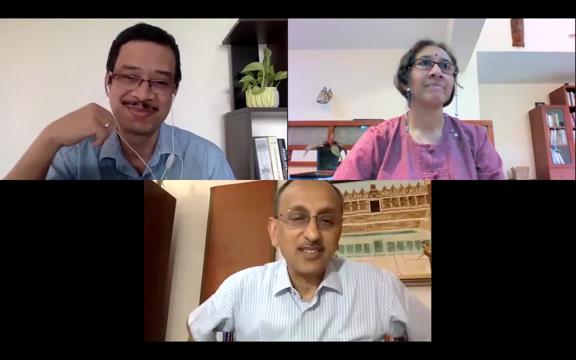 can see from space, Space. Yeah, There's an interesting question here. that kind of is an extension of what you've been talking about. It's called adaptive optics, So I just couldn't get that. Yeah, Adaptive optics, Correct, Yeah. 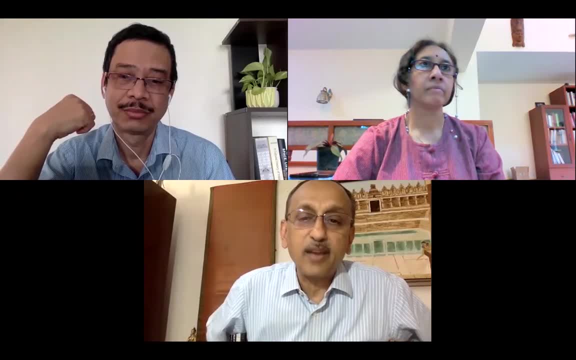 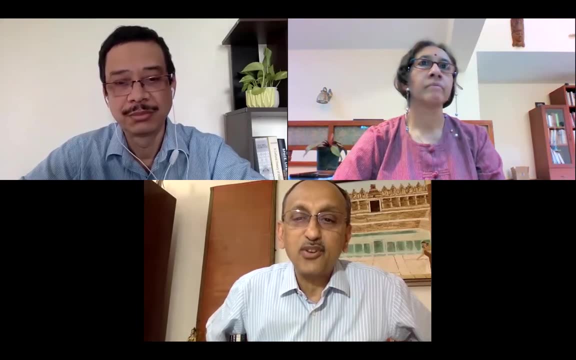 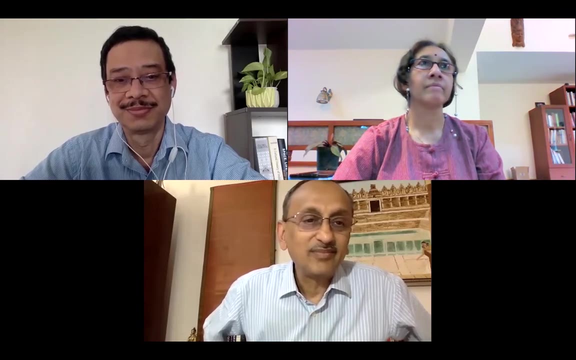 So I would just add here something that you just talked about when you are in the context of Dr Sarabhai. The question the person is asking here is: vertical hierarchy to horizontal hierarchy in science. What are your suggestions? I don't have an answer. 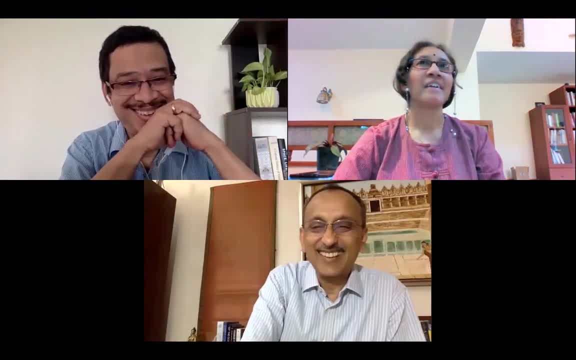 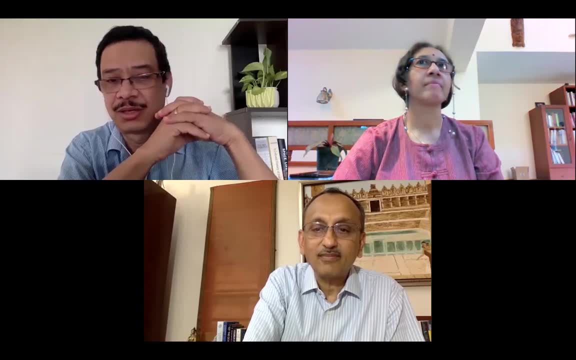 Well, every you know horizontal hierarchy. I mean I'm sure in most institutions it's not. I've seen it. It's not. It's not um, are not that hierarchical in the, in a, from a scientific point of view, that people have the. 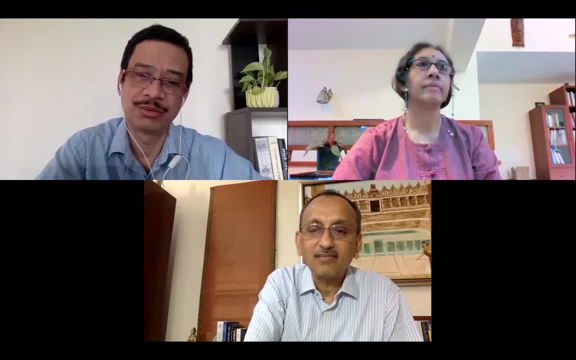 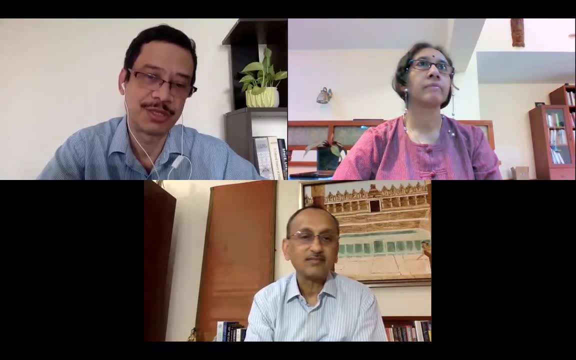 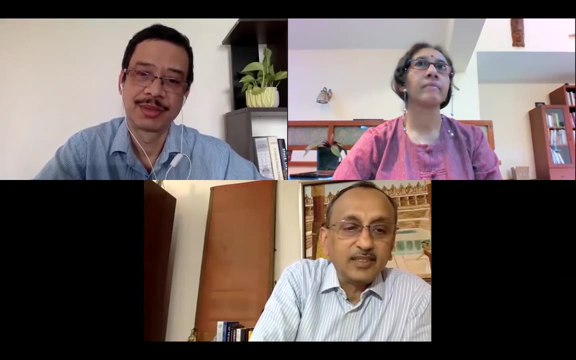 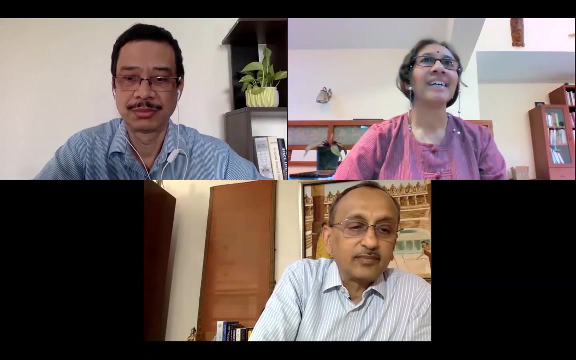 freedom to choose a problem, whatever they want to do. i don't think directors influence that much. it's a question of the ability to convince somebody that that you, this project is important, and the ability to get funding more than anything else. so, sheila, you want to ask the others? yep, thank you. so here are a few questions on. 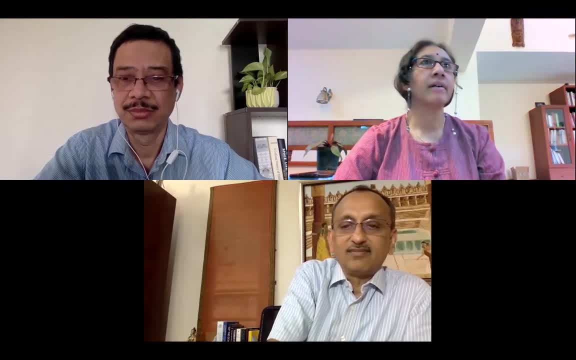 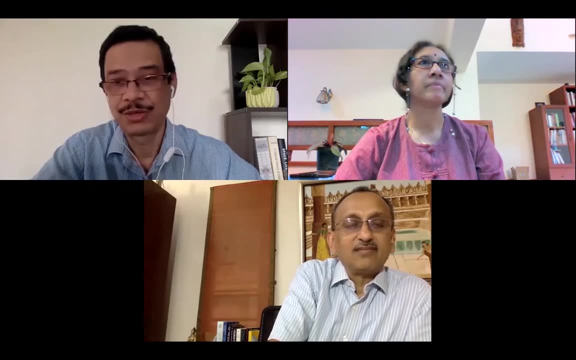 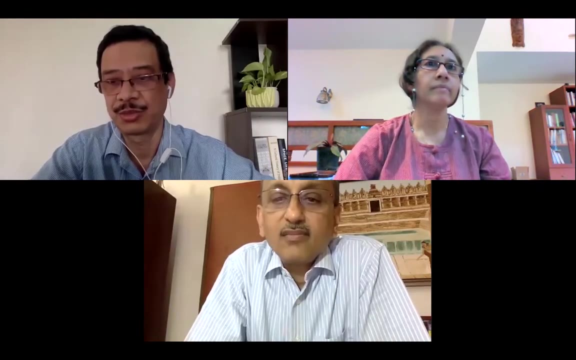 where does india stand with respect to other countries in term in the field of radio telescopy? well, india is one of the top nations. now, i mean, if you say this is a very arbitrary list, but if you pick five countries in the world, you can say that india is one of the top nations in the world, and if you say that india is one of 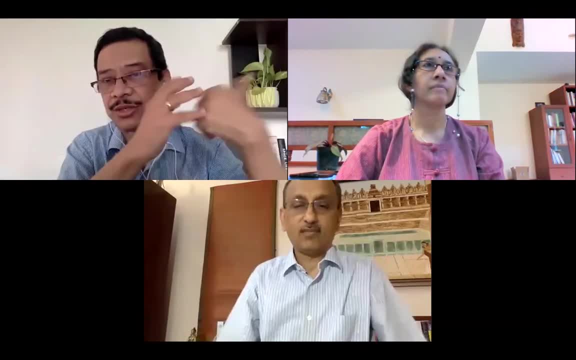 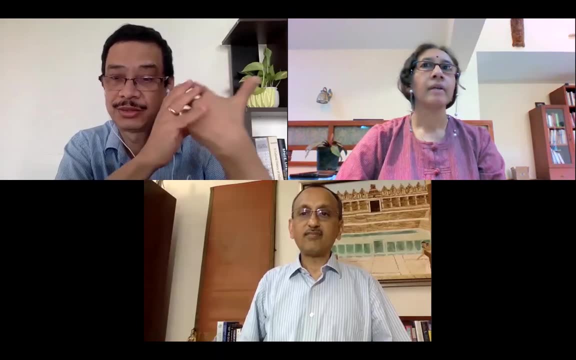 the top nations in the world. and if you say that india is one of the top nations in the world, um, who do with the larger india astronomy community, who tackle the big problems in radio astronomy? we would pick india. well, 30 countries, 50 of the proposals from uh gmrt is from outside. 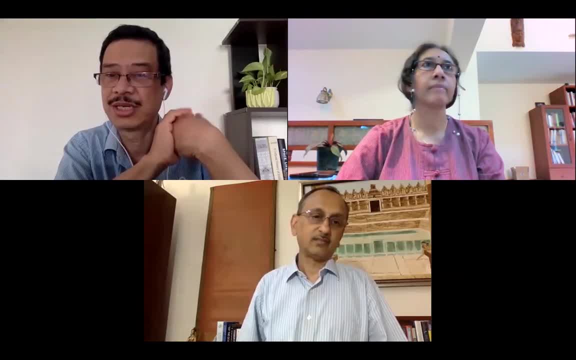 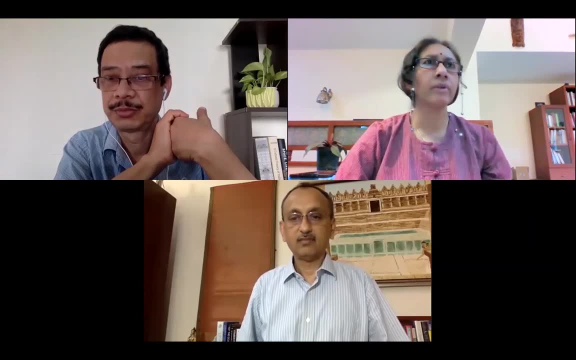 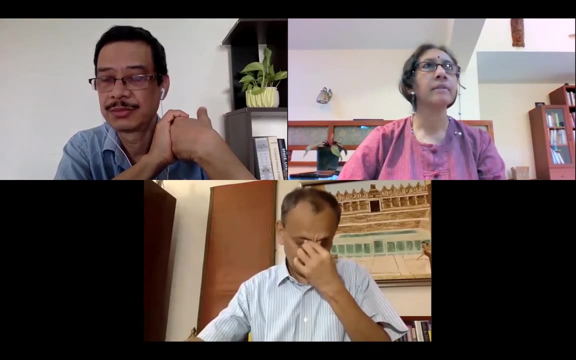 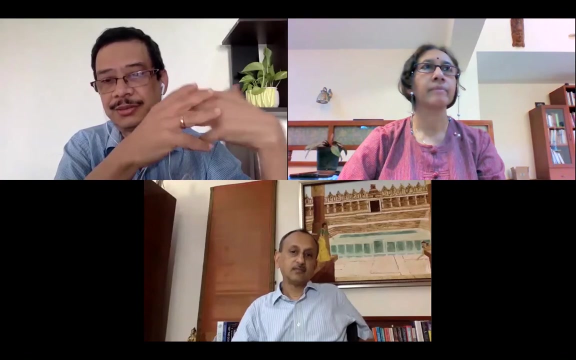 india and 30 countries use it. i don't think there is any equipment in india which is used this way. and what are the? in your research, what did you find are the important problems that people are looking at these days using the radio telescopes? so, as i said earlier, ready all objects. 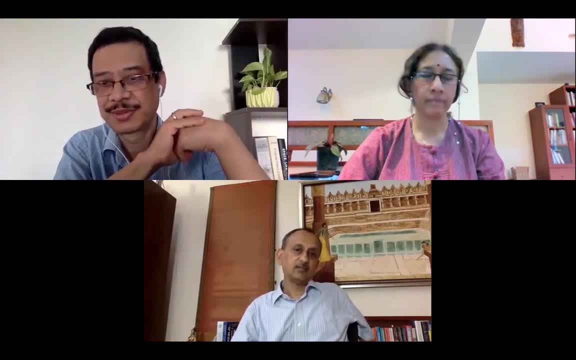 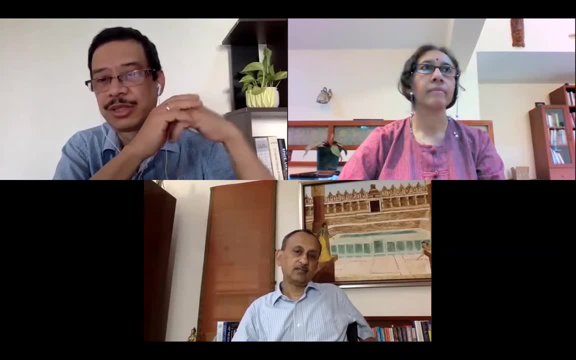 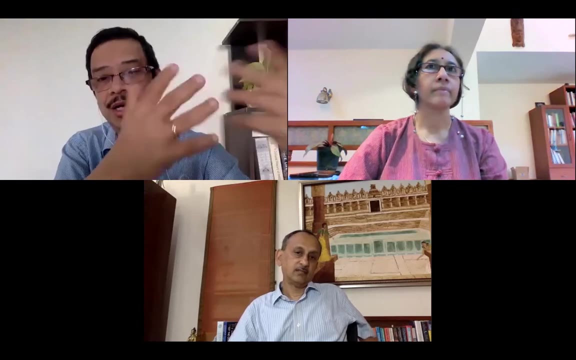 at all temperatures give off radio waves. so this is a. this is a big thing for radio astronomers, because with optical telescope you cannot. you can only look at bodies at high temperature and and with um, ultraviolet and x-rays, even higher temperatures. of course, x-rays are very good at looking at. 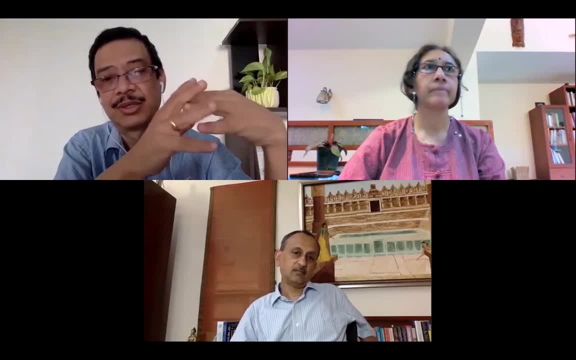 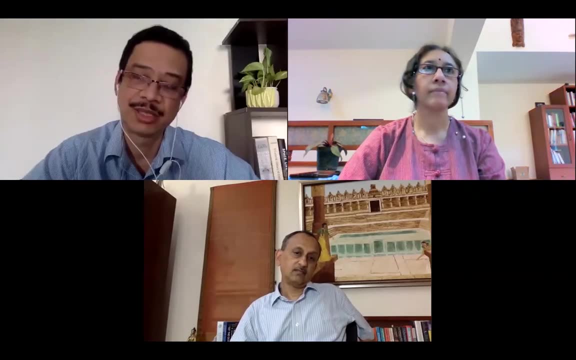 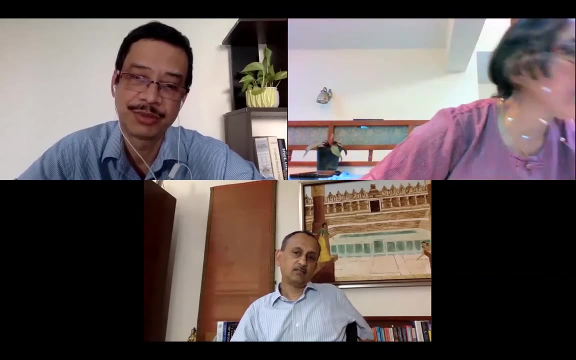 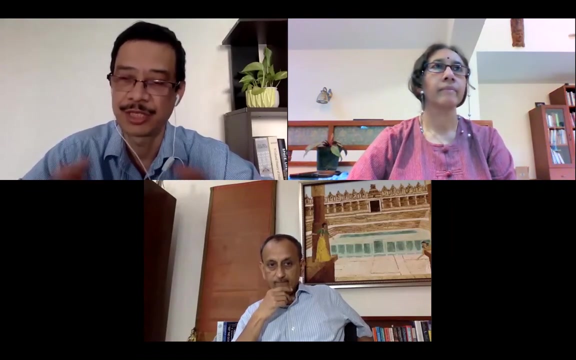 objects that are very, very hot. but radio astronomy is good for objects that you know at all, for all objects, but especially for objects that are very cold. and so when the universe was born, you know, when you, after big bang, uh, in about four hundred thousand years, i think, it became transparent. 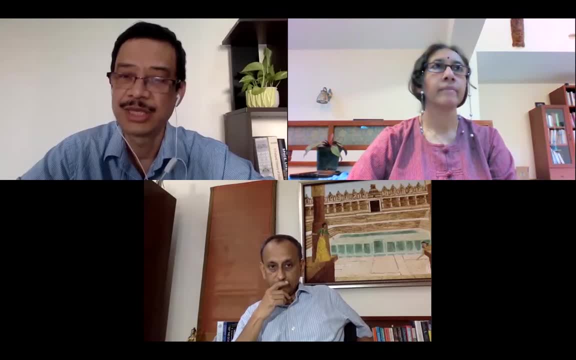 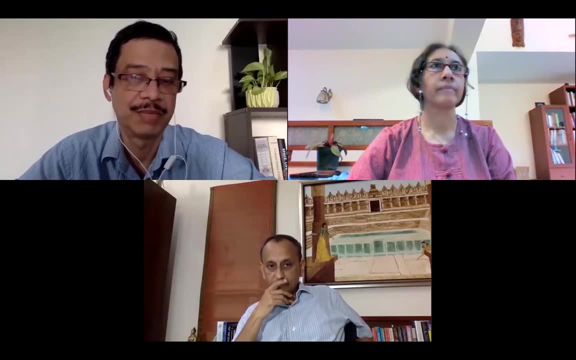 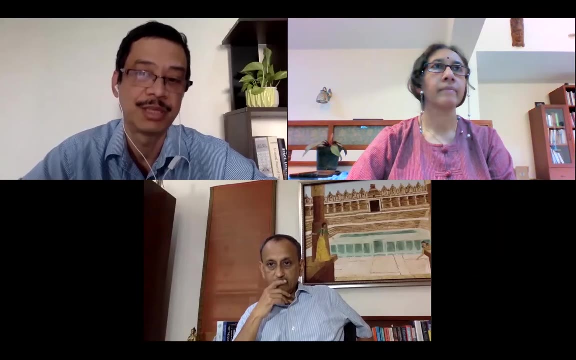 to radio waves. so since then, till the first stars formed, which we don't precisely know, but when that happened, um, maybe 500 million years or 600 million years, sometime in between the birth of the universe till the first billion years, there was not enough light. in fact, there was no light in the beginning. 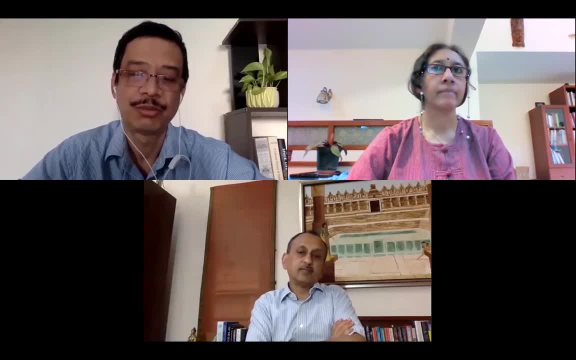 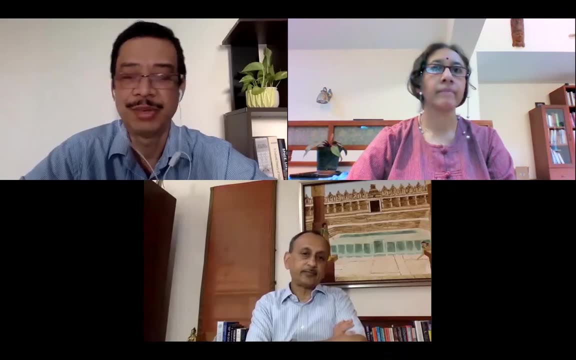 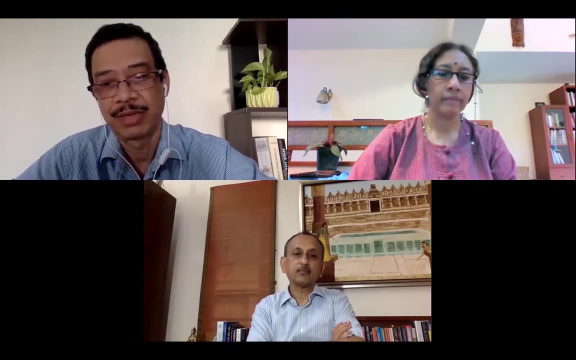 there were only radio waves. so if you want to look back into the universe, uh, early in its evolution you have only radio waves. so one big problem they want to understand is they call as a recombination, so at about 3000, you know, when the temperature dropped to below 3000 degrees centigrade. 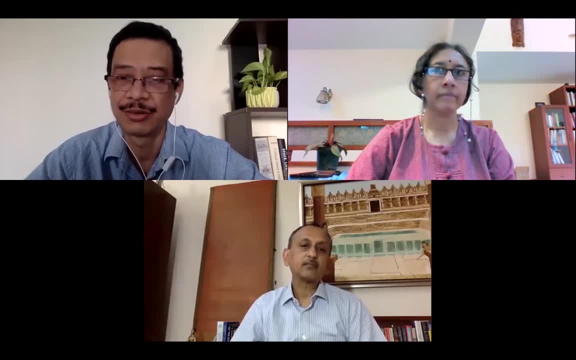 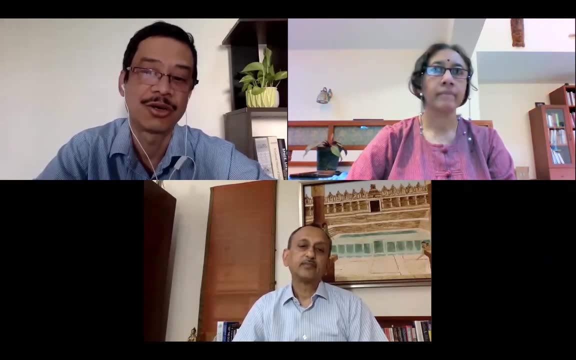 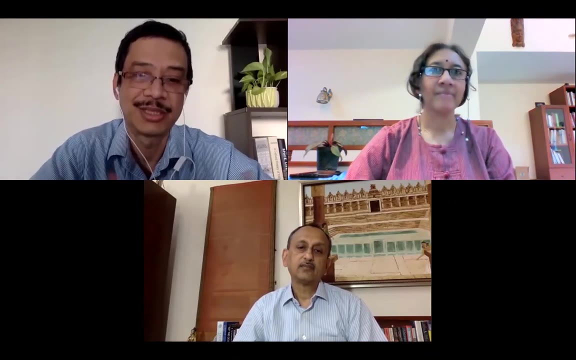 the helium nuclei and hydrogen. the protons came to combine to form hydrogen and and helium. it's this era they call as an era of recombination. i don't know why it's called recombination, because it was only the first combination, but it's called recombination. so we don't know how, when precisely, this happened. 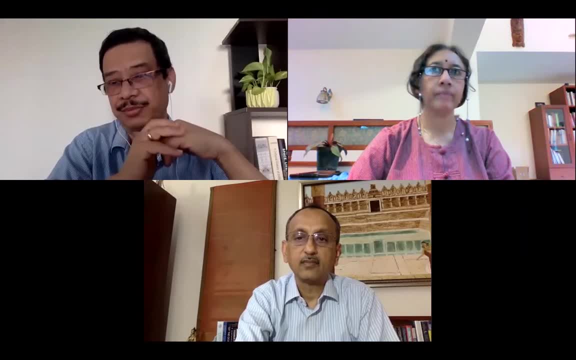 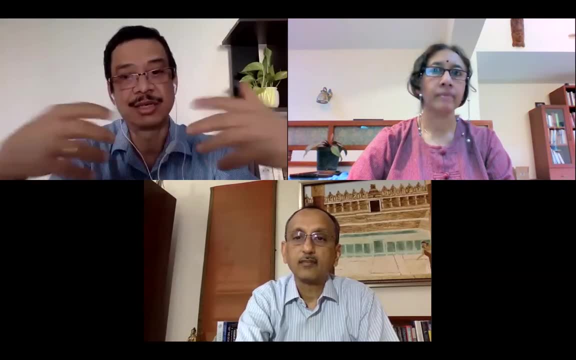 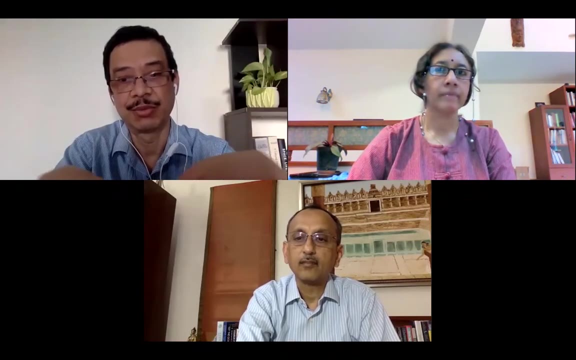 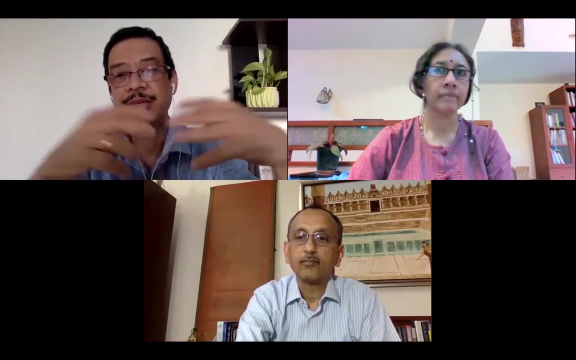 so getting signals of recombination is a big problem in radio astronomy. so, similarly, when the stars formed and they began to radiate light and ultra well, you know, because of this radiation the gas became re-ionized, they once again become um, you know, the electrons were stripped off of the hydrogen atoms and hydrogen became a lot of hydrogen became. 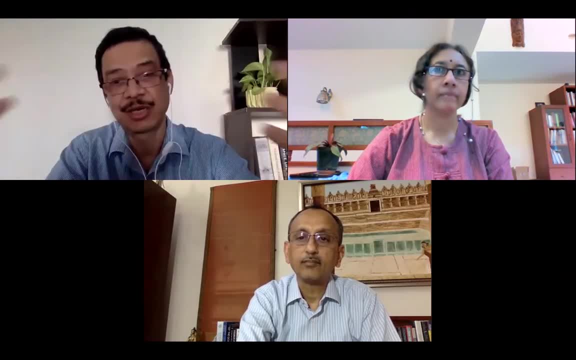 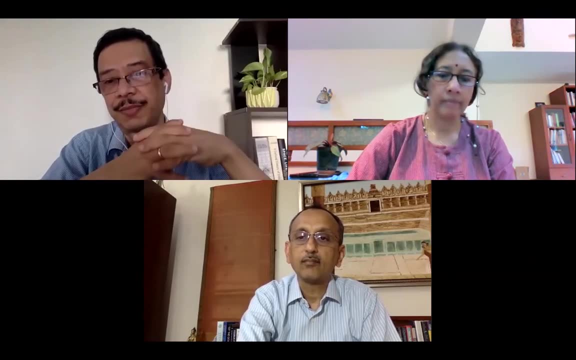 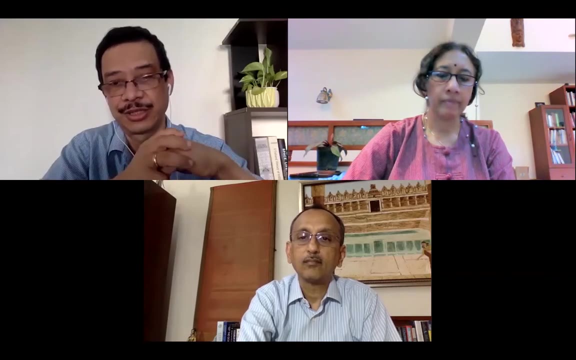 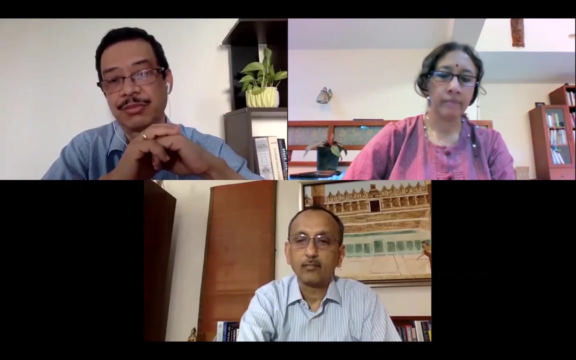 ionized hydrogen. finding evidence for re-ionization is also a big problem and you can use radio astronomy for many other things, for pulsars, um. because of this you know the other thing, the synchrotron radiation, which happens when electrons spiral around a magnetic field. it gives a lot of information because there are most of the hydrogen is not. 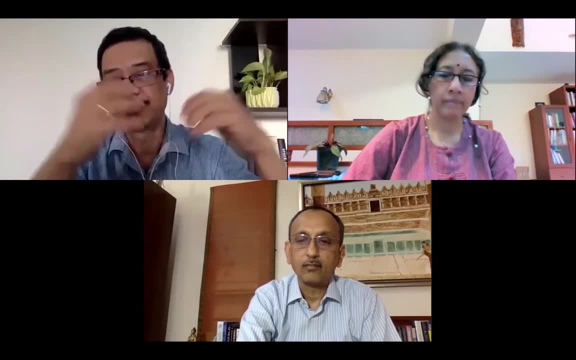 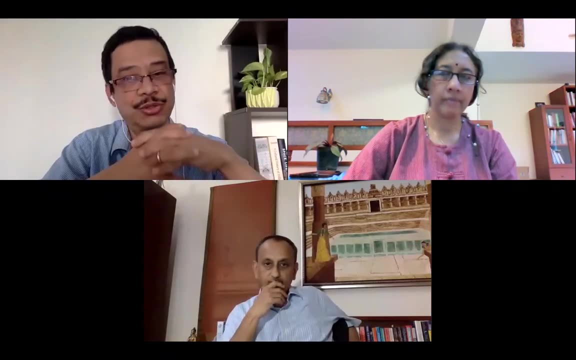 a lot of the hydrogen is ionized and there are lots of magnetic fields, so especially in pulsars, for example, they have intense magnetic fields. so radio waves are a good source of information about pulses in supernova. you can look backward after an event has happened- 10 000 years backward- using radio waves, which is not what you can't do with optical waves, and 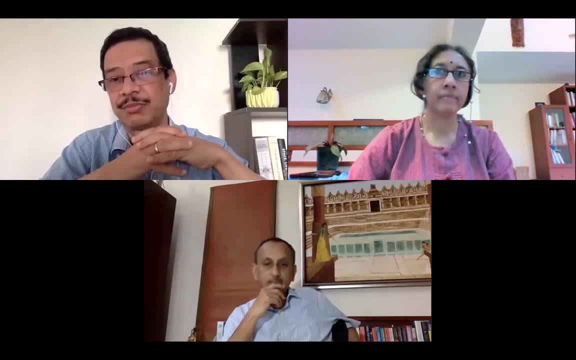 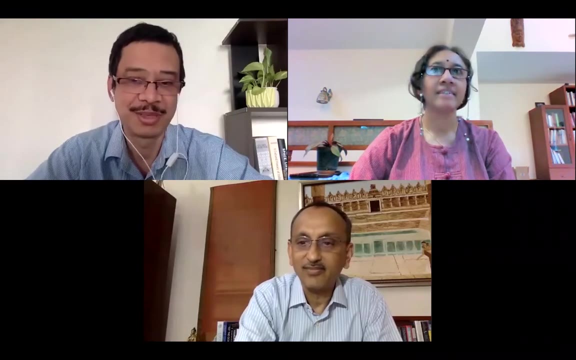 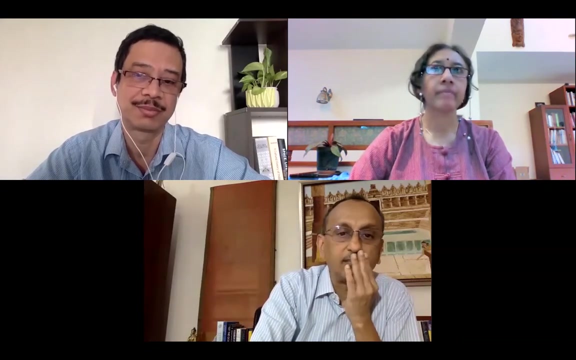 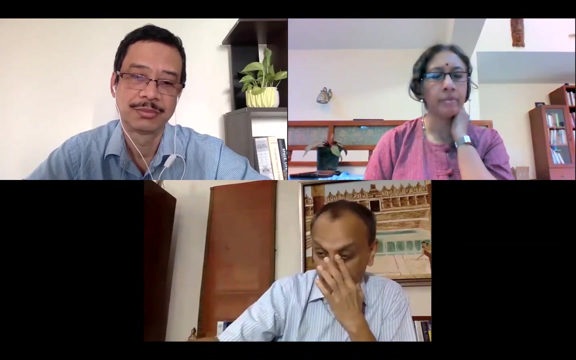 then many other big problems. uh, radio waves are important. thank you, um, someone wants to know: will the lego india come online sometime soon? no, it will come online, i suppose, but it will take a lot of time, probably 27, 28.. around that time let's come back a bit to what you were talking about earlier, about. 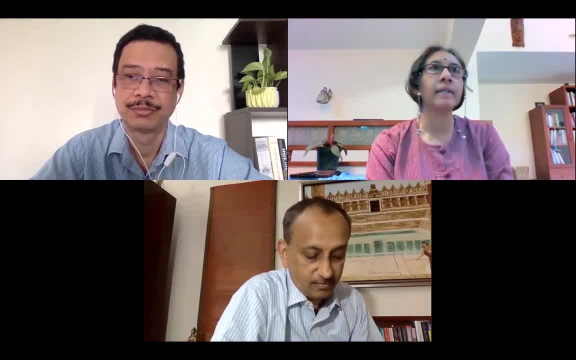 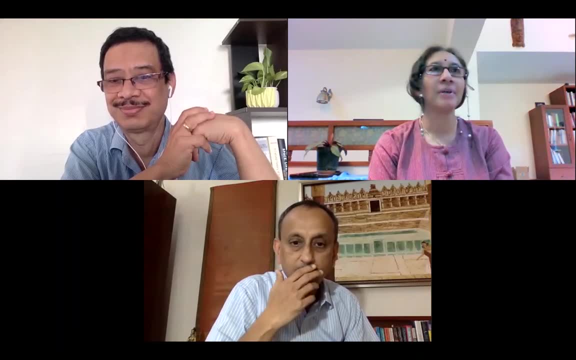 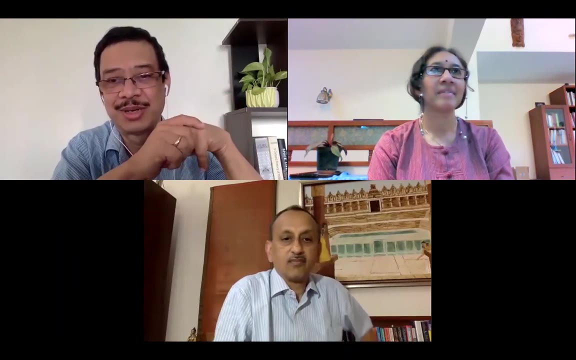 you know the importance of science a little bit about that. you've won an award for the popularization of science. can you tell us a little bit more about what, what you did and what can be done? what's your story? well, popularization of science is a word i'm not sure i like very much. 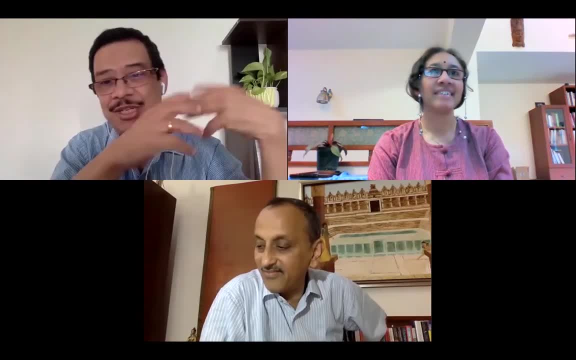 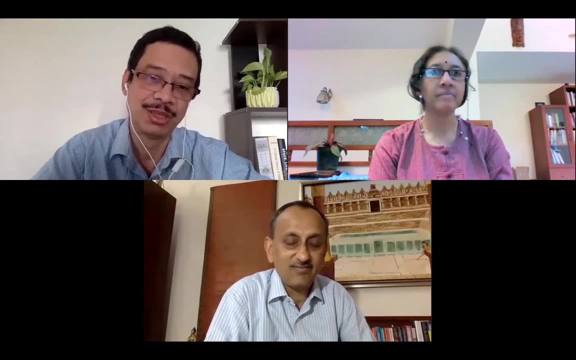 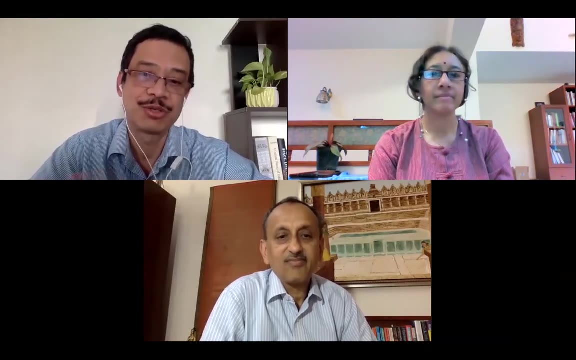 because, um, i was telling stories and it so happened they were in science. i was a journalist, i was. my aim was not to educate public about science, you know, in the way science popularized is usually taken to be. my aim was to tell people about what's happening in the world of science and technology. 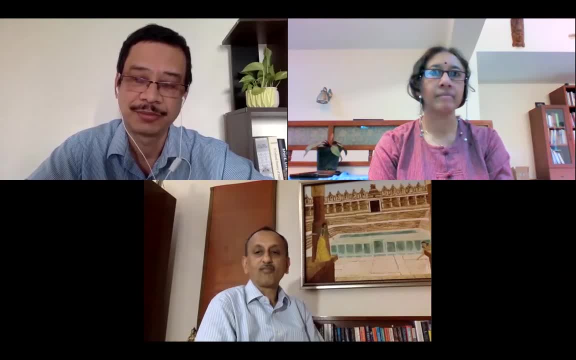 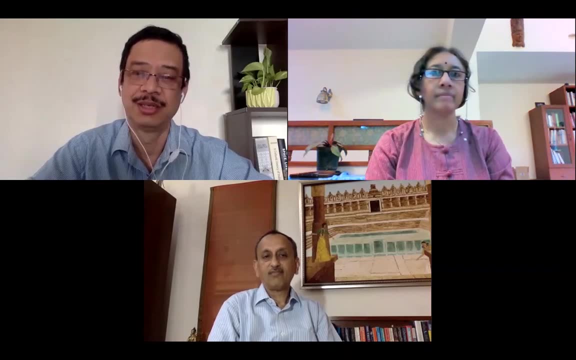 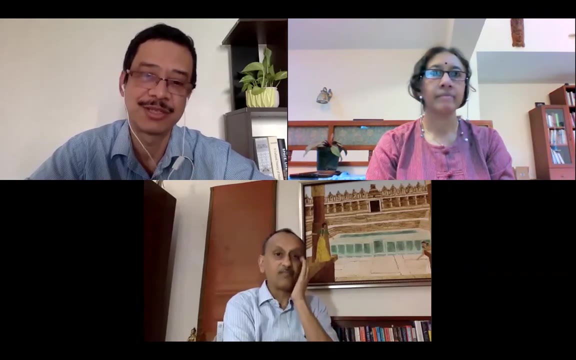 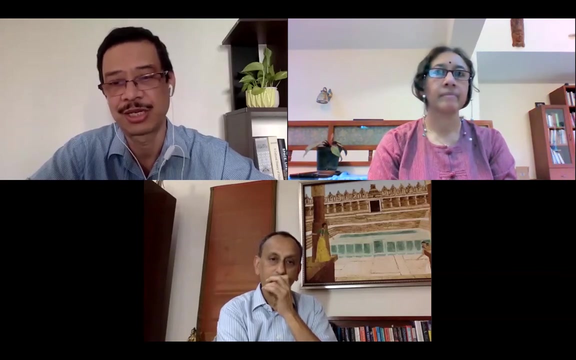 at that time and i worked in business news publications all my life in business world, first of all about 18 years, and then economic times for another seven years. so because of this accident, most of what i did was about private industry and not so much about fundamental science. i did write about science. 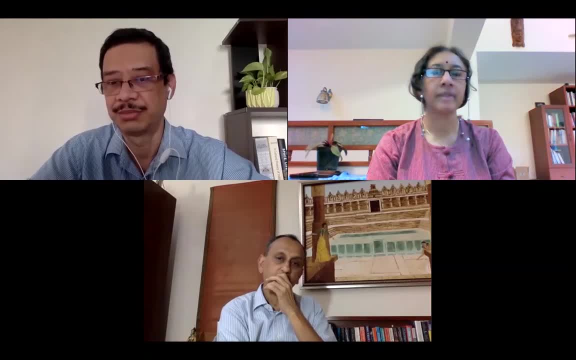 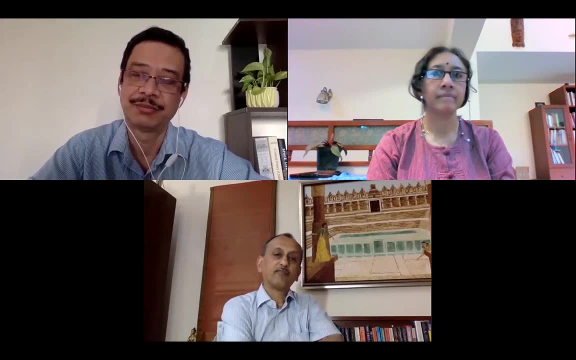 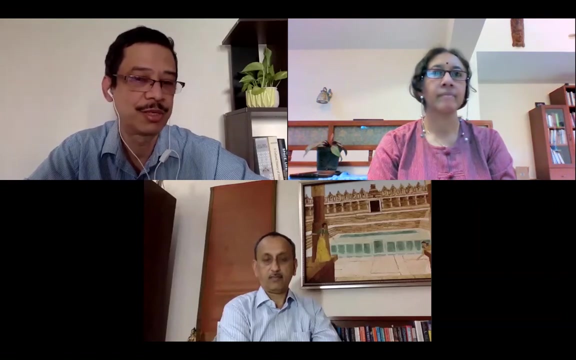 sometimes whenever something big happened like a higgs boson or a gravitational wave and other things in health. but mostly i was interested in what private industry did, about r? d, about the biotech industry, about the pharma industry, about a little bit about it industry. but i also wrote about space, not so much about astronomy but about the space program. 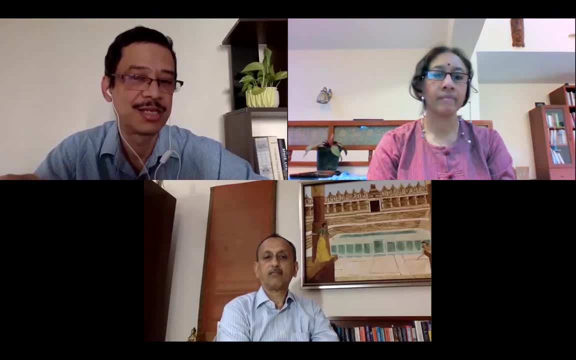 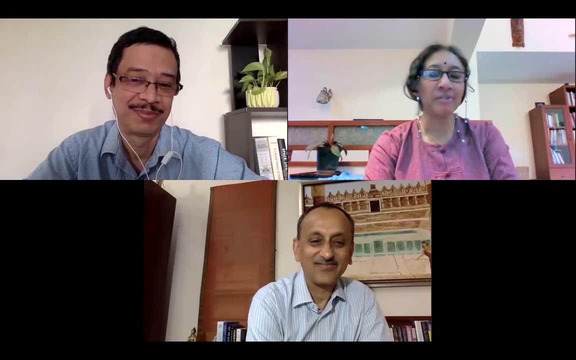 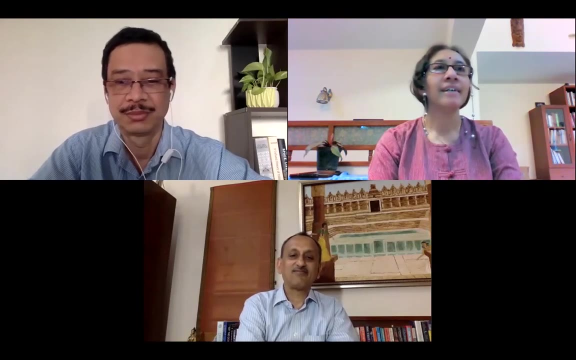 so. so i was not trying to popularize science. it is a side effect rather than in my main aim. so, um, you know, in terms of um how premier educational institutions like the ied is, which is really the uh group of institutes that we've kind, we've come together as alumni of 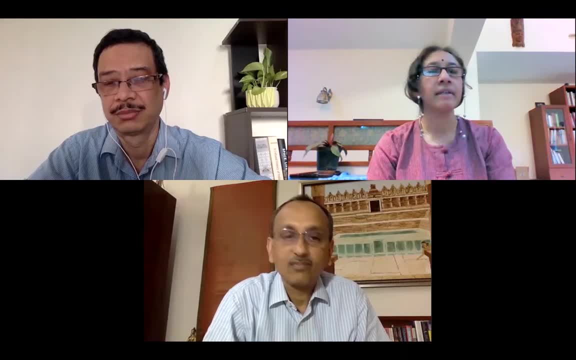 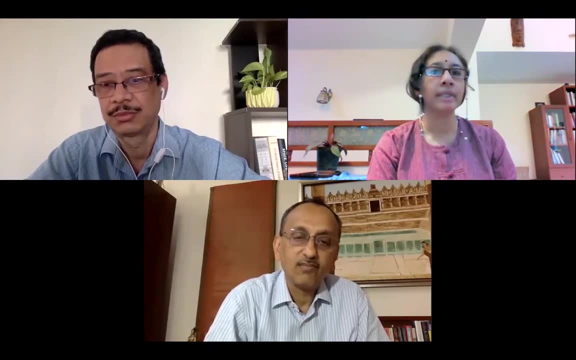 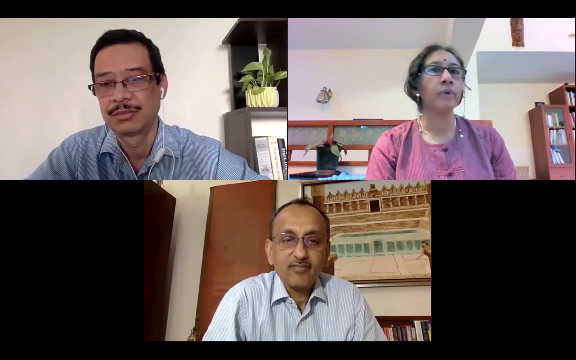 what can they do more to further science? and you know you talked about what happened when these grades of science, uh, set their mind to it and said science is important for this country, and indeed it is, and you talked a lot about all of that. how can we take it forward? what are some of your thoughts and what have you thought about it? 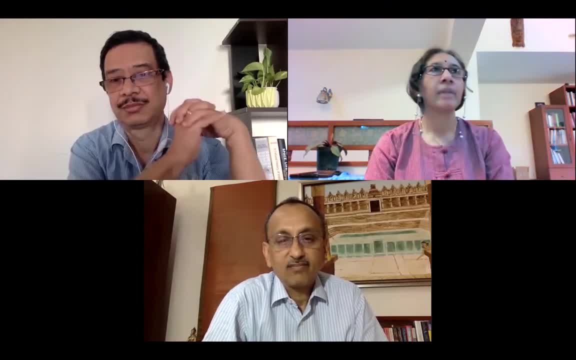 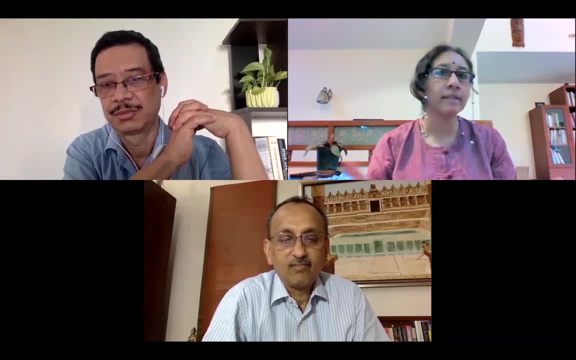 you know, what would you like to suggest? and and when you say science, now we're talking about, like you rightly said, uh, it's. you can't take out science and technology and separate them out. it's, it's all kind of together. so when you put it like that, what can? what are the directions? 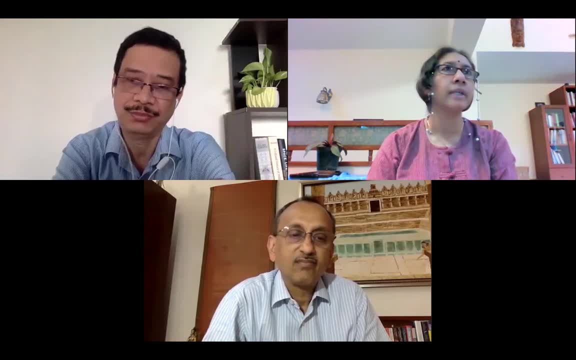 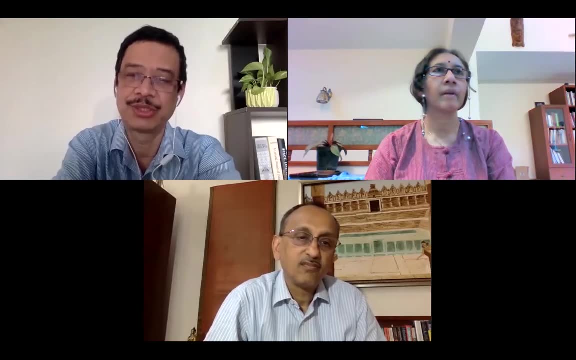 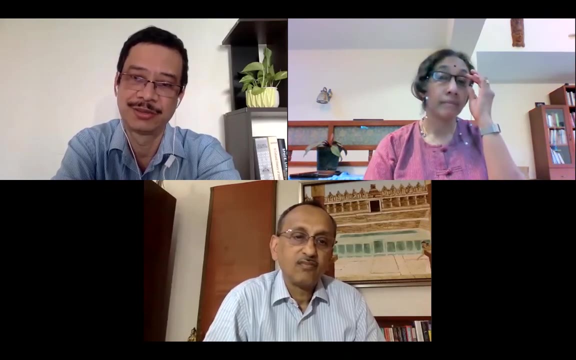 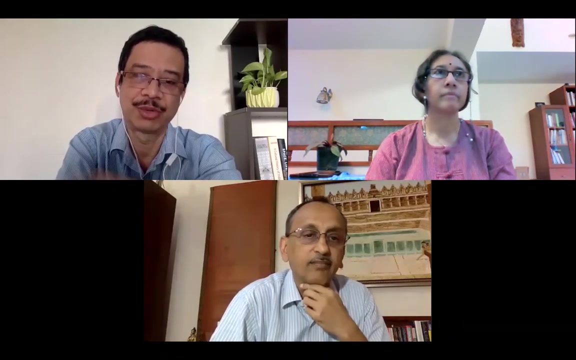 what are some of the actions that these institutes should be taking? so most of the institutions i i think doing the right thing, because indian institutions have changed a lot in the last 20 years and the IITs themselves have become very, very prominent into such, which was not the case earlier. you know, if you look at the output from indian 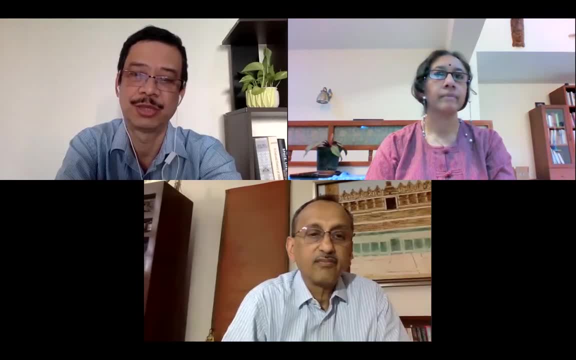 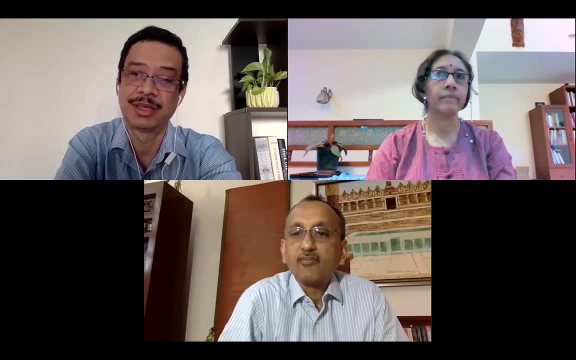 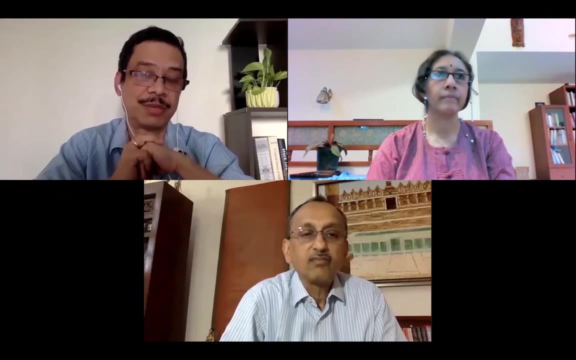 scientific institution in the last 15 to 20 years. IITs have dominated in the last, especially in the last decade. That is because engineering and engineering as a subject itself has become important in research now, because there are a lot of publications and that is overall. 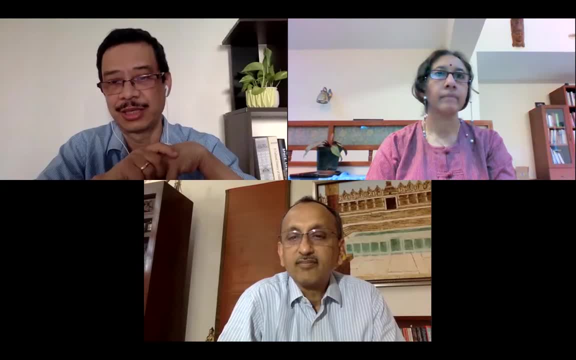 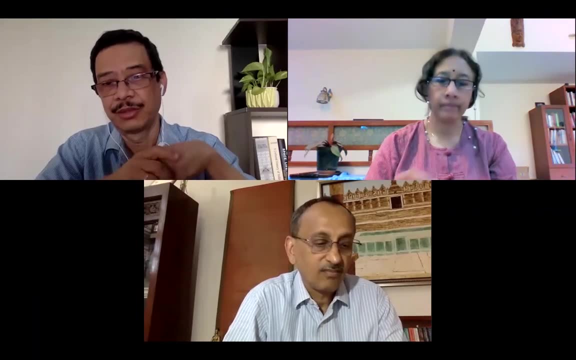 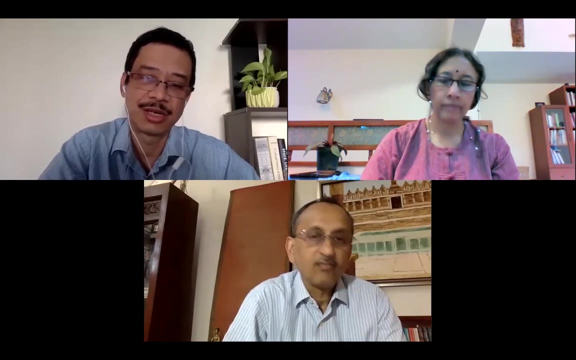 good because you know you can have the synergy between science and engineering. What has actually declined is this tradition of building equipment. So all this equipment that people build, not just two radio telescopes now, Sienna Rao built a lot of a equipment. you. 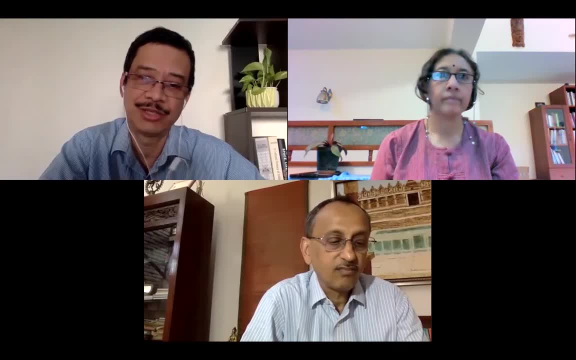 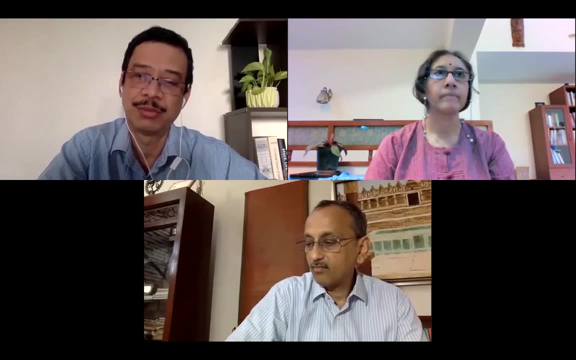 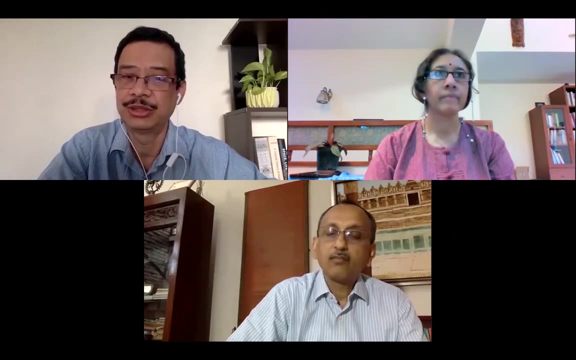 know we're using very, very, very ingenious methods. I mean methods means, not specific methodology. they found a way to build equipment that they wanted with very little money and using a spare parts, So this has been a tradition, not- and I have already mentioned one person. 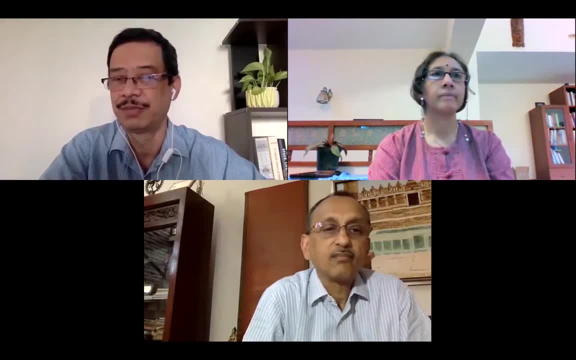 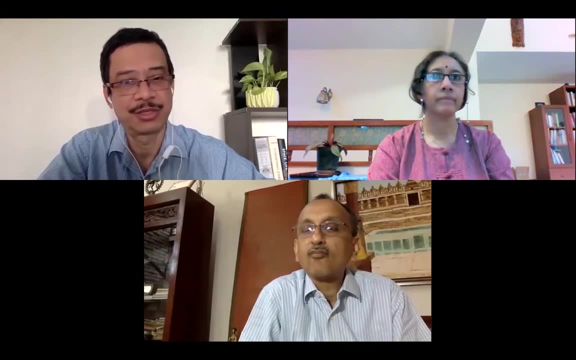 Sienna Rao, Im치, lightants, vierouts科学, 007. people in the 60s and 70s built a lot of equipment At a time when there was not much support. there was no private industry. you can't get components that easily. 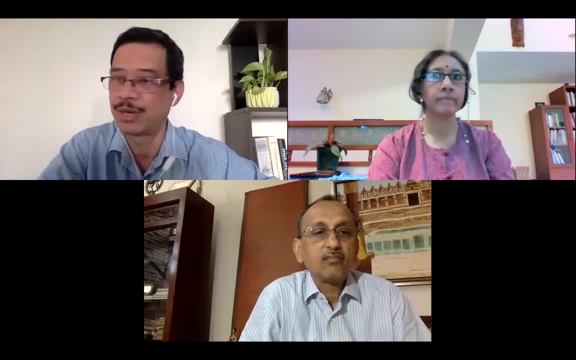 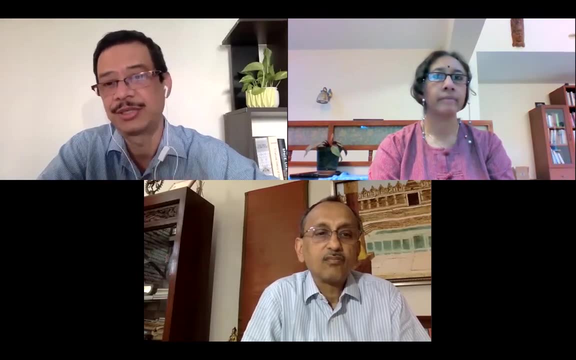 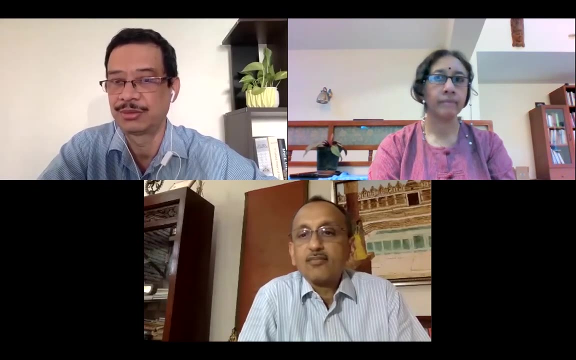 But now that tradition has sort of declined And I don't know why. I mean, I have not investigated too much. Probably it is impossible. People tend to buy equipment off the shelf. but scientific instrumentation is still alive around the world. An example is this cryo electron microscope. 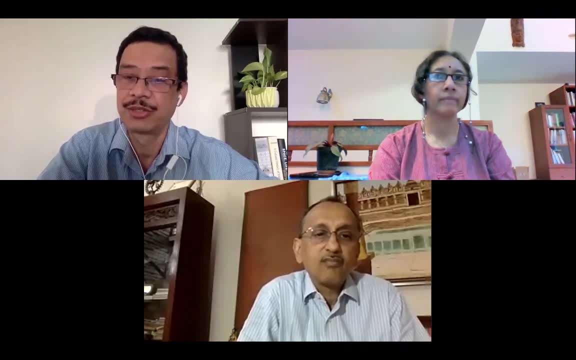 which was built in Cambridge over 15 years of work. So it is important for India to build equipment in the frontiers, And there is some support from private industry. now We have capabilities and this is the time to build equipment, And that is one thing that is missing. 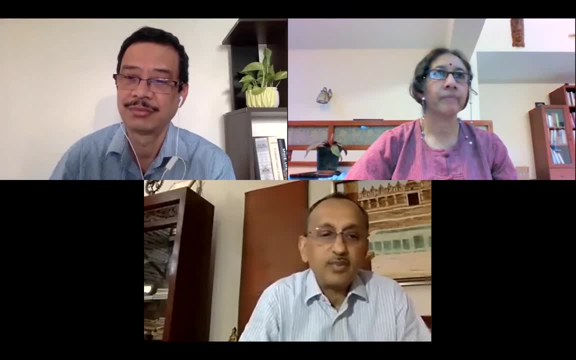 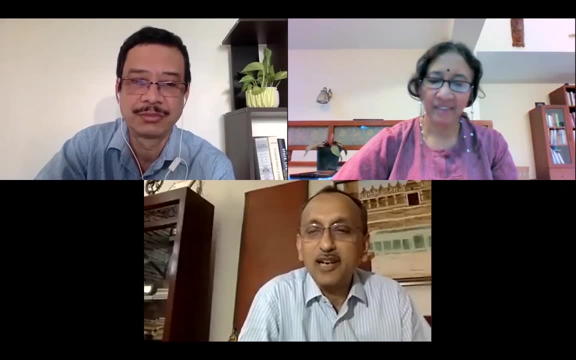 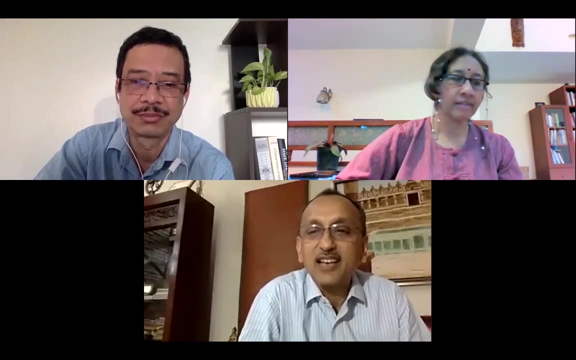 Thank you, Ashok. would you like to? You need to unmute, Ashok. So, going into the realm of a little bit of speculation, there's a question here which says: will Musk's Starlink fleet likely interfere with radio telescopes? 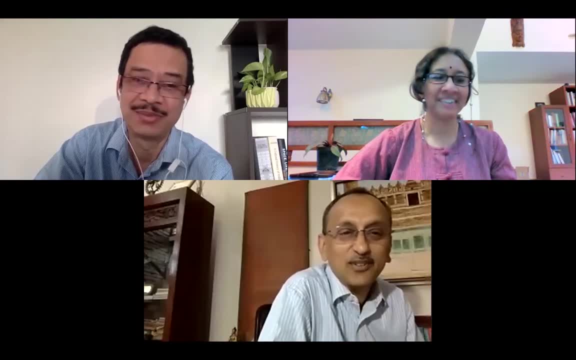 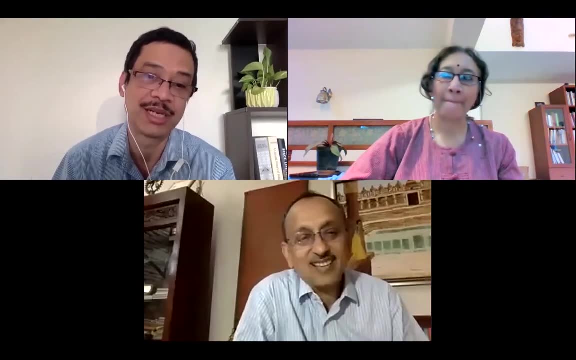 What is your take? I have no idea. This guy is going to put up some 10,000 of those little satellites. So a lot of things interfere with radio telescopes now, And mobile phones too. The biggest problem is. the biggest problem is mobile phone. And sometimes TV broadcast too. But I think that they are aware of that. Radio astronomers have figured out ways to counter those. You know they're very clever, They know how to get data from that noise, But probably there is a limit to that. Yeah, there will be. yeah, Because I think in the next 10 years you'll probably see 50,000 little satellites up there, you know, between all these guys wanting to offer you space based internet services. So It depends on what frequency they use. 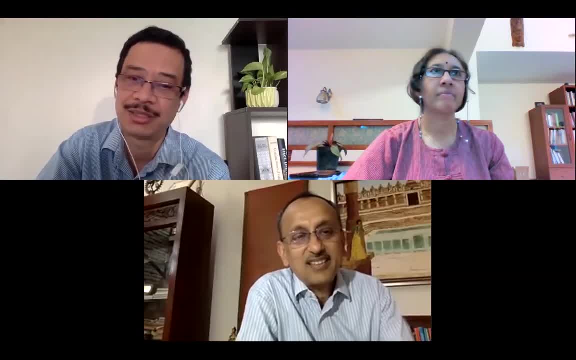 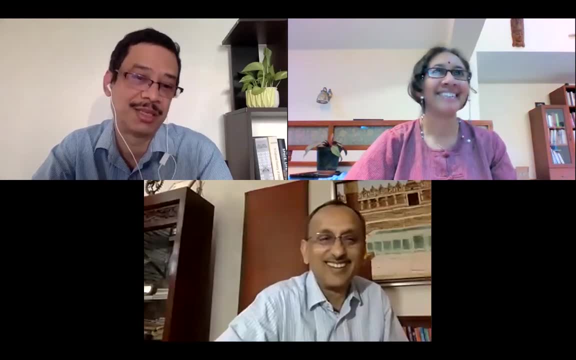 Yeah, that's true, Other frequencies will be, But there is a lot of noise even in otherwise And a lot of junk. Yeah, in Kodad, where they, which was a sort of a pristine place from a radio, noise free. 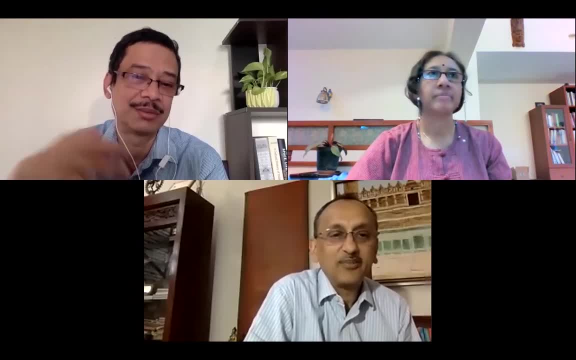 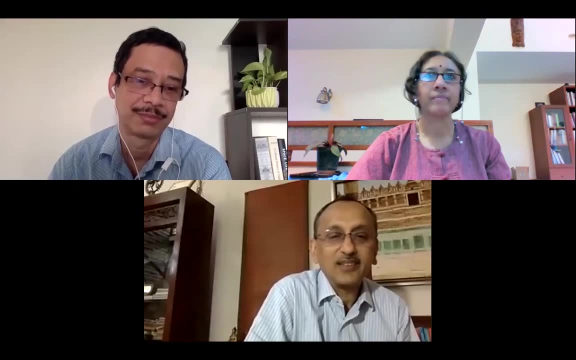 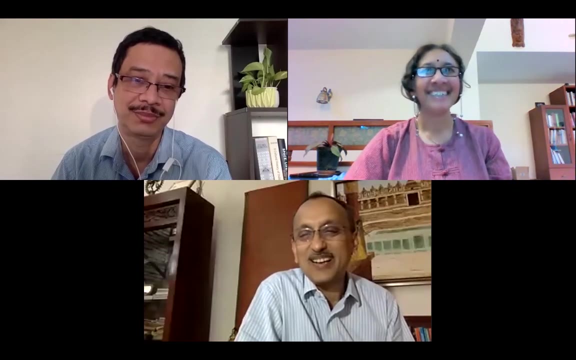 Now there is a lot of radio noise, but the techniques have their techniques have also improved, know how to handle noise that much better now. so we'll have to actually figure out the signal in the noise. so yeah, um, so radio waves are so so feeble, it's unbelievably feeble, you know, if you 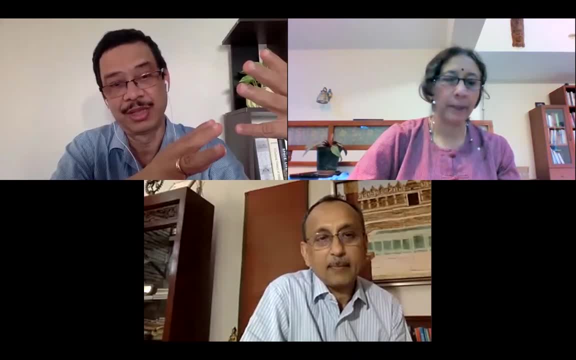 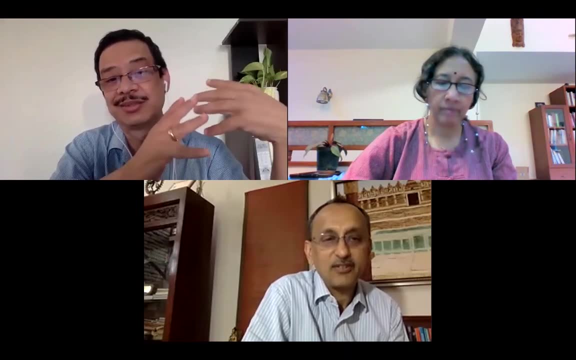 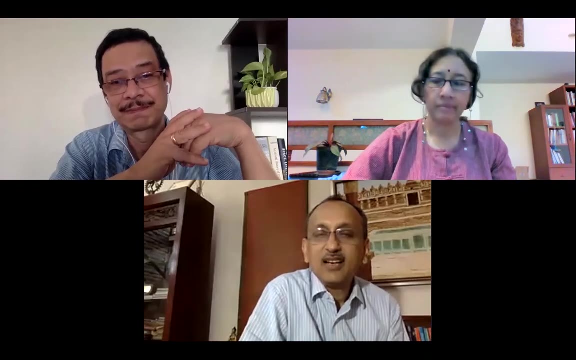 put a mobile phone on the moon, the signal from that mobile phone would be stronger than from a radio object, an object in the universe. they are that weak, sort of a billion billion times weaker than a mobile phone signal. yeah, uh, this, uh, also i think. uh, you know one of the questions. 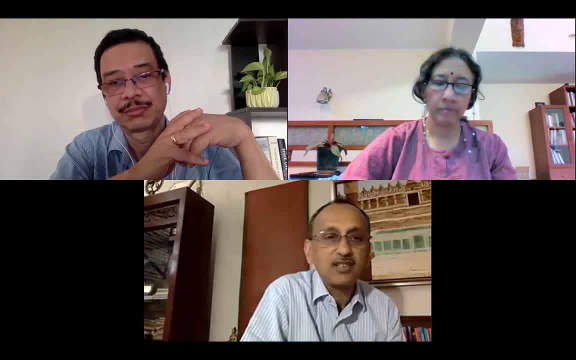 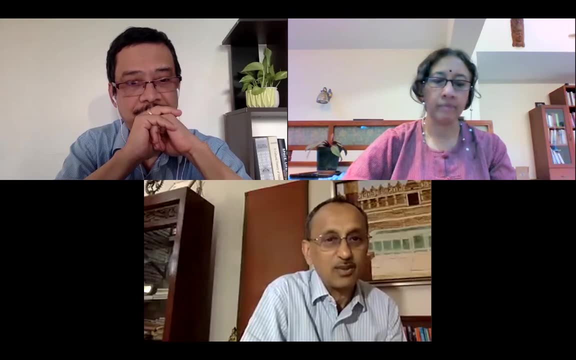 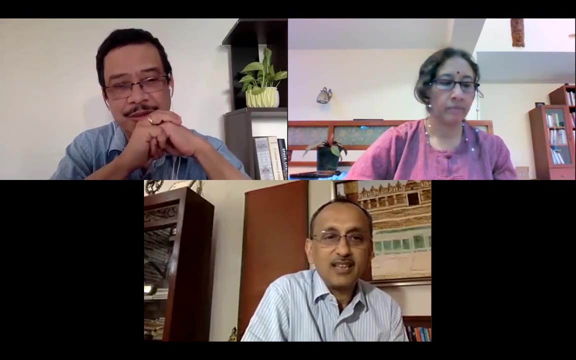 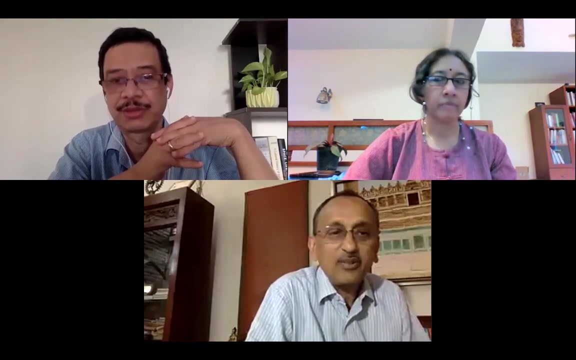 here that there's a big telescope being built in mauritius. uh, and i think the it is built with the help of indian scientists. are you familiar with that? no, i'm not. yeah, all right, is it south africa? is sk as part of that, there should supposed to be in south africa? south africa, yeah. what is the silicon? 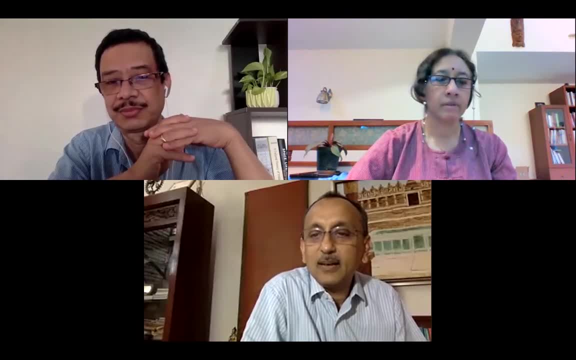 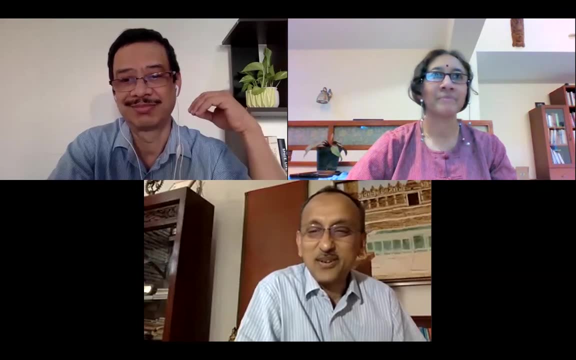 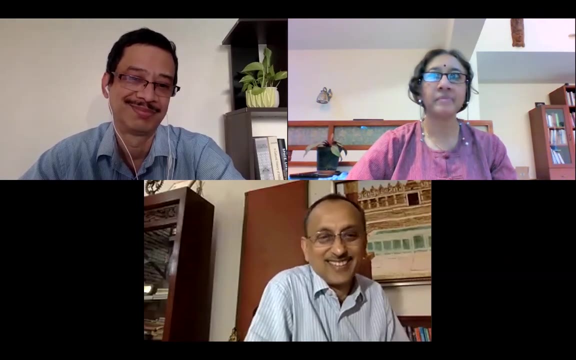 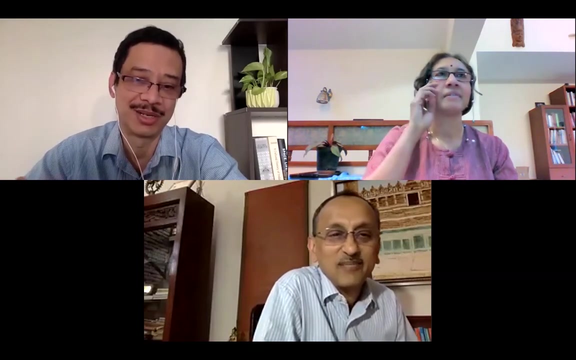 i'm not. yeah, uh, last, i think. uh, you know, and this guy is an anonymous attendee, okay, so he says: has politics in the scientific community decrease, increased or remained the same in the last one century? i think one century is a bit too far. i mean um, because when you say politics, what, what, what do we mean? no, people are. people remain the same. 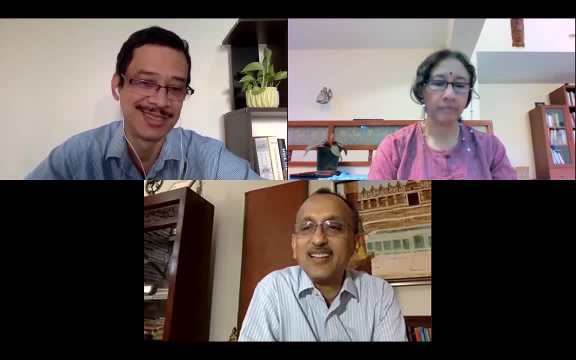 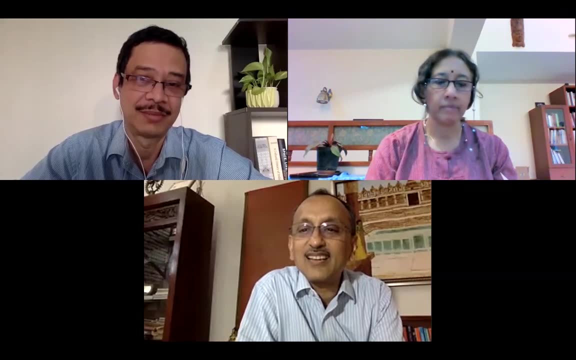 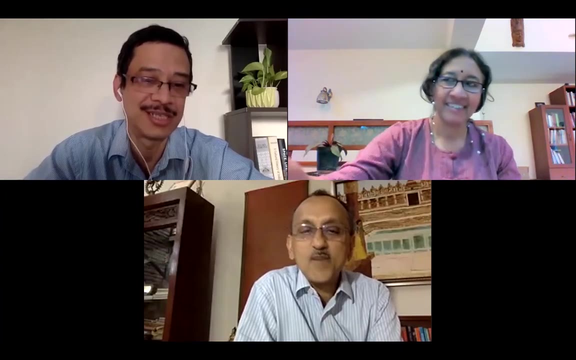 right, people's, people have ambitions, people have jealousies, um. so human beings have not changed the character in the last hundred years? has not changed in your opinion? no, human beings have not changed their character. so there are, there are ambitions. there are jealousies involved, um, okay. 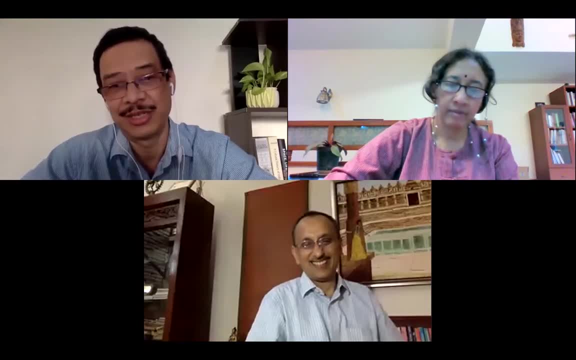 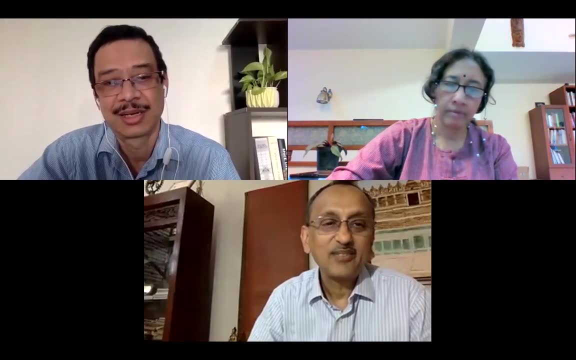 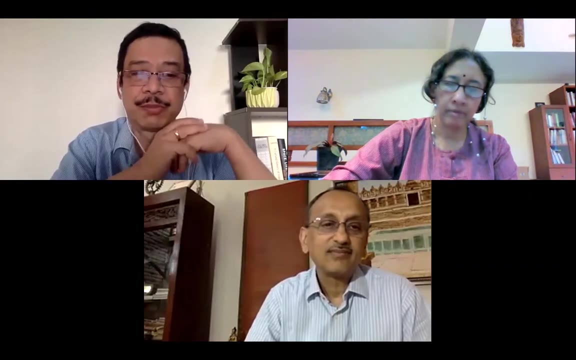 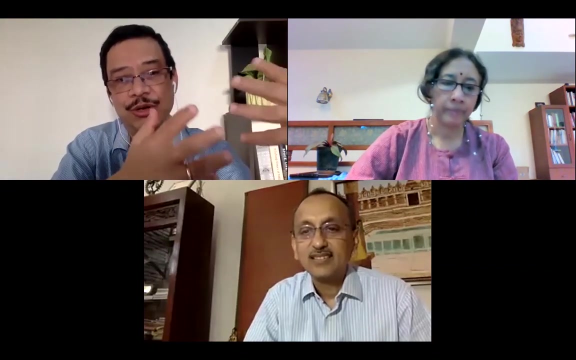 some amount of politics in every some amount of politics in every institution, in every company. so i don't think, you know, scientific institutions are also free from that, but largely this situation that now is politics from a different uh level. you know this idea that what india should do, what india should not do, uh things that come from ideologies, then i'm not. 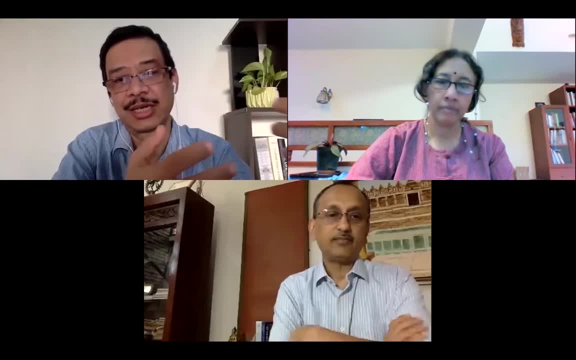 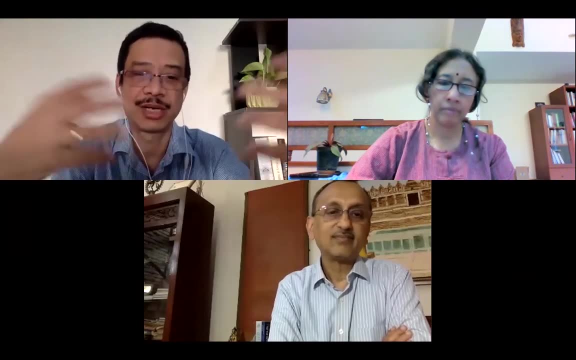 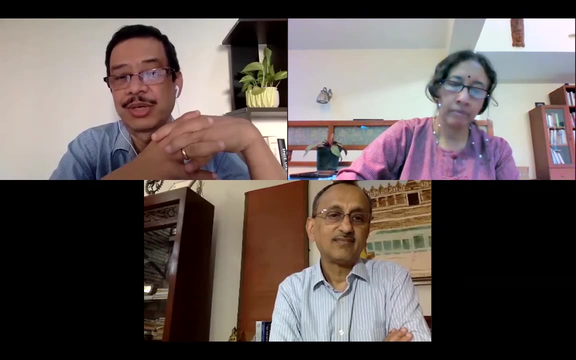 saying for a specific kind of ideology. um, you know the things like these are problems for the, for the, for the common man. so we should work, do such problems more than you know. high science, um, so those that sort of ideas is a bit uh, that that has more impact on what the future of inconscience than then you know small politics. 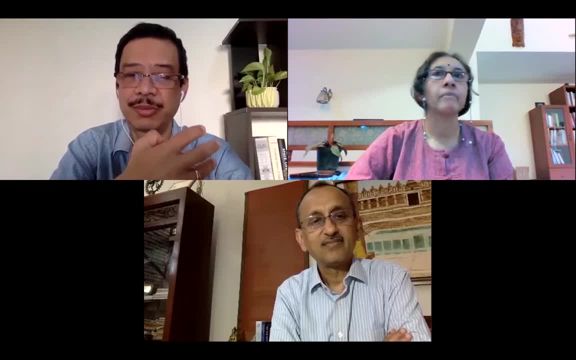 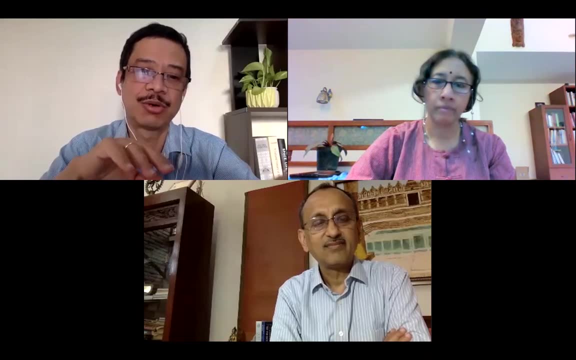 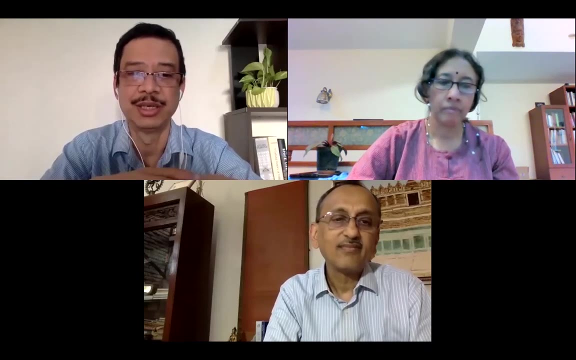 so that is sort of an ideology ideology- and this is not probably a political ideology- to separate science into what is necessary for a poor country and what is what a rich country can do. i don't see science except separated this way. science is all one uniform thing. either you do. 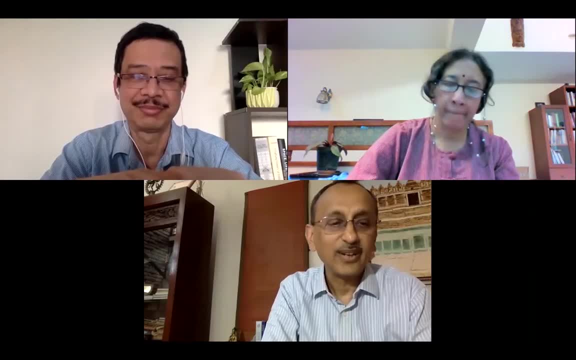 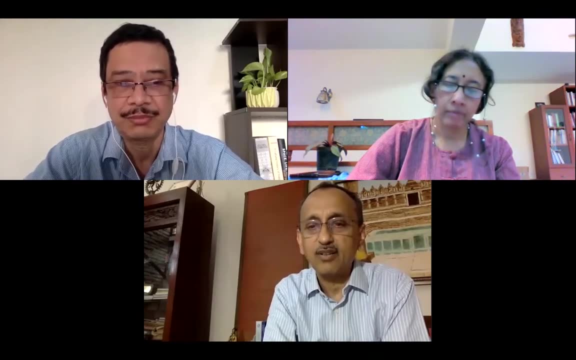 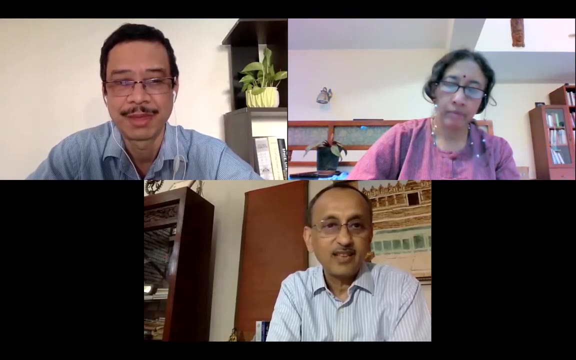 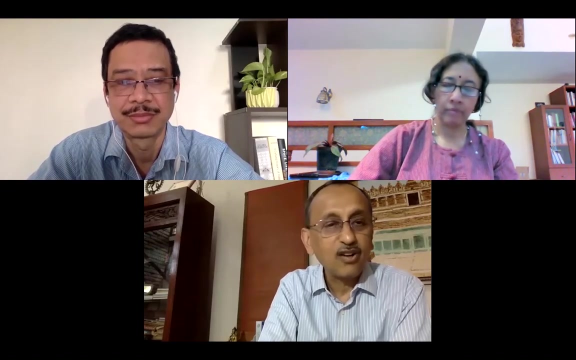 everything or you don't do. do it. uh, this, you might find this a little difficult. uh, you know, professor mishra is asking. signal processing plays a very important role in radio telescopy. do you know who the in your research? would you have met the guys who are the top dogs in this? 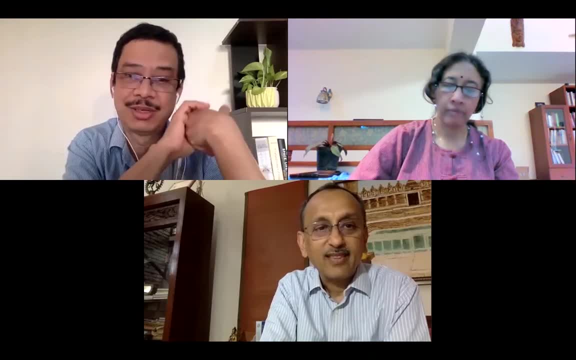 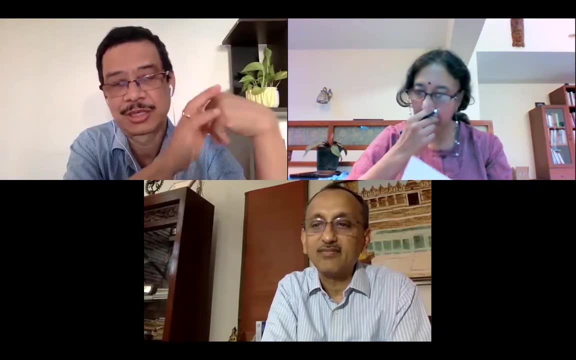 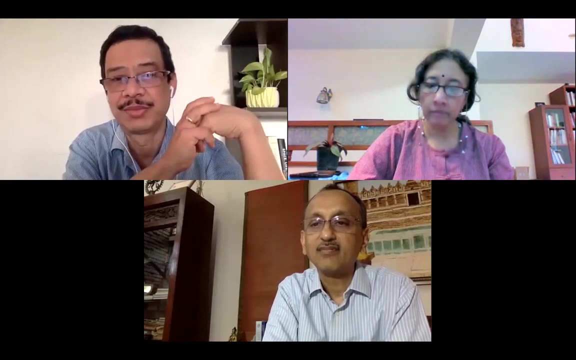 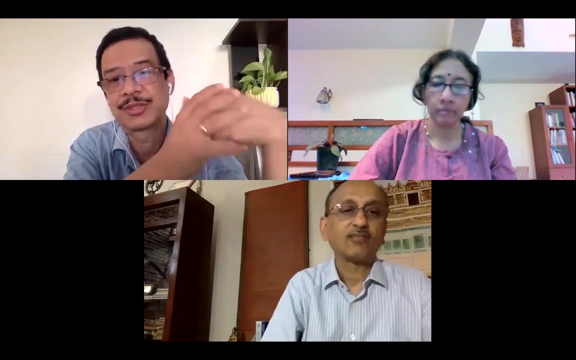 field. well, i don't know um they signal the lot of the electronics for gmrt was led by his current director, dashwan gupta. he has you know who specifically did what. um i don't know, and in siya subramanya was the person and he's now still there. 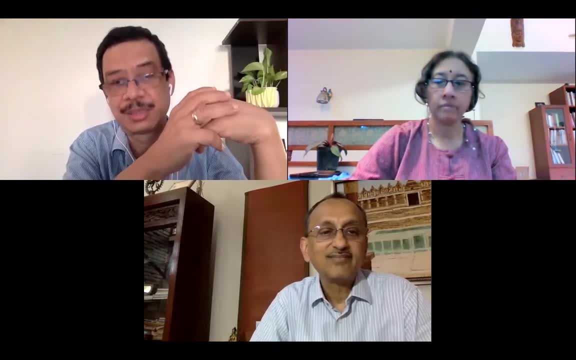 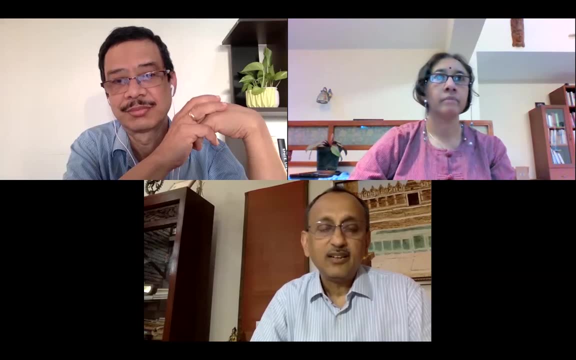 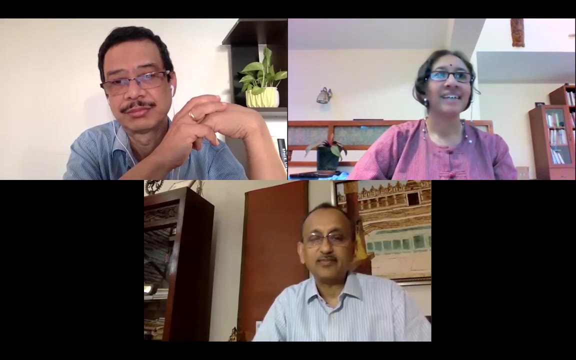 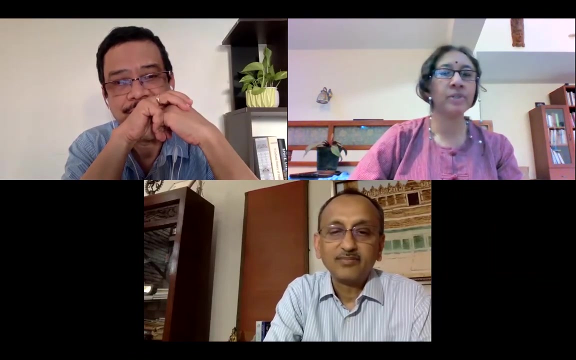 although he's retired and lives away from bangalore, he is involved in this upgrade. all right, so, uh, i think we are done. uh, sushila, do you want to wrap up? sure, thank you, yeah, so we've had uh an absolutely fascinating peep into uh, into into history, into the. 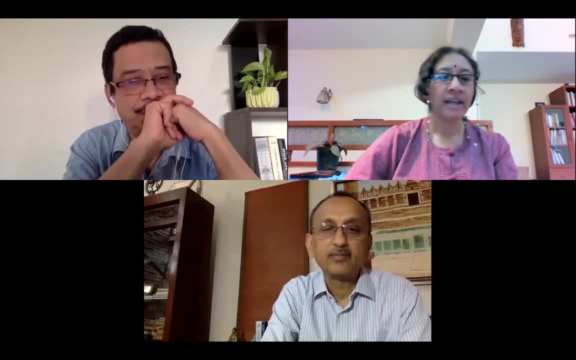 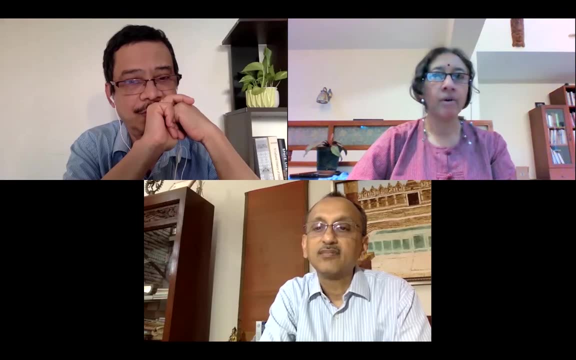 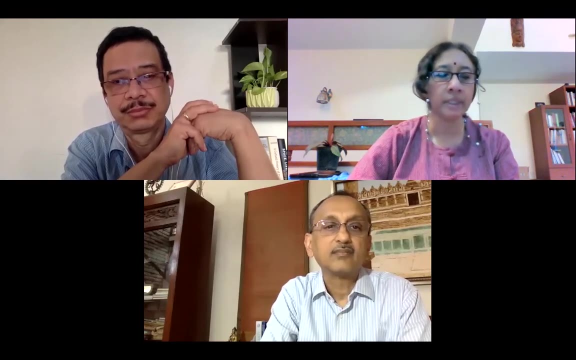 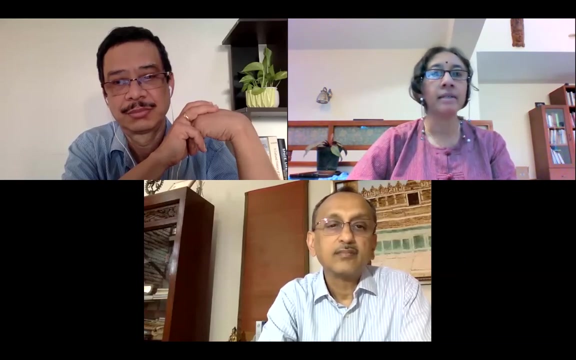 history of science. uh in our country today. uh, you know when? when we got our independence, there had already been an environment of uh science and some wonderful scientists who had achieved a lot, including uh cv ramen saha says vatnagar, homie baba and others. so that's where we started. but 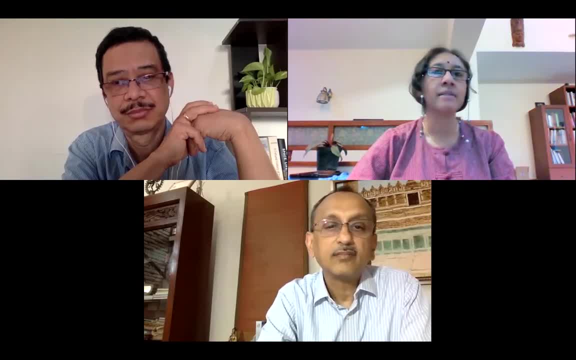 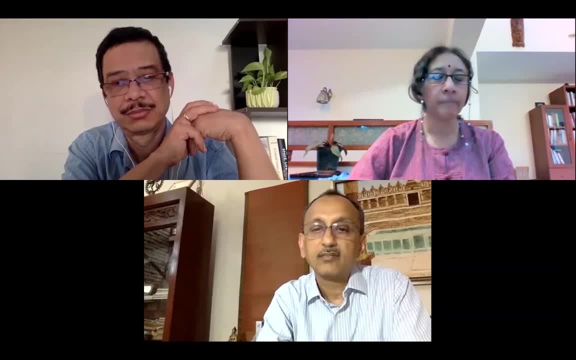 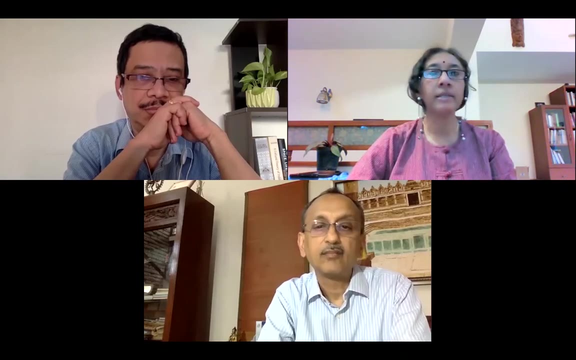 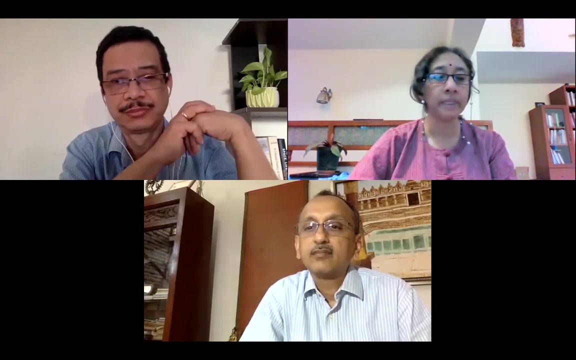 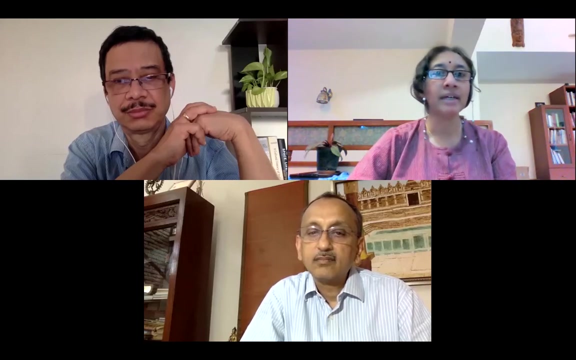 they- all of them- saw the importance of science and the development of science for an independent nation that was getting onto its feet And we looked at today. Hari talked us through the kinds of investments that went into science during that period. So we heard the story of Govind Swaroop. 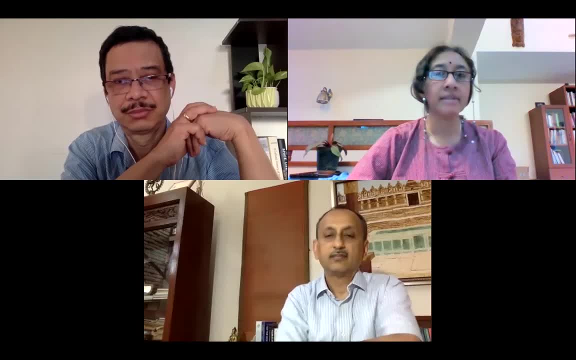 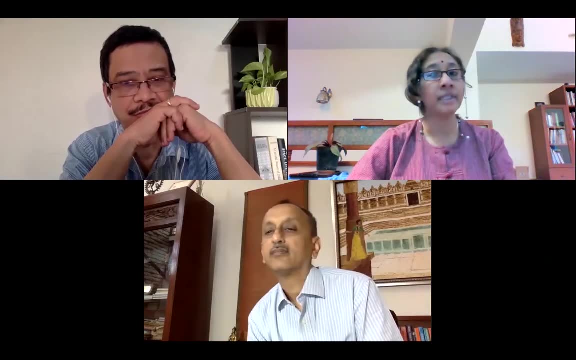 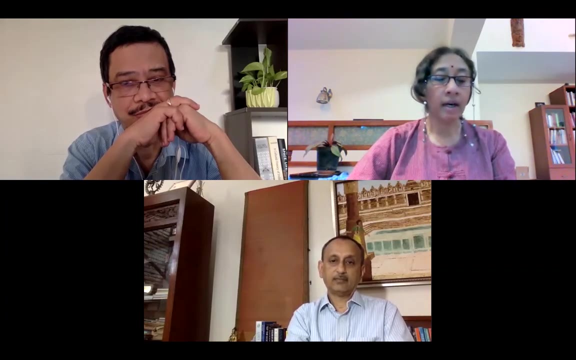 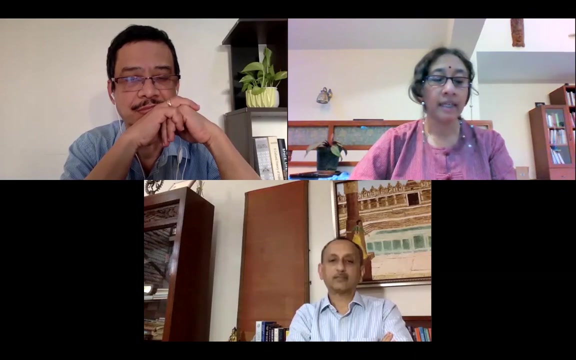 of how, as a scientist who was in the US at Stanford and then came down to join TFR in 1963, how he kind of battled with what do I do with myself and where should I focus, And eventually deciding that what was important for us to do. 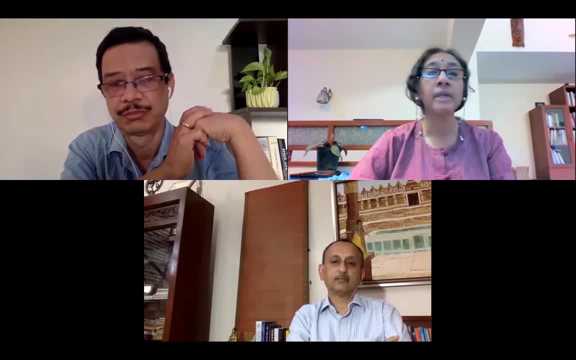 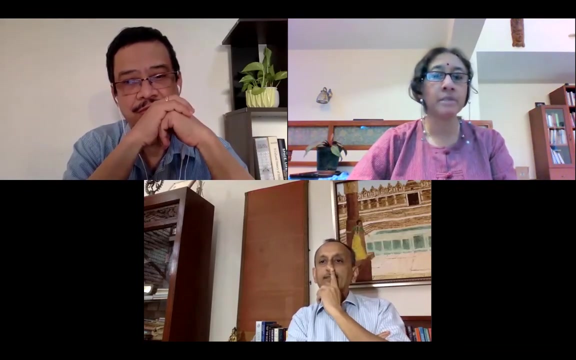 And that astronomy was to build a good radio telescope, because of the need to set up something really impactful, And Hari has also talked us through today about how that step of setting up a completely indigenous radio telescope has been so important, not just from the astronomy point of view. 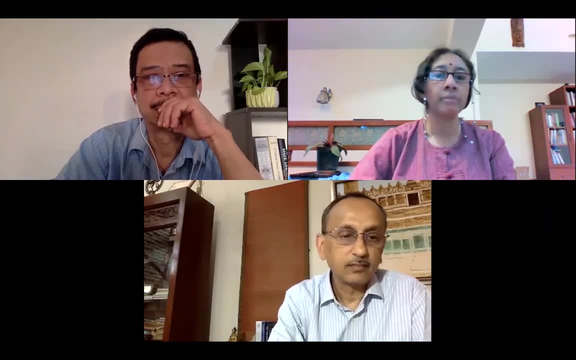 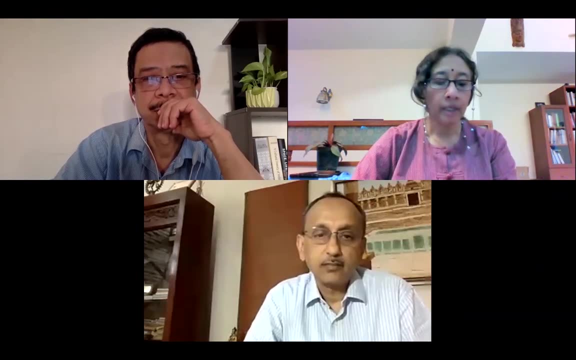 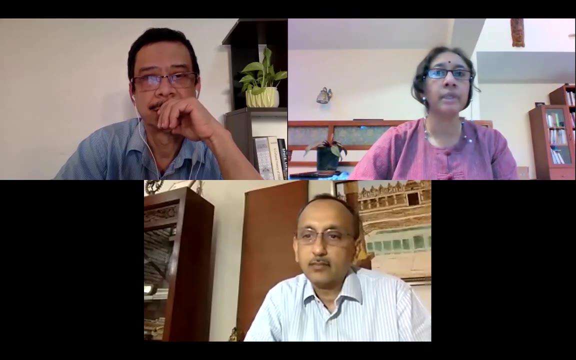 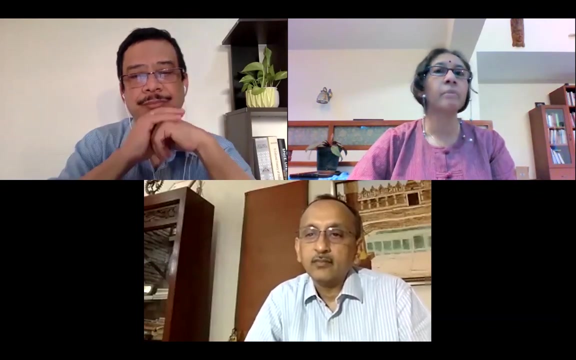 from radio astronomy point of view, but also the development of many other allied pieces of knowledge. And why is this important? Why is radio astronomy important? This helps us. despite the fact that radio waves are so feeble, they're still probably our best source. 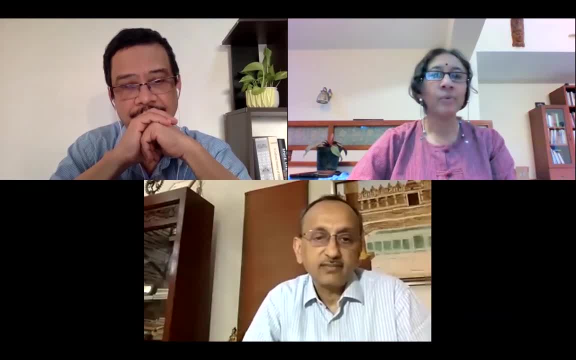 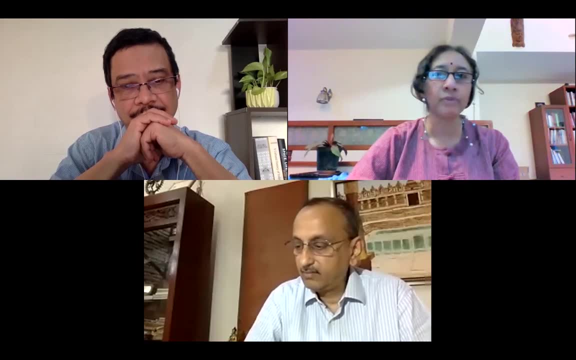 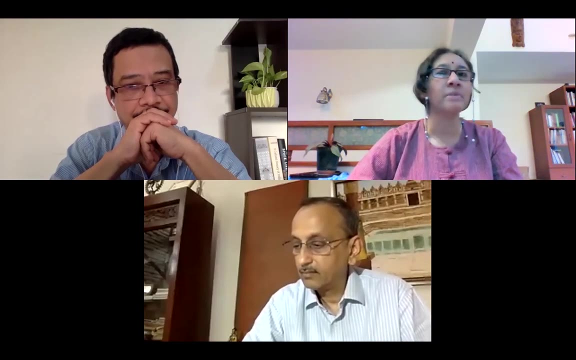 of being able to understand questions like: why is our universe what it is today, How did it come to be- And these are questions that man has searched for for thousands of years- So that- and this is only possible when you have the right kind of radio telescopes. 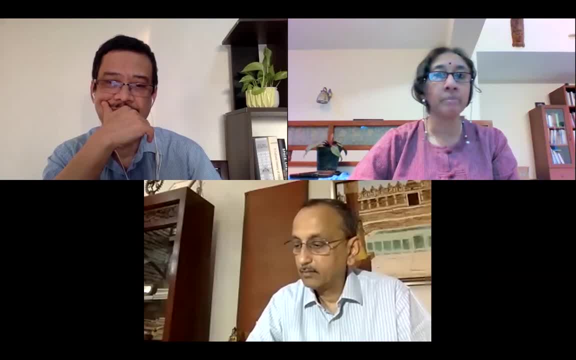 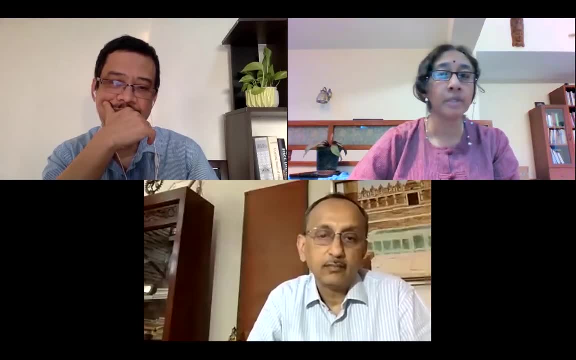 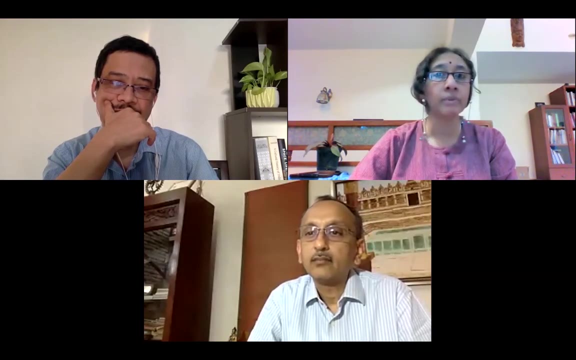 So after Govind Swaroop set up the first, the GMRT, and the GMRT has been used by over 30 countries to help solve various problems, Research problems that they've been involved in, And it's probably one of the best low frequency telescopes. 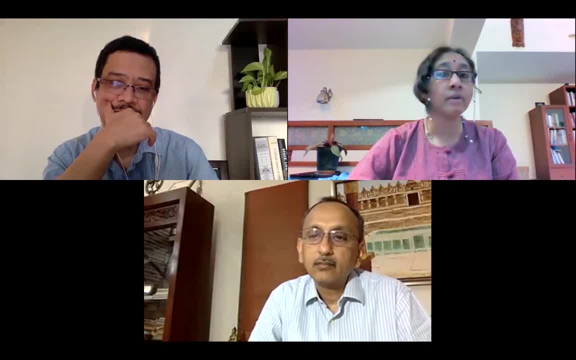 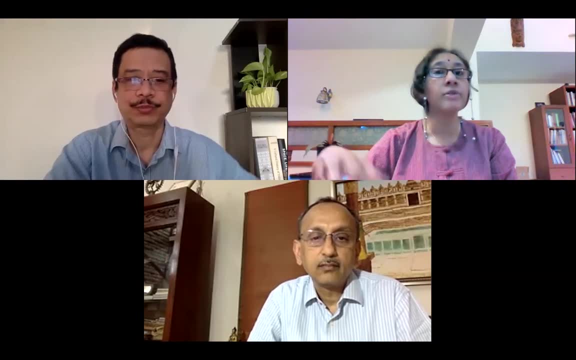 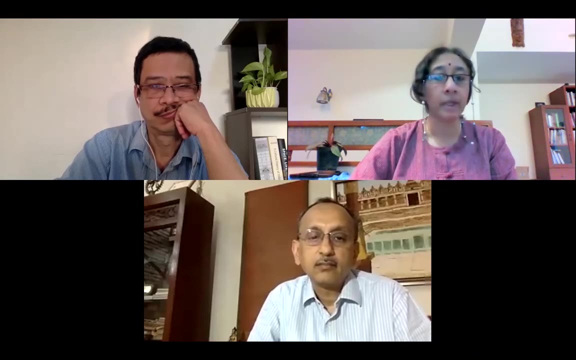 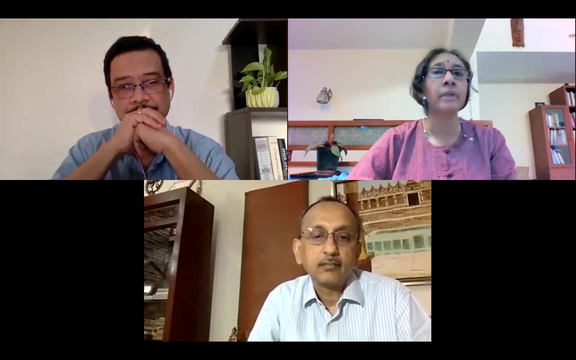 still anywhere in the world. And then he talked to us about the square kilometer array now and India's role in both the concept and the building of that whole equipment. And this is across two parts of the world And it's a wonderful example of what global collaboration. 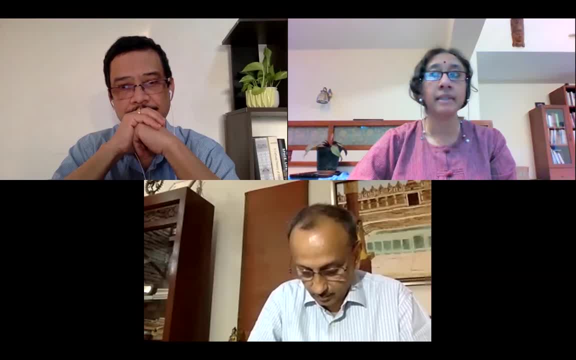 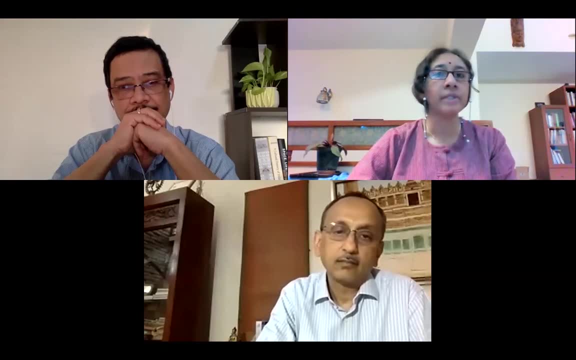 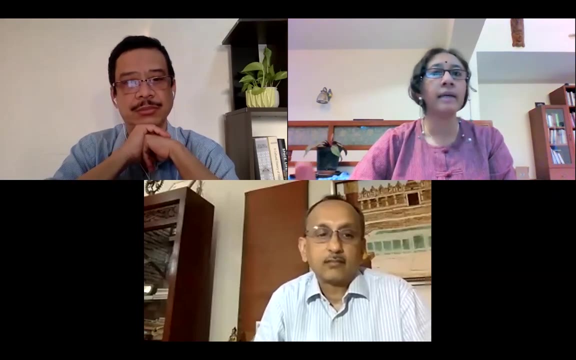 can do So. last year, when we had our IIT industry conclave, one repeated theme that came up was the importance of collaboration, of interdisciplinary work, And here is yet another great example of why and how that can be done. What is very clear is that when we set our minds to it, 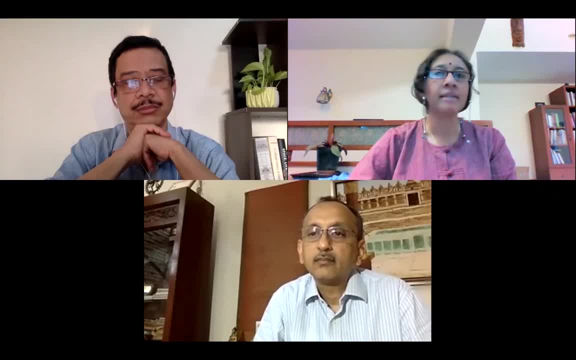 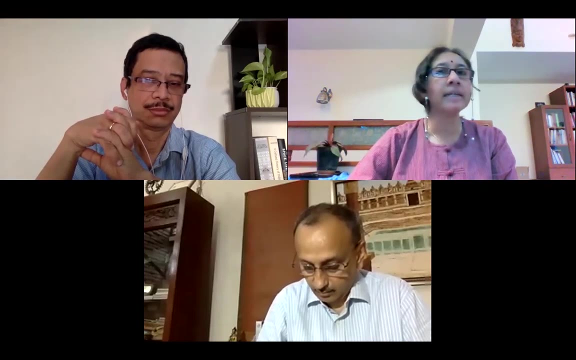 and decide that we are going to do something like this, whether it is at the level of across institutions within India or globally. we do do it And we do achieve some wonderful results, And Hari wrapped up his presentation by talking about some of the characteristics of the scientists. 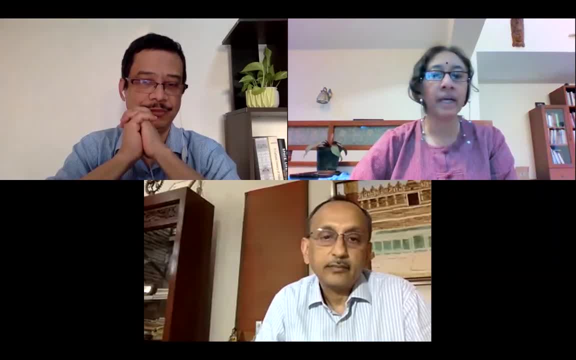 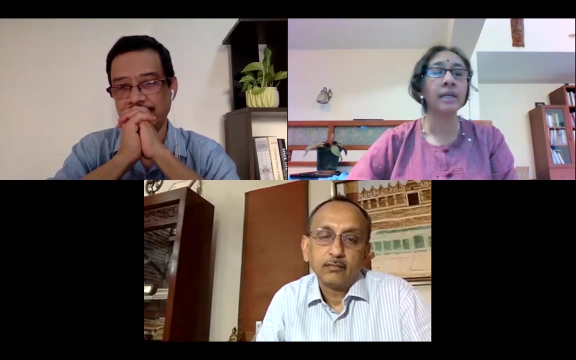 that he has studied for his book, And some of them are the motivation and the sheer determination to see that science would build out in independent India, being able to work in a resource constrained environment, which we will always be like, he pointed out. 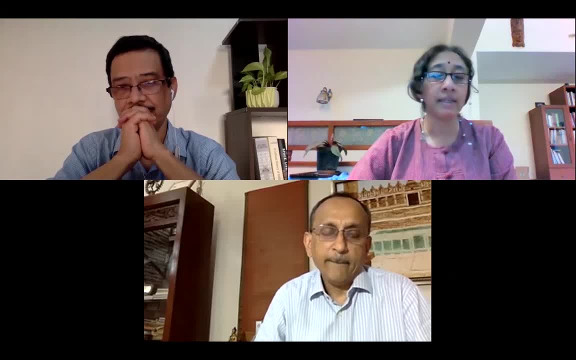 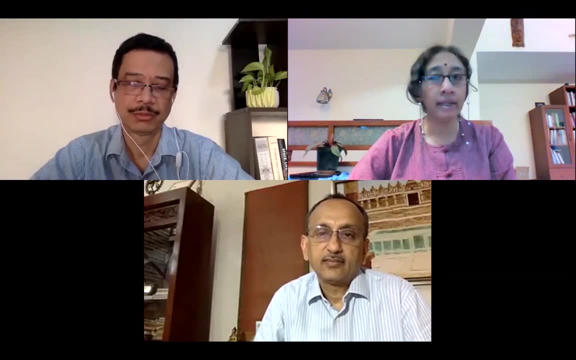 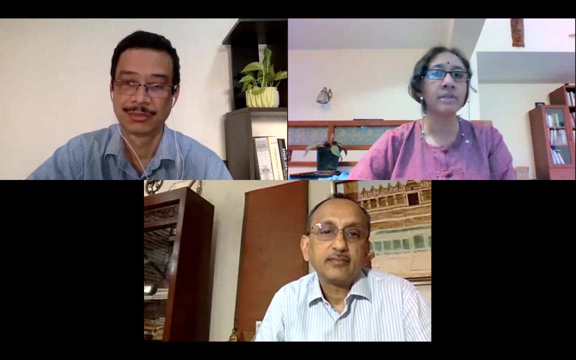 but also the ability to solve, to choose problems that were important to India but solvable, And he also mentioned that, going forward, the focus is less on the solvable and more on the solution. And he also mentioned that the focus is less on the solution. 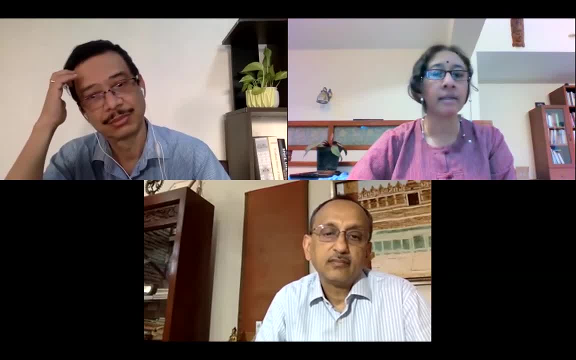 but more on the solution. And he also mentioned that the focus is less on the solvability than on problems that are important and at the cutting edge than on problems that are important and at the cutting edge. And finally, he said that one of the key characteristics- 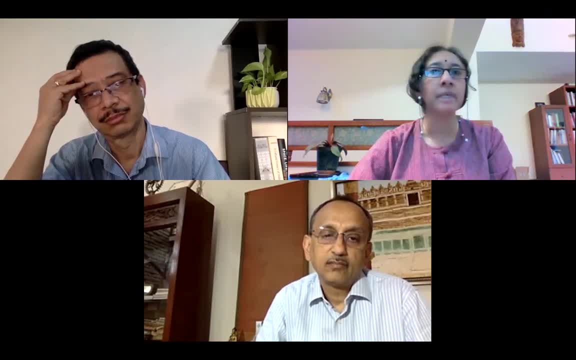 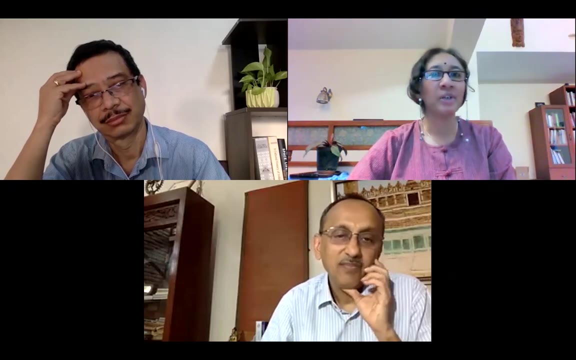 was that they had the ability to convince policy makers about the need to invest in science. And when you talk about a figure like 58 lakhs to build out a telescope in the 60s, that was a huge sum And you know to have been able to convince Dr Baba.